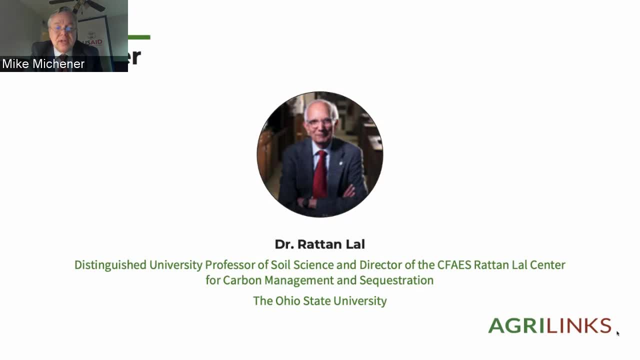 spans five decades and has influenced the future of agrilinks. Dr Lal's work on soil management practices spans five decades and has influenced the future of agrilinks. Careful shew is an originality and a recursive process. He has accusedreme and模bular and 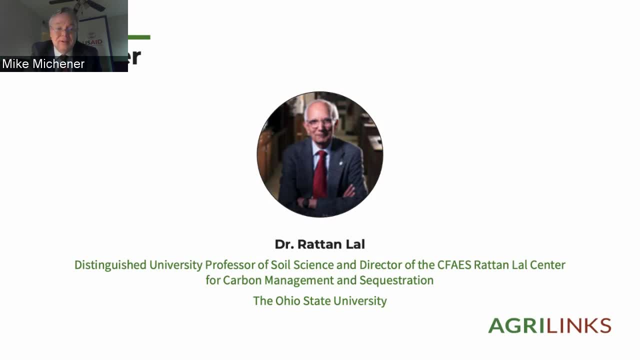 bioanimic practices based on health and wildlife, damage to general areas that are not accessible to the public and rural areas, whileatsächlich invading our historic, natural theirs and bridging the lives of the people and nations. Dr Lal has published over 1,000 peer-reviewed 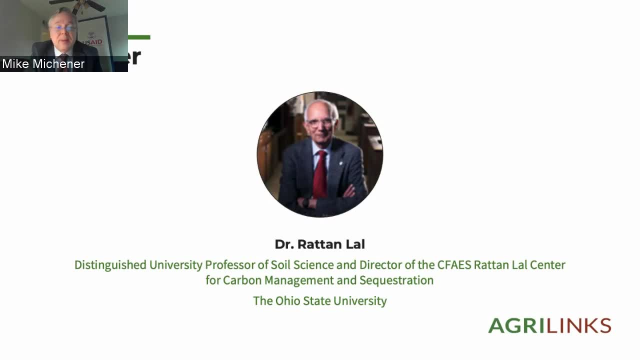 about 400 professionals from around the world, making up a network of scientists addressing global issues related to food and nutritional security, adaptation and mitigation of climate change, and restoration of degraded soils and ecosystems. dr law's work underpins our accomplishments under feed the future and will serve as a key resource as we develop the new. 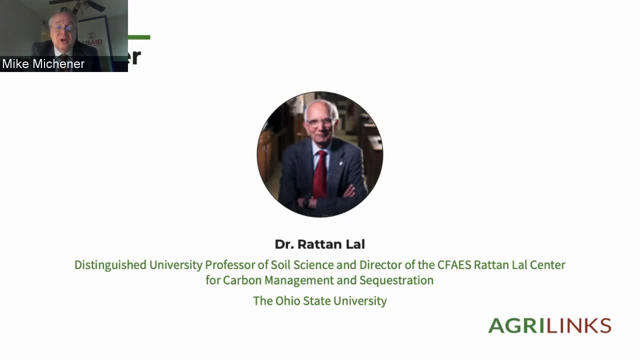 2022 global food security research strategy. we're also looking forward to working with dr law as a new member of the board for international food and agricultural development. with the events unfolding in ukraine, this is a somber and solemn morning, but we can always take a moment to reflect. 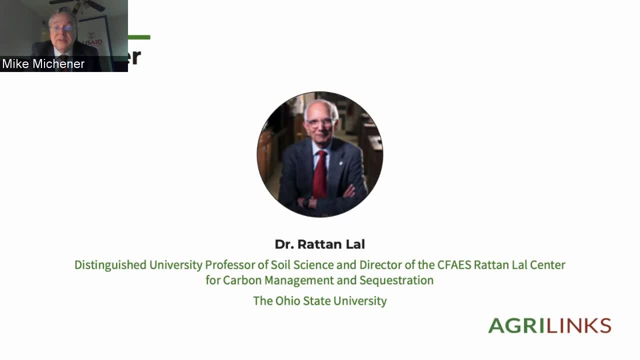 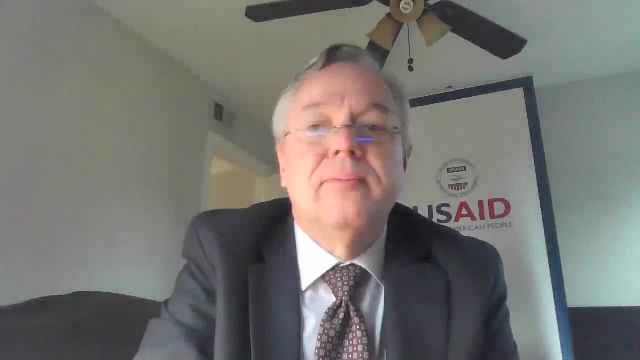 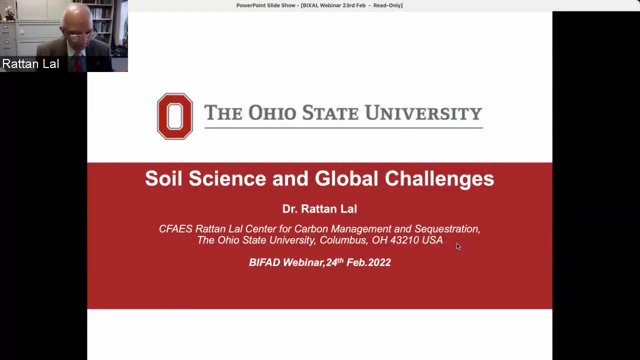 on ways we can all contribute to making the world a better place. i can't think of a more appropriate way to hope for a better future than by spending some time with a visionary like dr law. dr law, we look forward to your remarks over to you. thank you, dr mitchell. i appreciate the opportunity. i also want to thank 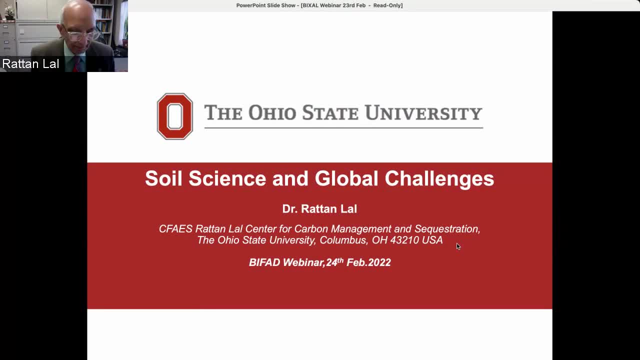 in addition to your kind word of introduction, dr rob burtham, dr jerry glover, gross, clara cohan, many other colleagues, it's a great honor and privilege. i hope you can see my screen slides and you can also hear me. well, the topic i want to discuss with you today is 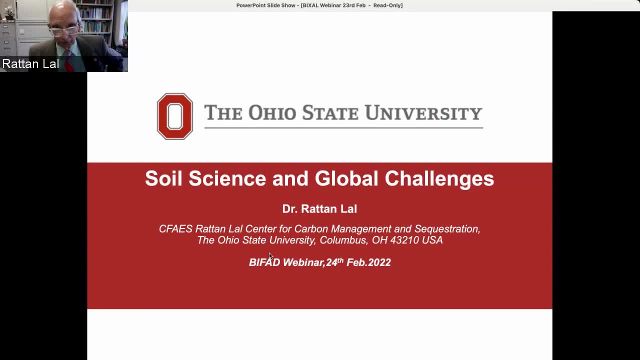 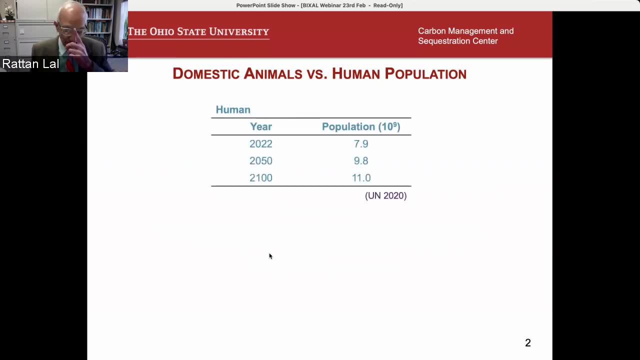 about food and natural resources and the importance of food and natural resources and the importance of food and natural resources and the importance of food and natural resources, today's soil, science and global challenges. i want to begin with the population. human population at present in 2022 is estimated at 7.9 billion, by 2050 9.8 billion and by 2100. 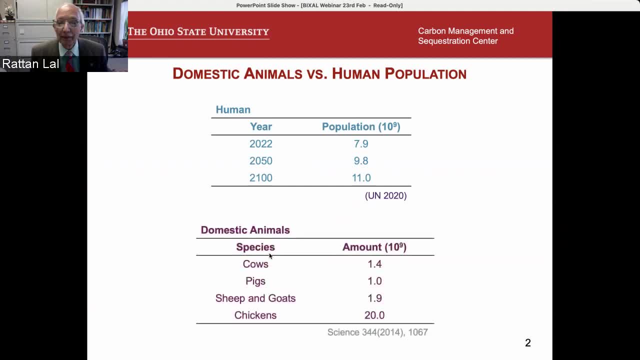 more than 11 billion. in addition to human, we also have domesticated livestock cows, estimated at 1.4 billion, pigs, 1 billion sheep and goat, almost 2 billion chicken, 20 billion. these human and animals require resources. it is estimated that humans are already using. 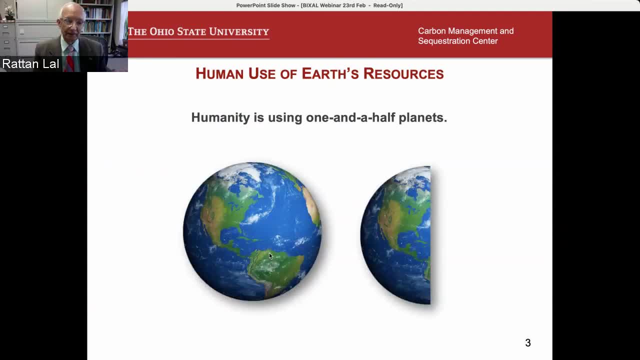 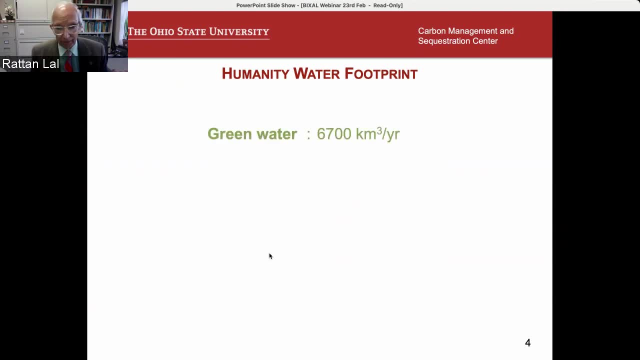 equivalent to one half of the planet. in terms of the resources appropriated by humanity. for example, the water footprint: green water: 6700 kilometer cube. blue water: 1000 to 1700 kilometer cube per year. gray water: 1400 kilometer cube per year. in terms of the sustainability, 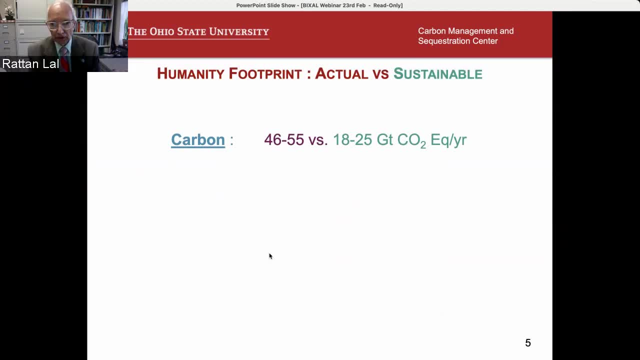 the carbon used by human: 46 to 55 giga ton of co2 per year. the sustainable value should be 18 to 20- 25 giga ton of carbon per year. ecological footprint: 18.2 billion hectare equivalent: it should not be more than 12 billion hectare. material supplies: 70 giga ton per year. it should. 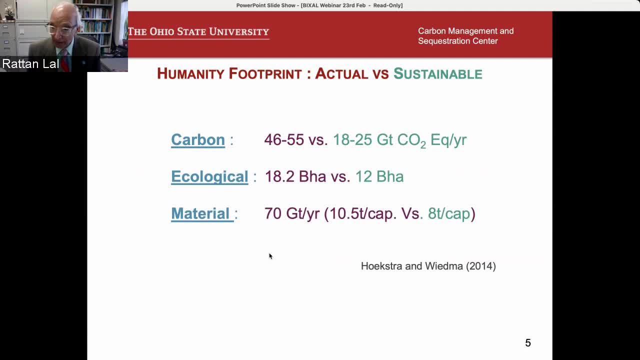 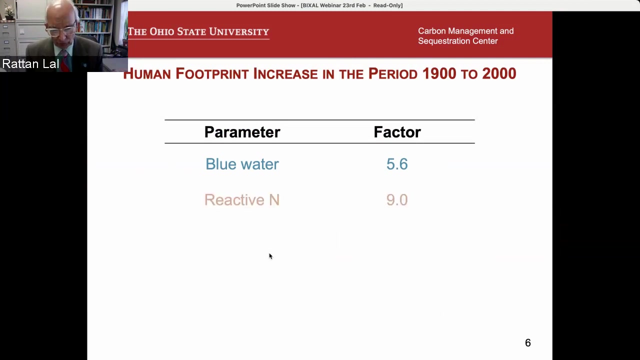 be somewhere about 10.5 ton per capita, which means about 8 giga ton or 8.5 or so ton per capita, rather than 10.5 per capita. human footprint blue water has increased for the last century, from 1900 to 2000, by a factor of almost six reactive nitrogen that 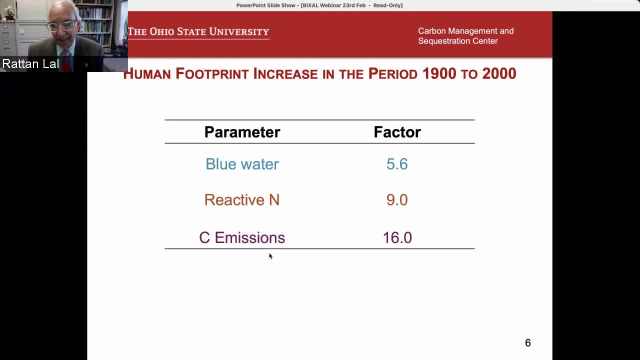 the fertilizer nitrogen by a factor of nine and carbon emission over the last century by a factor of 16.. is there for time to think and revisit our strategy? how to be environment friendly, how to make agriculture and a lifestyle environmental congenial, protective, restorative and friendly, of course? 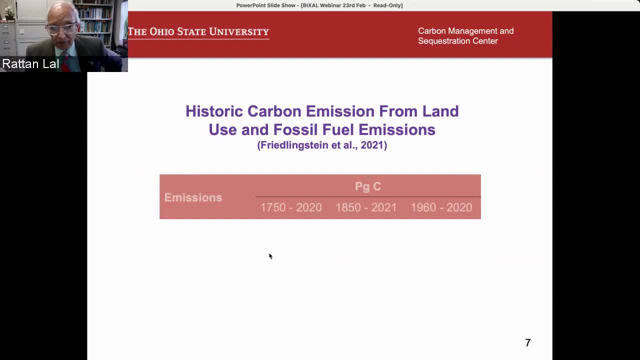 now let's start by the carbon emission. historic carbon emission in land use change from 1750 to 2020 is about 235 giga ton. over the same period, the fossil fuel emission are 460 gigaton from 1750 industrial revolution to 2020. total emission from land use. 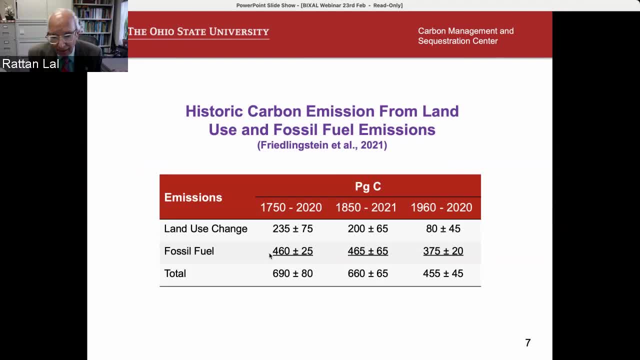 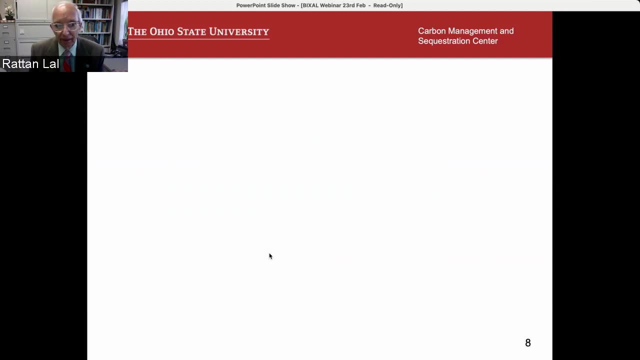 and fossil fuel to date, 690, out of which one third is absorbed by land, half of it by the atmosphere and the remaining by the ocean. so land has been a sink even under natural condition, as human intervention has not particularly tried to recognize the importance of the land-based sink. 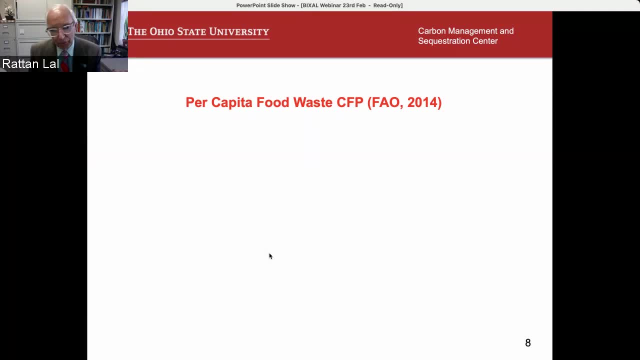 another source of emission which is not commonly mentioned is the humanities food waste. per capita, kilogram of carbon dioxide emitted per person per year by food waste alone: north america: 860 kilogram. industrialized asia: 800 kilogram. europe: about 700. latin america: 500. north africa about 350. south and southeast asia: about 350. 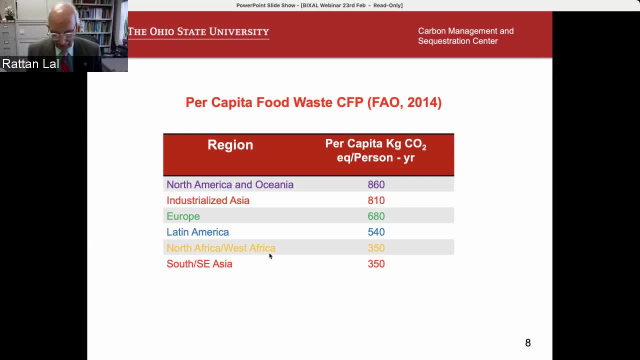 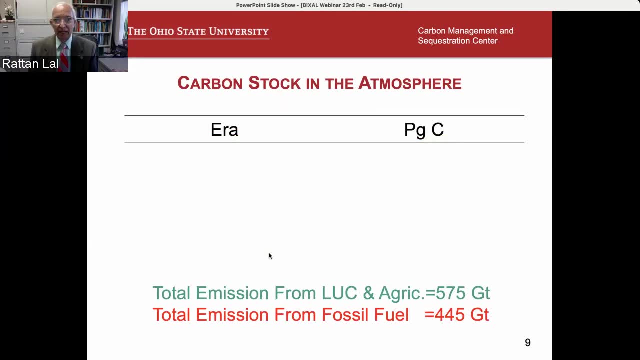 each one of us is culprit and victim in more than one scenarios. think we need to think what can be done to the atmospheric carbon stock which is influencing the climate change. let's take a look at the total carbon stock in the atmosphere. i'm not talking about the co2 in parts per million. i'm talking about the total carbon stock in gigaton. 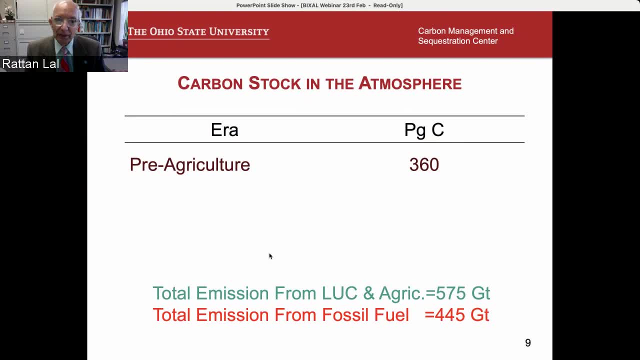 petagram is gigaton billion tons. pre-agriculture: 10 000 years ago it was 360 gigaton. pre-industrial era it was 560 gigaton by 1750.. so by the time agriculture began 8 000 bc and by the time 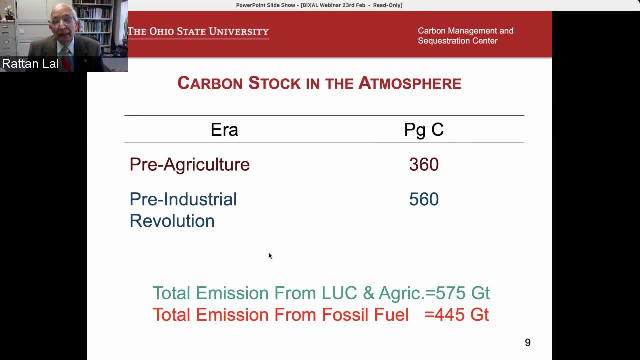 industrial revolution started in 1750, we had already added 200 gigaton. that primarily mostly came from land use conversion for agriculture. since 1750 till now, the carbon stock in the atmosphere is 880 gigaton per year. that's, the total carbon stock in the atmosphere is 880. 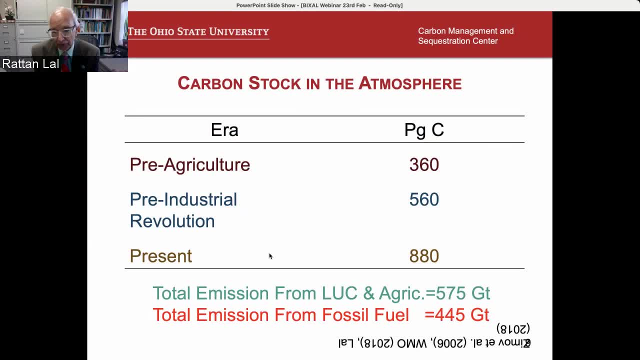 ton, that 320 since 1750 has come both from fossil fuel and land use curve. total emission from land use conversion, if you take 320 gigaton until 1750 and 255, which i showed you in 1750, is about 575 gigaton. total emission from fossil fuel is 445 gigaton. therefore, with 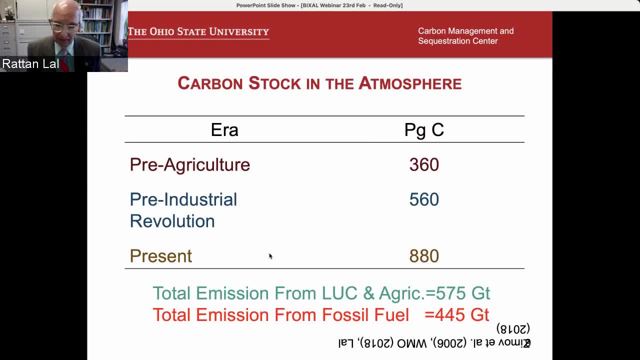 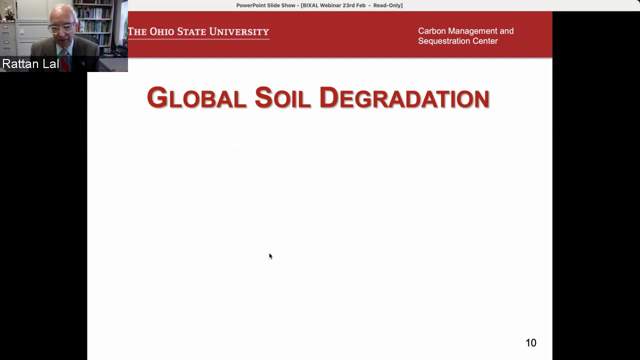 some change in land use pattern, from restoration of degraded land, better use of land, bridging the yield gap, returning some land back to nature. we can, should, must put some of that 575 gigaton back into the nature, into the land, soil and vegetation. so our degradation already mentioned. 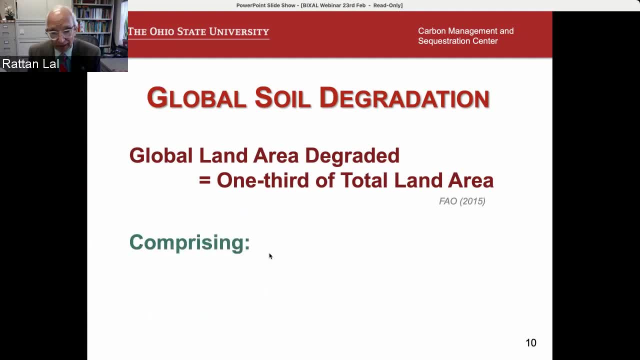 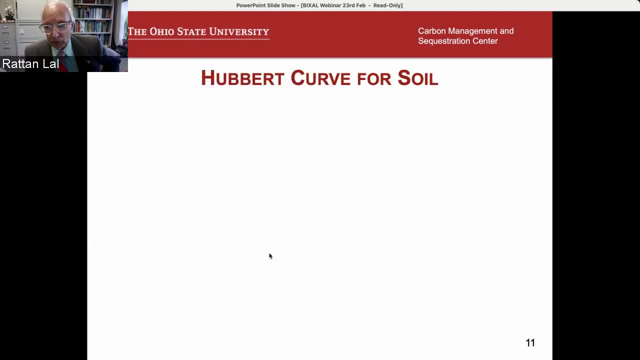 one-third of the total land area. and Lastly, i now would like to move on. young people, if you don't mind, then change hands again from increase. İ answer you. the first idea asked is: the third area will also salt 이�nu had indicated, not just, whereas in this case the third area, which have we also mentioned? 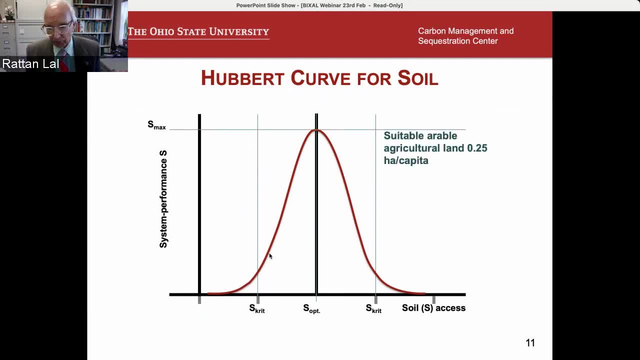 but as as a potato areation we introduced as times change in the location of the earth, as can we break up a new temperature around this plate. we change the changes incé and in we, then we develop it and then the environment we have. so you put as major portion each pointket. 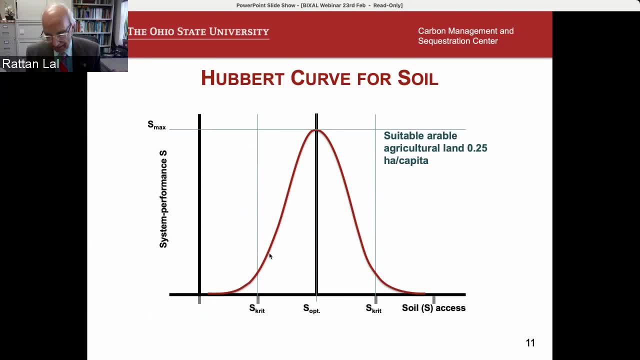 or any of these facilities as we. your investment for five- mocadow- that's why none of them is living- is about quarter of a hectare. in many densely populated country, the per capita land area is already 0.05 hectare. china is very close to it, bangladesh is close to it, and this has 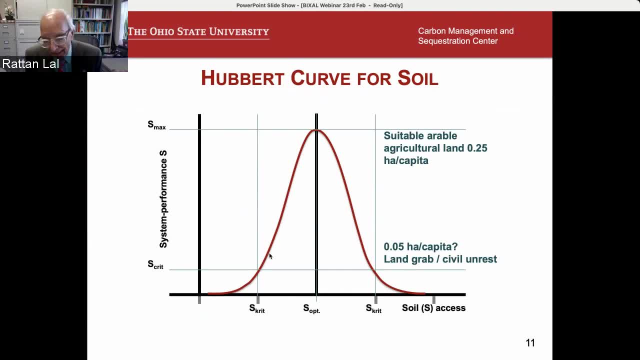 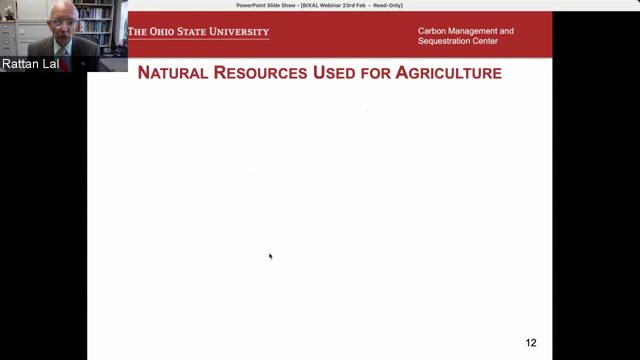 promoted this serious problem: land grab- you understand what that means- and soil refugees, climate refugees. so indeed, there's a peak soil, there is a undangered soil. we do have extinct soil. it's not only plants and animal that are endangered and peak and extinct, we also have the soil the same way. so if you look at the natural resources used for agriculture, 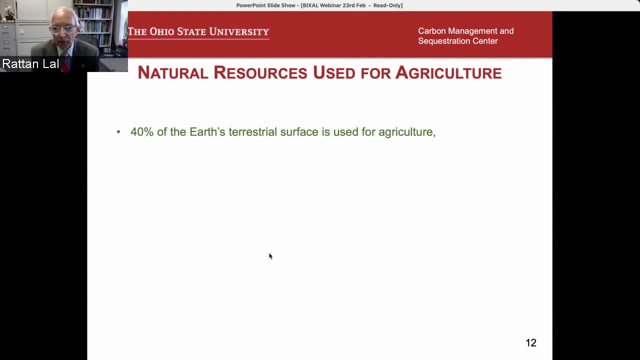 40 percent of earth's trential surface is used for raising plants and animals. 75 percent of agriculture land- estimated about 3.75 billion hectares- is allocated raising animals. Another 1.5 billion hectares to raising crops total 5 billion hectares. 70% of global fresh water withdraw. 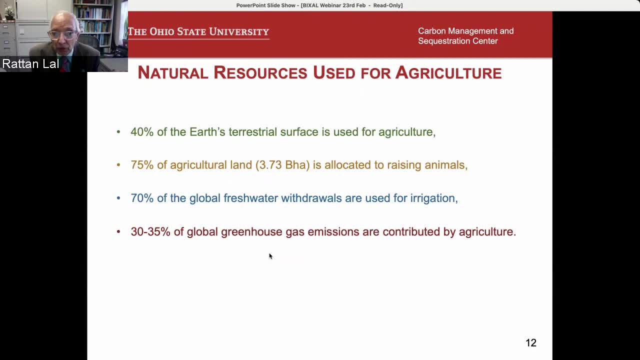 are used for irrigation. 30 to 35% of all greenhouse gas emissions come from the world food systems, All aspects of agriculture, plus food processing, packaging, transport management, everything food supply chain. 30 to 35%, and yet 820 million people. 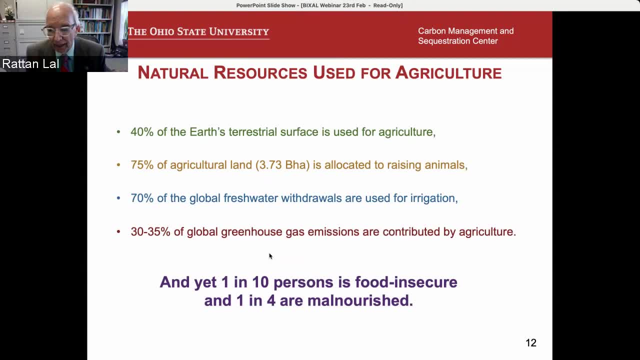 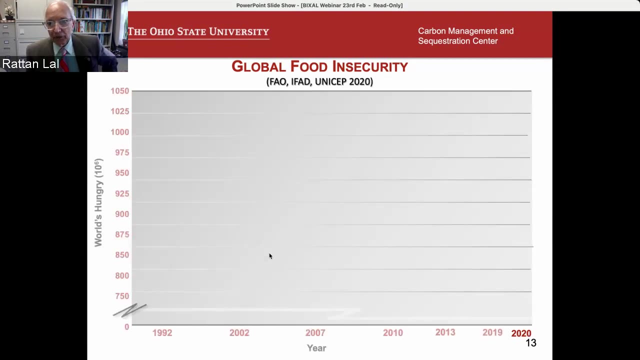 1 in 10 are food insecure and 1 in 4 are malnourished. Therefore, business as usual is obviously not an option. It's not sustainable. The food security issue really had to be looked at from the point of view of. 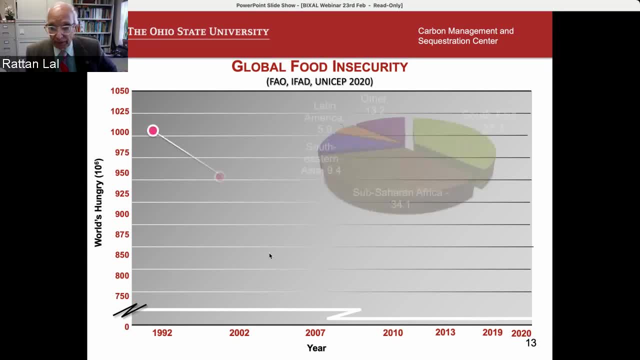 global sustainable development goals. We made good progress. In 1990s, almost a billion people- more than billion- were insecure food. We kept on decreasing the number to less than 700 million- 690 to be exact, in December 2019.. In December 2020,. 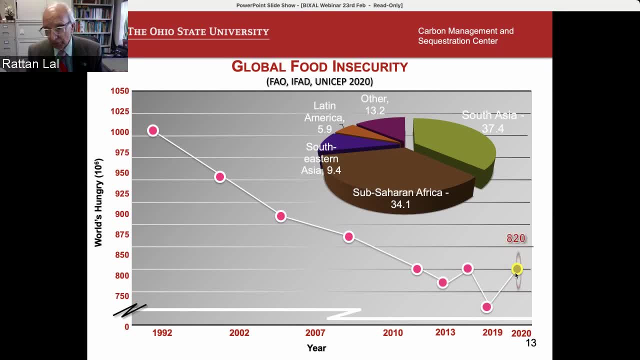 because of II. the number of insecure people is around 820 million people living in South duck has almost 37%. Sub-Saharan Africa, with face lake wildfire Swedish to 13% Vнд, ablCanada- about an hundred thousand. like America, Most in the US. I, South Asian and sub-saharan Africa account for most of the world's. 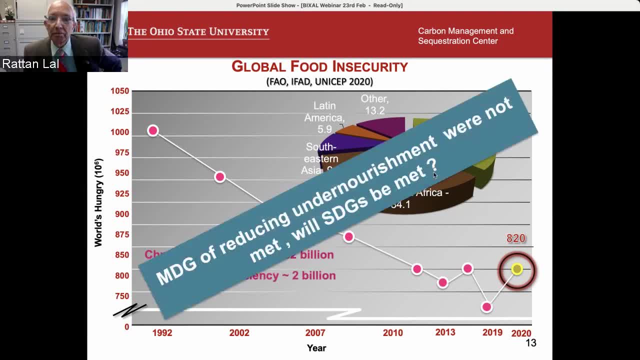 26 million and 30% are others. South Asia and sub-Saharan African account for most of the world's hundreds hungry people. This part just as millennium development goal. unfortunately, sustainable development goal as of today are not on track And we still have eight years. We can do something. 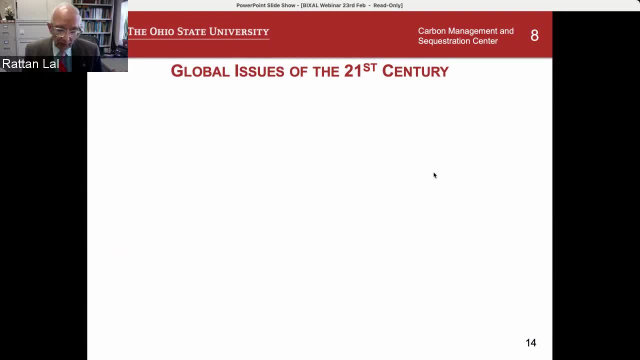 even now. Therefore, after what I presented to you, what the state of the planet Earth? we have at least 10 issues of global significance. Population: 7.9 billion, increasing at the rate of 1.1% per year. That is, 7.25 million per month Per capita. arable land area already. 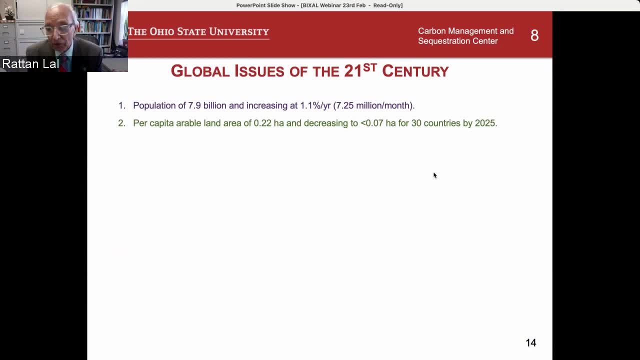 0.22 hectare and decreasing to 0.07 hectare in 30 countries by 2025.. So I'd like to say this is a clear result: Renewable fresh water supply, less than 1,000 cubic metre per people in 30 countries. And. 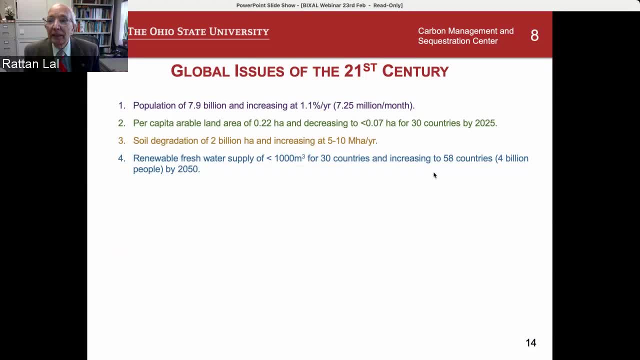 those countries number, with water scarcity increasing to 58.. 4 billion people affected by 2050.. Atmospheric concentration, as of yesterday, 222.. was 412.5 parts per million and increasing at the rate of more than two parts per million per year. 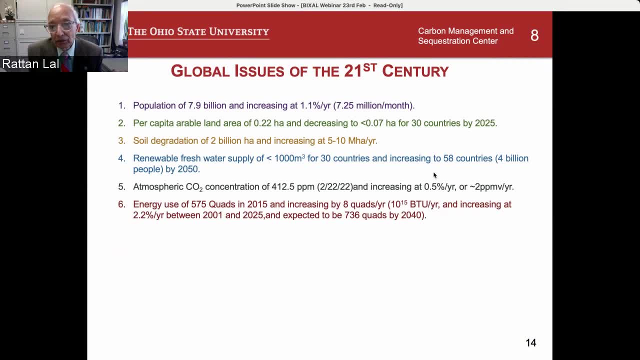 Energy use: currently 575 quads, that is, 10 to the 15 BTU and increasing 2.2 percent per year. The number will be 736 quads by 2040.. Per capita grain consumption: 300 kilogram. unfortunately in some countries decreasing and food insecure. population: 820 million and increasing especially. 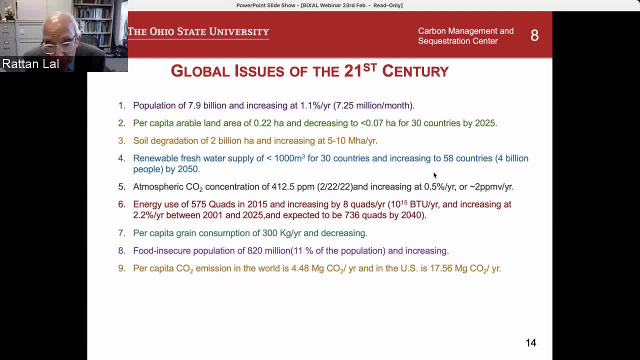 because CO2 emission per person, globally put, 4.5 metric ton of CO2. you can see that CO2 emission per person globally 4.5 metric ton of CO2. you can see that US somewhere between 15 and 17.. Humanity's per capita water footprint 1385 cubic meter per year. 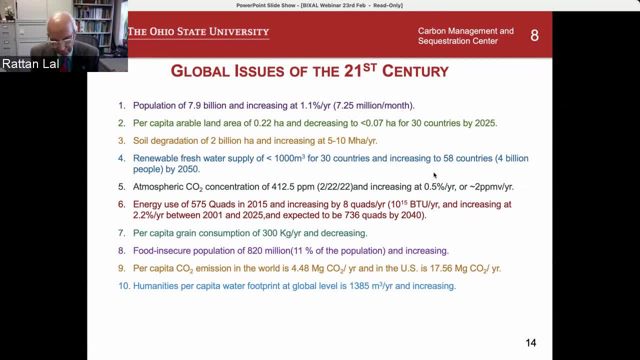 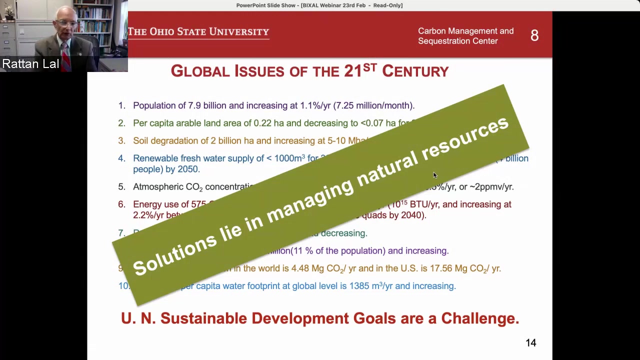 per person and increasing. This state of affair cannot continue. It must not continue for the sake of humanity and, of course, for the sake of the planet earth. UN sustainable development goals are now being challenged. UN sustainable development goals are now being challenged. Solution to this issue really lies in sustainable management of natural resources. 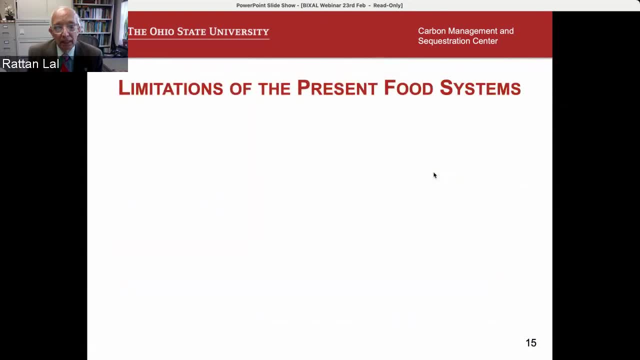 especially the soil, soil of the world. That brings me to the question of the food system. The food system summit started for two years, ended on 23rd of September The final report by the secretary general, and this has failed to end hunger and nutrition. The food system at present have failed to end hunger and malnutrition. 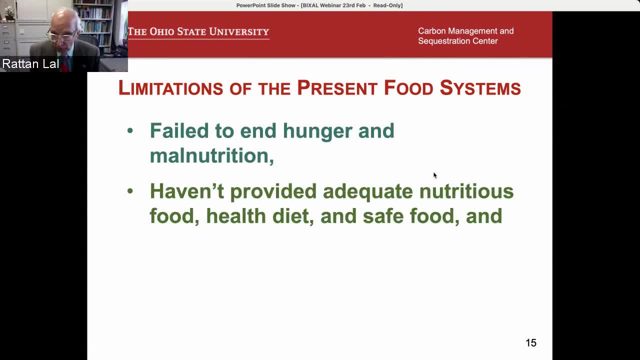 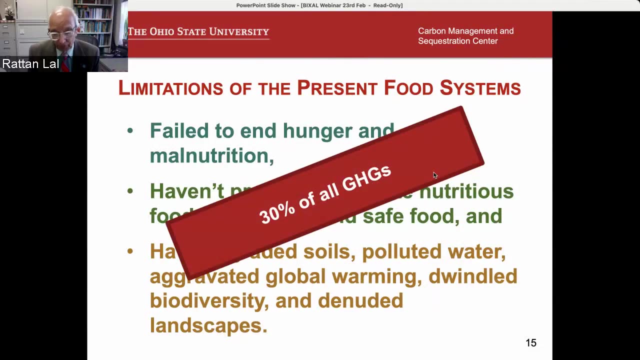 They have not provided adequate nutritious food, healthy diet and safe food, and they have degraded soils, polluted water, aggravated global warming, dwindled biodiversity and the nudity landscape. 30 percent of all greenhouse gases come from food systems. 30 percent of all greenhouse gases come from food systems. 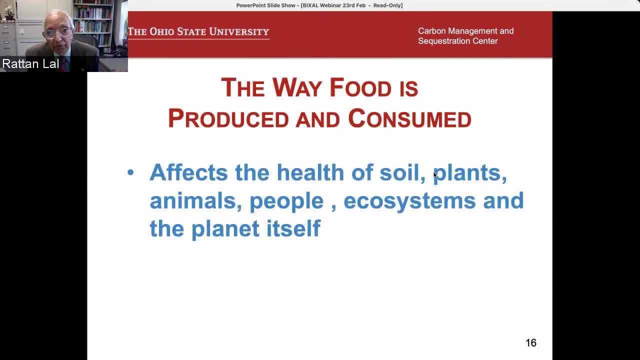 The way food is produced and consumed. it affects the health of soil, plants, animal, people, ecosystem and the planet itself. Above all, the sustainable development goal of the agenda 2030 are not on the track, and food systems have something to do about it. 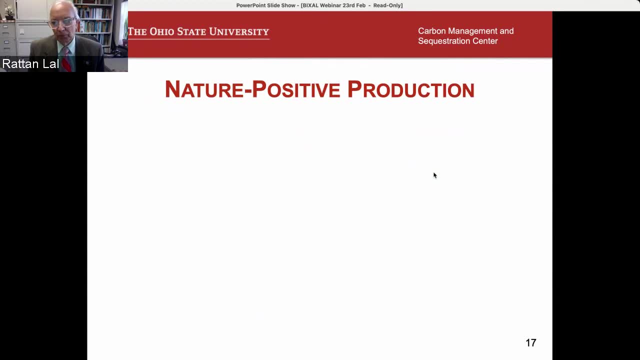 Therefore, we should be thinking about nature positive production, nature friendly production, Agriculture and nature have to be having following synergistic pathway, friendly pathway, cooperative pathway. Agriculture, which we, each one of us, perform three times a day when we eat food, has to be nature positive, has to be nature friendly. There's no other option. 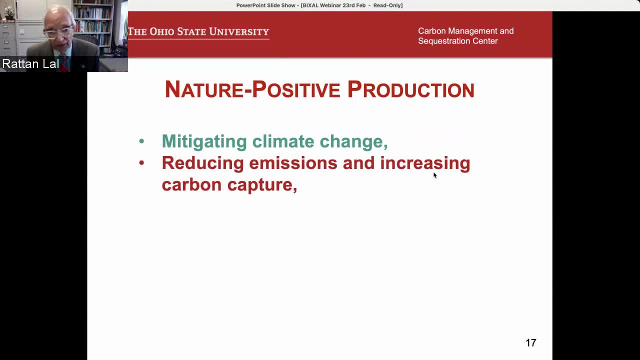 It must mitigate climate change, it must reduce emissions and increase carbon capture. it must regenerate and protect critical ecosystem. It must reduce food waste and energy uses, and we must return half of the agricultural land back to nature sometime by the end of the century or soon thereafter. We cannot keep taking more and more from nature. 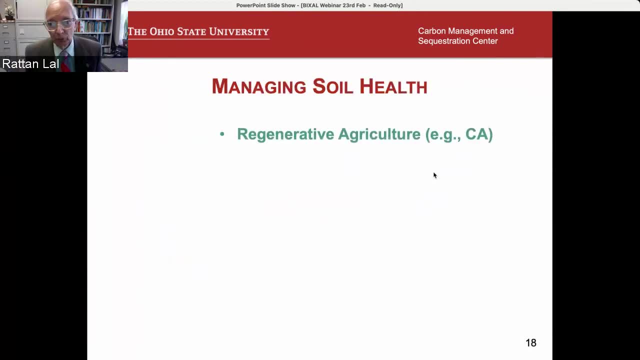 Managing soil health is very critical to regenerative agriculture. digital agriculture, artificial intelligence in agriculture, biofortification of crops to fight hidden hunger, the soil-water-air-energy nexus, interconnectivity- These are not silos, They interact together And of course, we must try to build and synthesize and restore the soil quality and soil health. 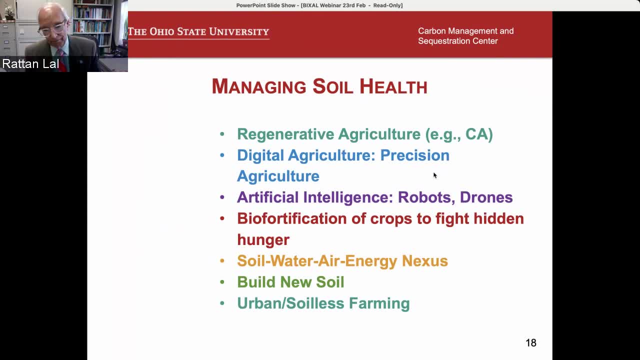 We must think about soil-less farming in an urban ecosystem so that we can return some land back to nature, but, more importantly, take carbon dioxide from the atmosphere, which has taken a lot for the last 10,000 years, back into the land. 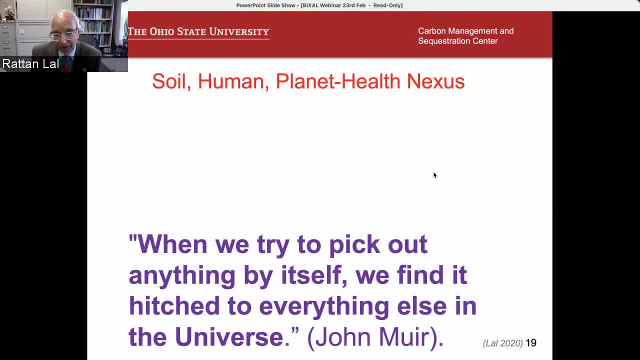 That brings me to the question of the interconnectivity. One health concept, Soil, plants, animals, Human ecosystem and the planet is one and indivisible. This was said in a very different way by John Muir, but the concept is the same. 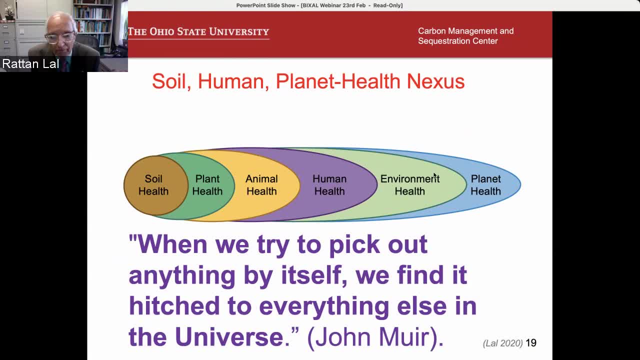 When we try to pick out anything by itself, we find it hitched to everything else in the universe And this interconnectivity should not be forgotten. I know because of COVID-19, we have given a lot more emphasis to human health. 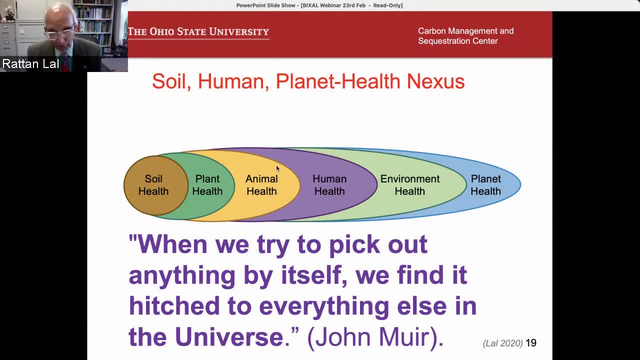 We have given a lot more emphasis to human and animal health, which is true, should not be undermined, But the fact remains: human health is strongly impacted by the health of soil. True soil impact on plant, animal environment and the planet. 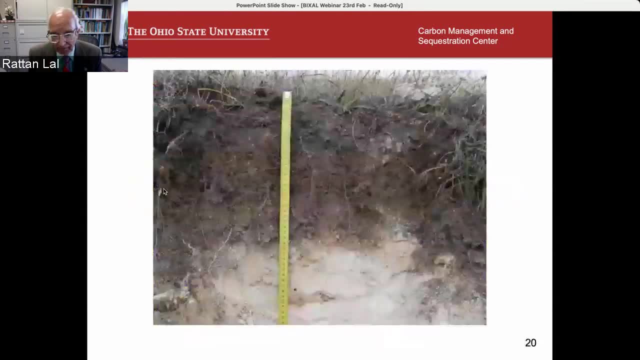 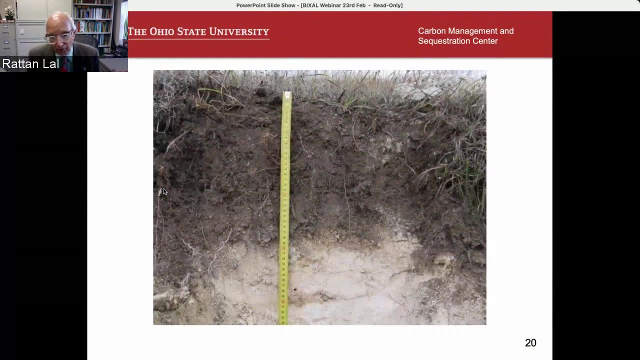 That is the philosophy, that is the concept that we should not forget. Now, coming back to soil quality, If you look at a soil profile, you normally see the topsoil rich in nitrogen. Underneath, in many soils, especially the dry region, you have inorganic carbon. 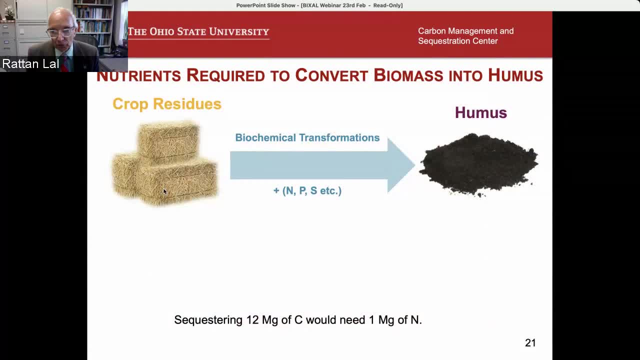 And we have both of these carbon, which are important. Question is: how do you increase the depleted carbon stock in the soil? Soils of agro-ecosystems, especially those of resource-poor small farmers, is depleted to as much as 75 to 80% of what it originally was. 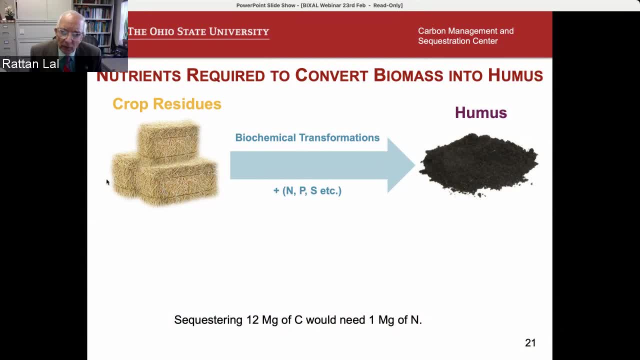 And the only way we can restore is by adding organic matter- biomass carbon- into that soil. So here is a biomass carbon. somehow it got to become a humus. This biochemical transformation requires input of additional plant nutrients: Nitrogen, phosphorus, sulphur. 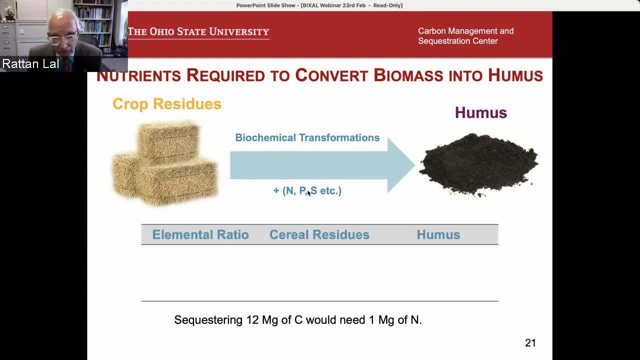 At least these. Why? Because the carbon to nitrogen ratio in the residue in the wheat straw- corn straw- is about 100, 120.. In the humus it's about 10 to 15.. Carbon to phosphorus ratio in the straw is about 200.. 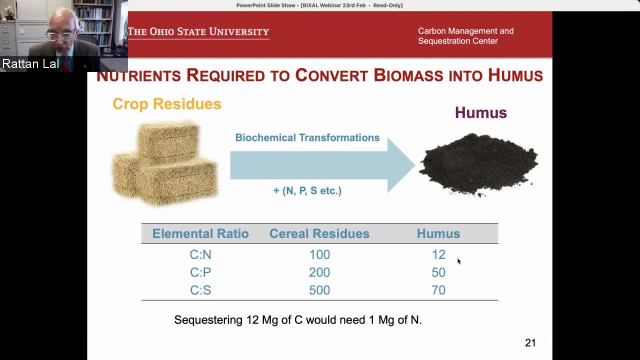 In the humus it's about 50.. Carbon to sulphur ratio in the straw is 500.. In the humus it's about 70.. So humus is enriched of nutrients. Therefore, for the organic carbon to be replaced, 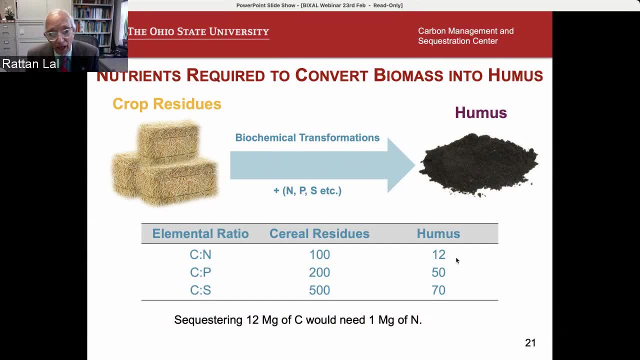 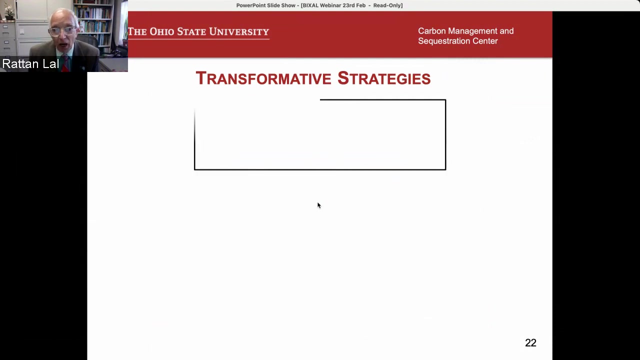 in the soil that we have depleted. not only have the farmer to put the residue back, but this residue also has to be supplemented by additional nutrients. Therefore, farmer has to be compensated for all those additional input. This is very critical. And that brings us to how. 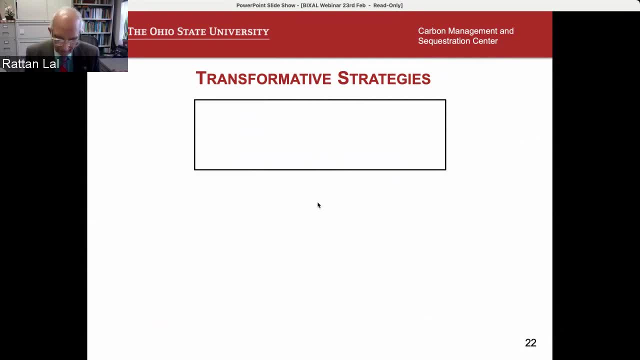 How this transformation will happen. The current business as usual, as we have discussed it, is characterized by 5D: Humanities have depleted, degraded, destroyed, discarded and dominated nature. In addition, we should think about how to reduce our needs so that we can share some of those resources. 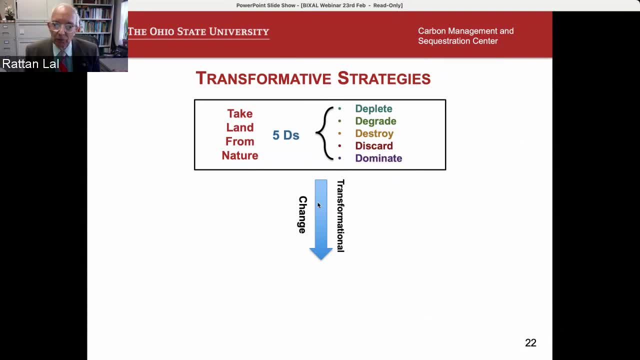 with another habitat of the planet, the biodiversity, And therefore that transformation is with 5R. And what are the R's? Reduce, reuse, recycle, regenerate and restore So that some of the land can be returned back to nature. 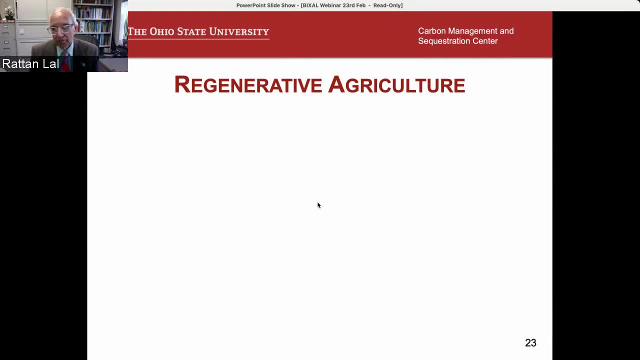 That's the philosophy, That's the concept that we want to talk about And these days, including the Food Systems Summit, talk about regenerative agriculture. We have 300,000 types of known soil series. To assume that there is one type of regenerative agriculture? 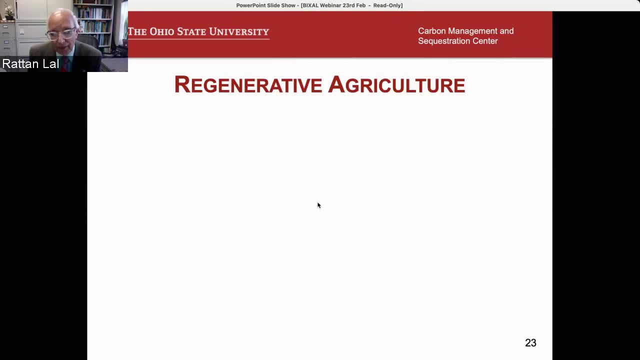 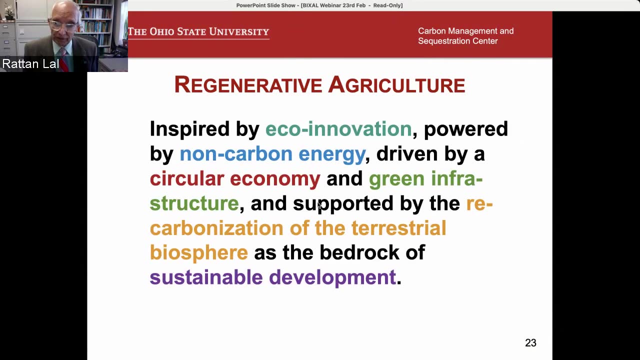 applicable universally is rather being naive. But there is one concept: the principle. The principle is the one which is inspired by eco-innovation. It's powered by known carbon energy, Known carbon energy. It's driven by a circular economy and green infrastructure. 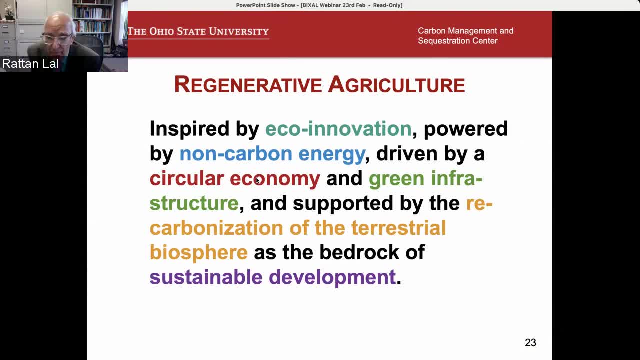 But it must be supported by the re-carbonization of the terrestrial biosphere at the bedrock of sustainable development. So any practice that will re-carbonize the terrestrial biosphere, based on intensive ecological intensification, based on known carbon energy and driven by a circular economy. 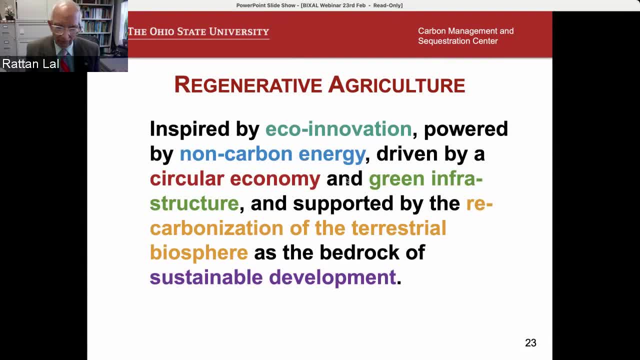 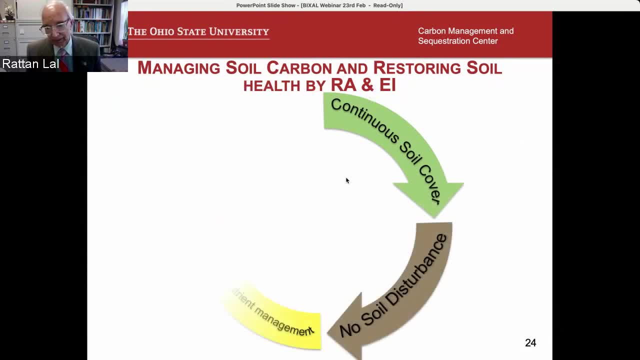 it does not mean no input. I want to come back to that in a moment. No input is not what we are talking about And this concept is based on continuous soil cover, soil never left bare, no soil disturbance, integrated nutrient and pest management. 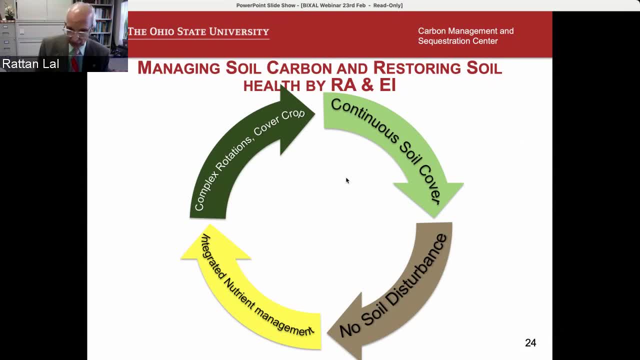 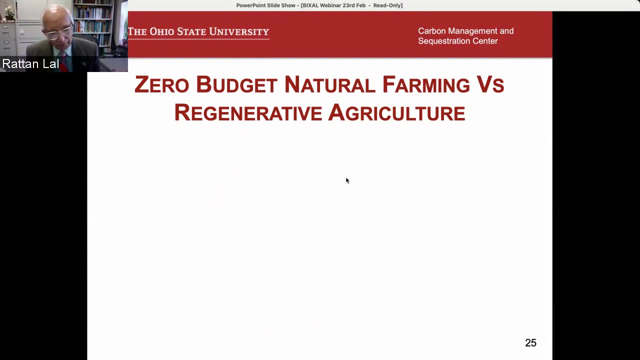 Remember integrated, It does not say zero. this Integrated Complex rotation and cover crop so that we can produce more from less. More from less, Less means judicious use, Reduce waste. Many people talk about zero budget, natural farming, And I want to make sure that's different. 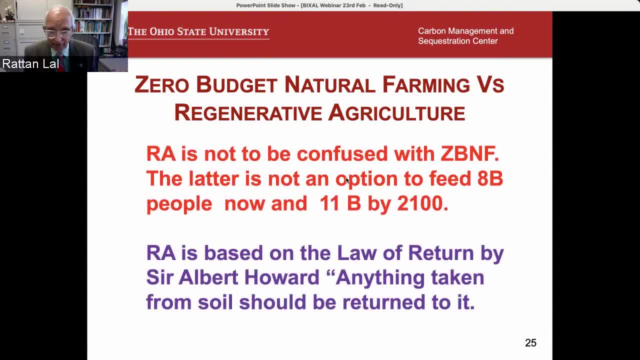 than the regenerative agriculture. Regenerative agriculture is not to be confused with zero budget natural farming. The latter, sometime, is not an option to feed 8 billion or 11 billion people by 2100.. Regenerative agriculture is based on the law of return. 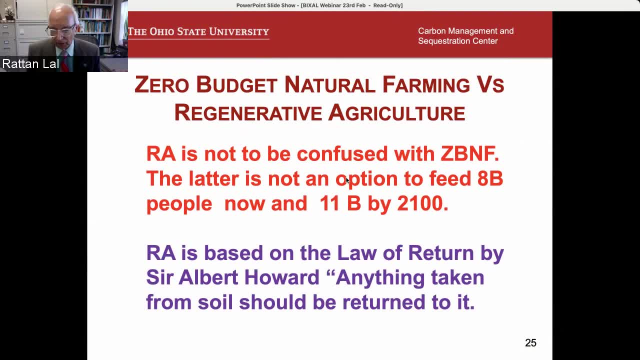 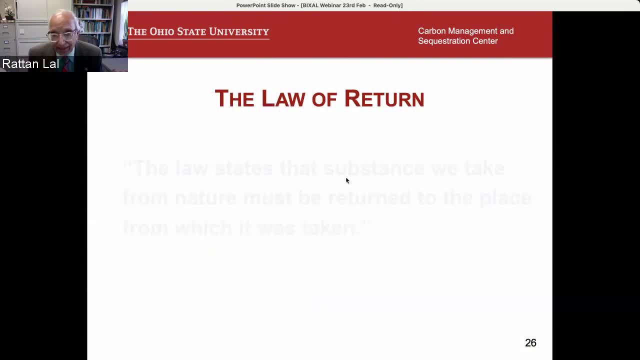 Law of return, Very well explained by Sir Edward Howard, That anything taken from soil must be returned to it. And that is what it is. The law states that substances we take from nature must be returned to the place taken From the same place. 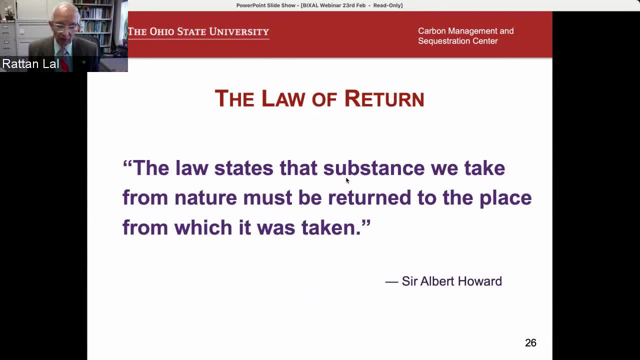 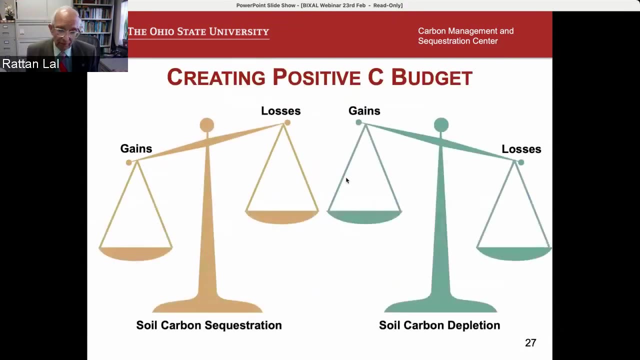 One way or the other, And that is what it means. If you want to harvest productivity grains, livestock, anything produced, whatever is taken one way or the other, has to be returned back to Because we have taken too much already. 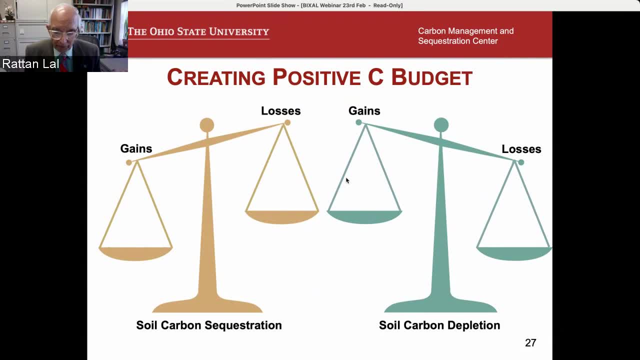 Therefore, what we put back into the soil has to be more than what we take out of soil, And there are many ways we can put things back in the soil. But to take away carbon from soil by erosion, leaching, decomposition- those are the most common processes. 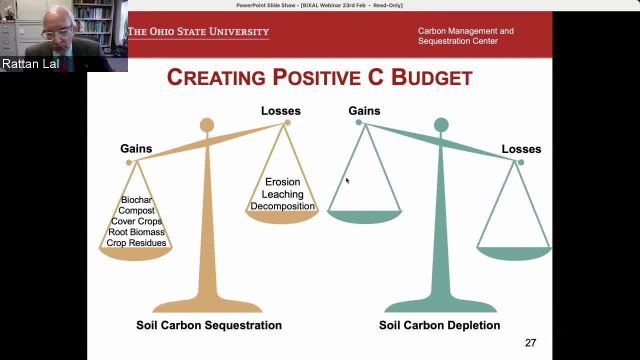 Harvesting sometime. root crops can also take away soil and carbon, But whatever we put in the soil must always exceed what we are taking out. Unfortunately, throughout the developing world and everywhere else, most of the time what we put in is much less than what we take out. 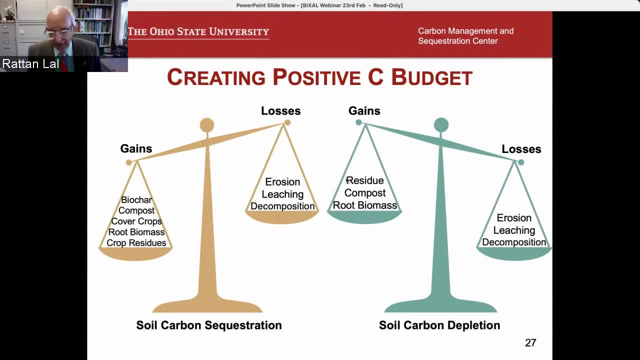 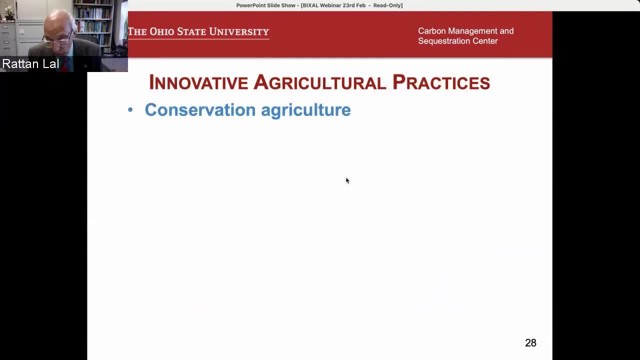 Therefore, soils are continuously being depleted, And that depletion process is what we call degradation. It has to stop. What we do is to make a lot of excess of these soils. There are many issues in our agriculture right now. In fact, we have lots of issues. 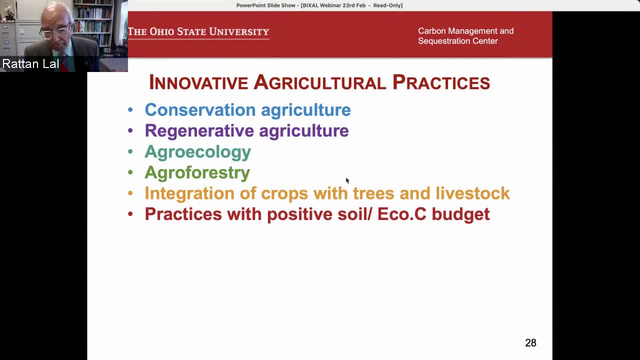 that we must take care of, And they are a lot of holidays. We need to try and take them out, And that's why we are doing so many things, So we should try to do as much as we can to get rid of the problem. 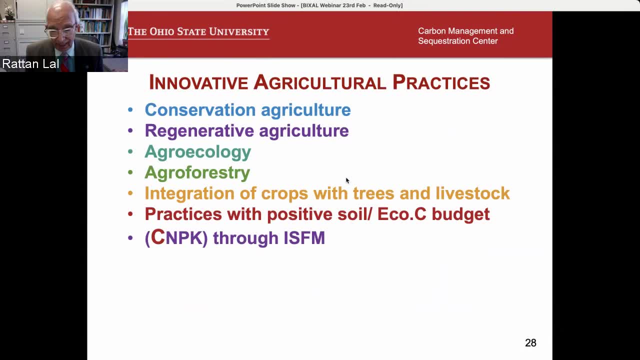 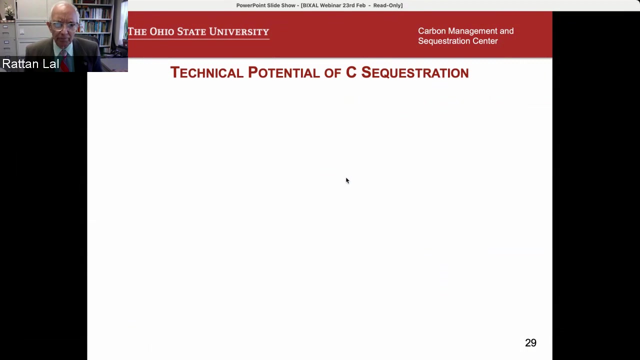 Let's try, becomes less. and the CNPK concept is: integrated soil fertility management, balanced use of N with PKS and other macronutrients, drip fertigation to replace flood irrigation, and digital agriculture, precision farming, artificial intelligence, many other options. if we did that and consider about the positive carbon budget, the technical potential carbon, 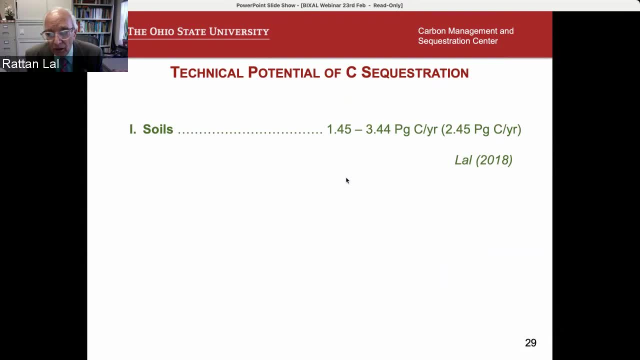 sequestration soil of the world is about two to two and a half gigaton of carbon per year. remember, annually we are adding carbon into the atmosphere: 10 gigaton through fossil fuel and about one gigaton to land use. out of 11, two and a half can be returned back to soil by improved 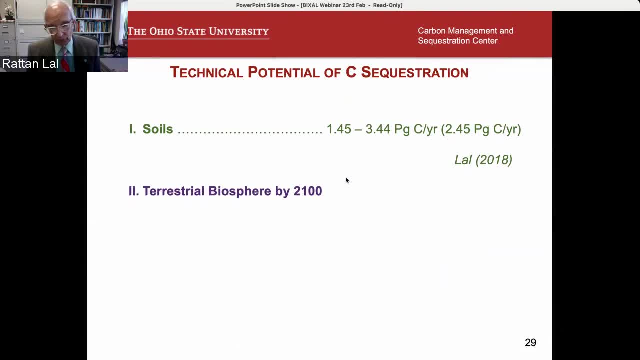 soil management practices between 2020 and 2100. the estimate of how much carbon we can put back in the soil is about 180 gigaton. in vegetation we can put another 150- 160 gigaton, total about 333 gigaton, which can create a drawdown of atmospheric co2 about 157 part per million. 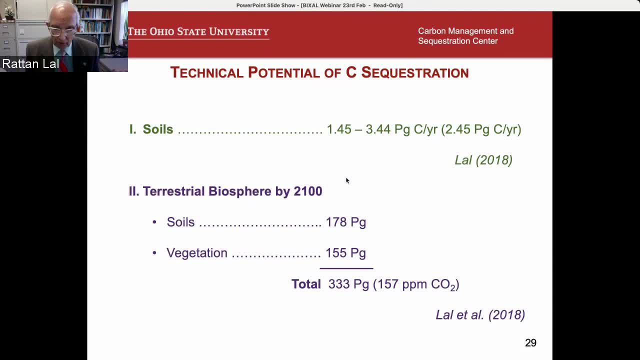 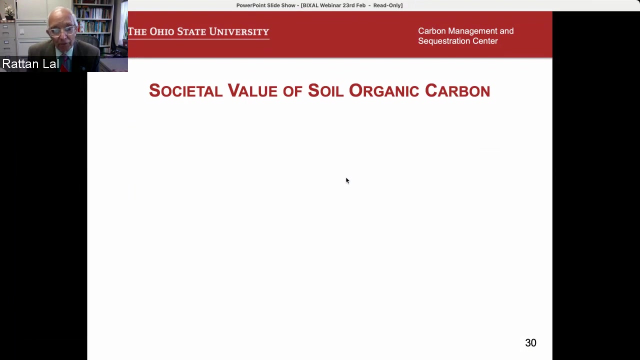 therefore, if we find non-carbon fuel sources soon- solar energy, hydro, geo, whatever bio- we do better agriculture, which we just explained. the possibility of limiting global warming to two degrees centigrade is still possible, as long as we take action. and for this action one part is paying. 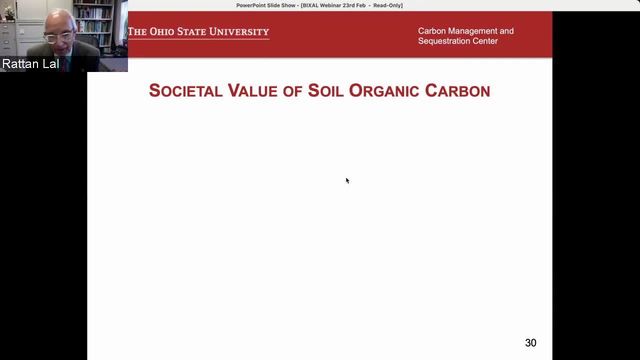 farmer fairly, justly, transparently and sincerely- that payment under 30 dollar per ton of carbon come to 30 to 35 dollar per credit of carbon. so if a farmer sequestered half a ton they should be paid about 60 to 17 dollar per hectare, 25 to 30. 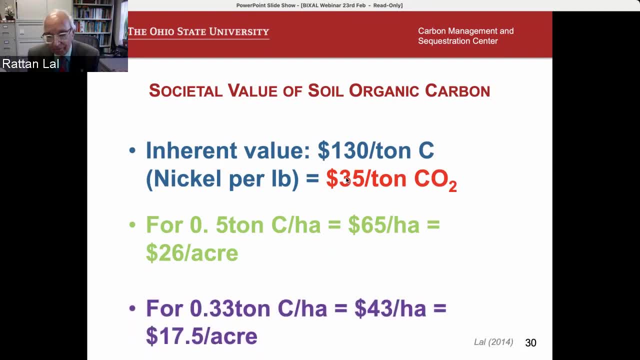 dollar per acre. if they sequester one third of a ton, they should get about 40- 40 dollars per hectare, about 18 to 20 dollar per acre, five dollar per person, per acre or per ton. credit will not do it, but in 2020 the policy will be passed and that's it, and that's what we're talking about. 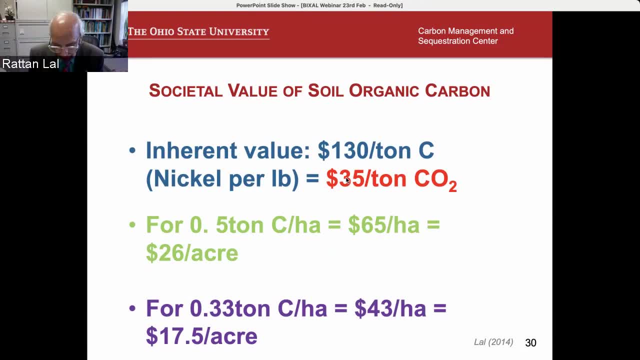 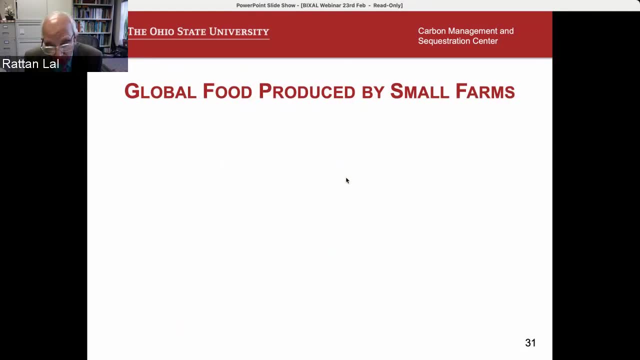 take care of how much carbon is being used and how much carbon you can get from carbon. so we need to do something about this, because a lot of people are working in this kind of business and they are making a lot of money now. and here's the thing. 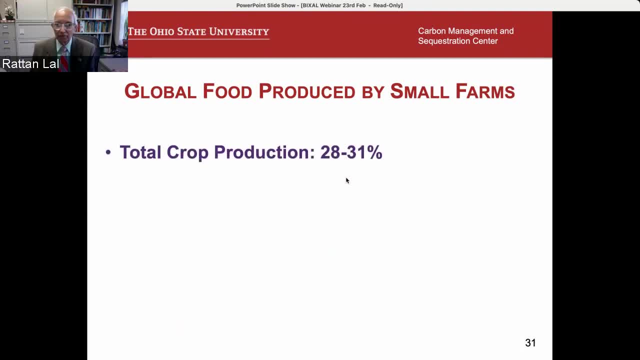 i think that we need to do is to uh collect the carbon that we get by removing the carbon and to make an effort to generate carbon. that is the way that we can bring home. longer is to reduce carbon production by taking carbon out of the soil- at least a single drop. we can do that, but 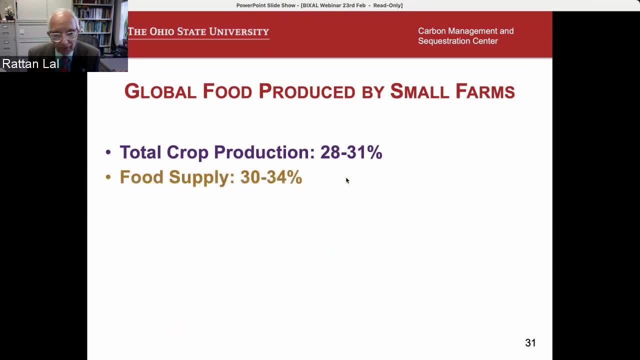 70 million of them globally is about one-third. 30 percent food supply, about 30 to 34 percent gross agricultural area cultivated by them: 24 percent. total number, about 570 to 600 million. their farm size is less than two hectares. we cannot ignore them. we cannot afford to ignore. 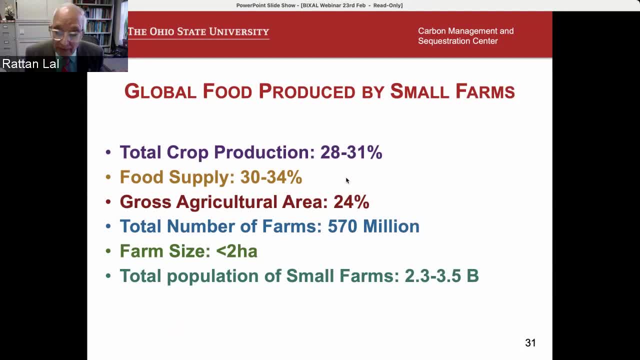 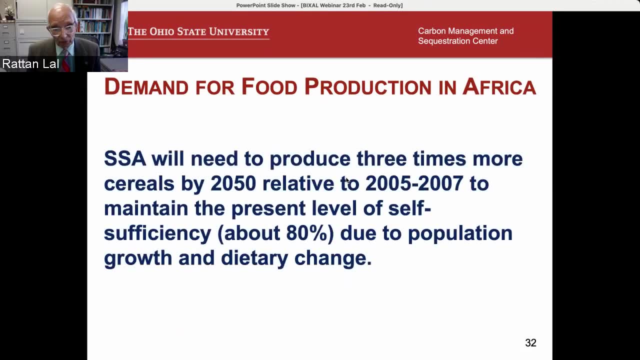 them because 2.3 to 3.5 billion people are fed by small landholder agriculture. they're very important from southern africa. smallholder farmers will need to produce three times more cereal by 2050, relative to 2005-7, to maintain the present level of self-sufficiency. 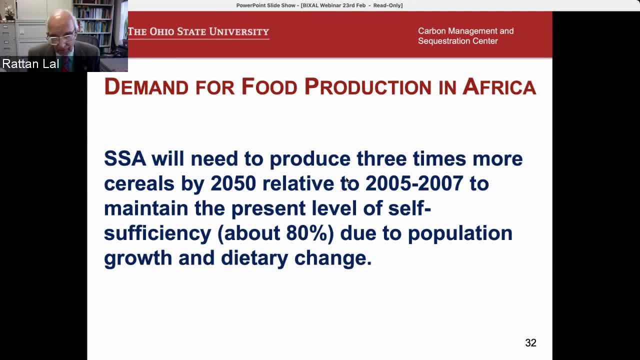 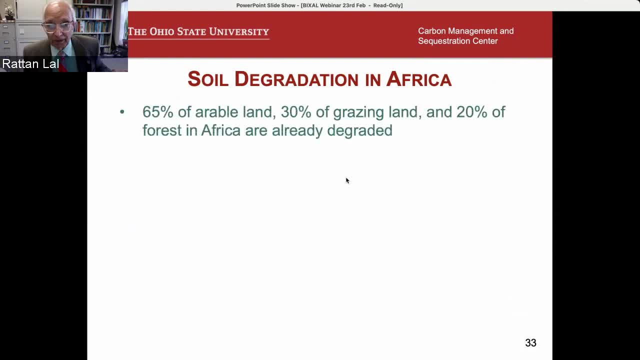 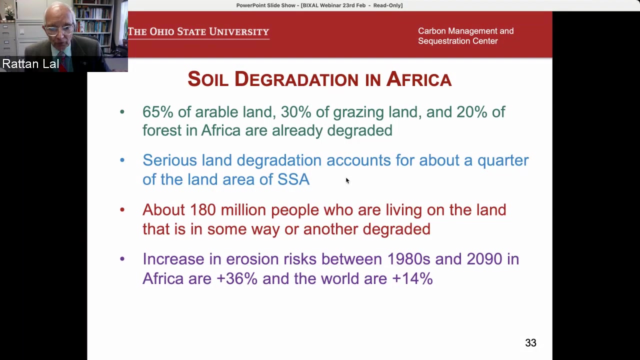 which is only 80 percent. therefore, small farmers there really need major transformation in agriculture, especially because soil degradation in africa- from africa 65 percent of cropland- and serious land degradation accounts for very major problem affecting 180 million people- 200 million dc estimate- which are food insecure and increase risks of soil erosion between now and 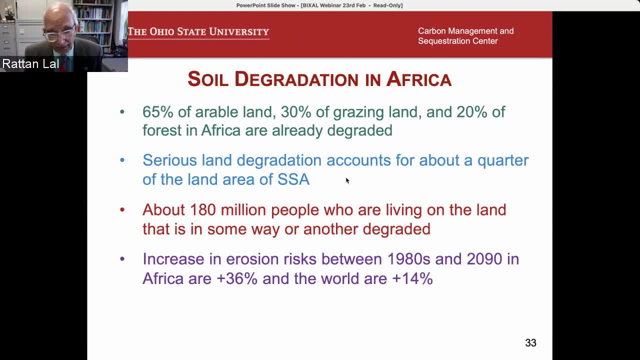 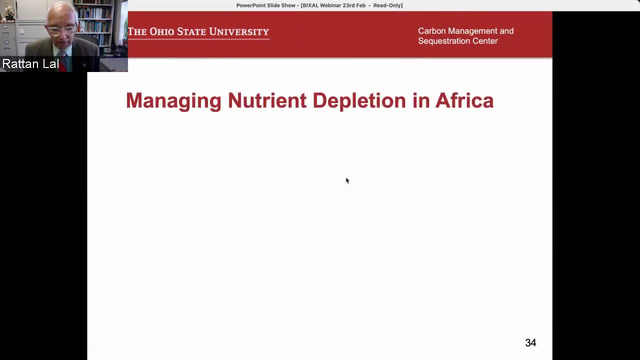 end of the century in southern africa, sub-saharan africa, maybe additional 30 to 40 percent, which is really a cause of food insecurity. i personally believe that the green revolution bypassed sub-saharan africa because the soil resources were neglected, are still being neglected. nutrient management global. 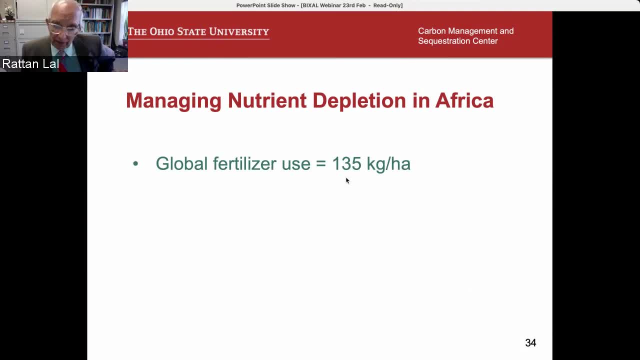 fertilizer use 135 kilogram per hectare. global average- sub-saharan africa: 17 kilogram per hectare. yesterday i checked the number: it's about 18 to 19 kilogram. 20 percent of the cropland area uses only two percent of the world fertilizer irrigation, which can alleviate drought. 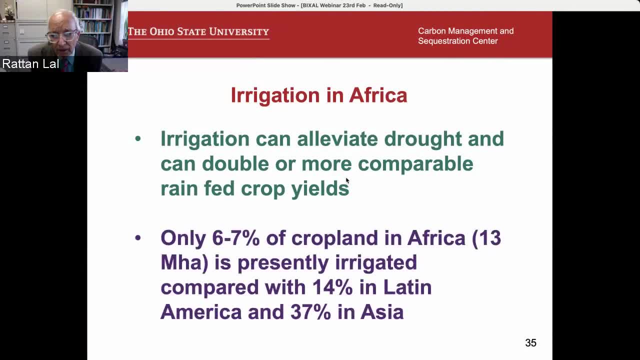 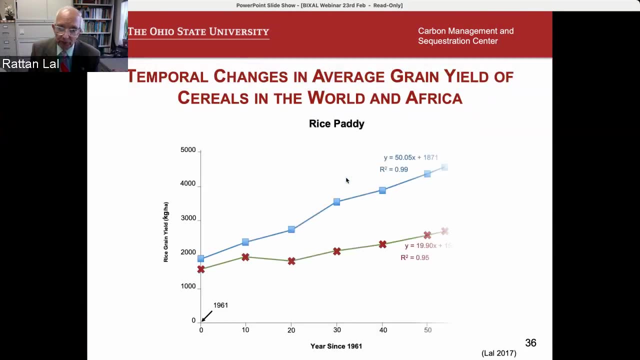 only seven percent of cropland in area. in africa, about 13 to 15 million hectare is presently irrigated, compared with 40 percent in asia and 15 14. so drips of fertigation that saves water should be a very good option because of the degradation. look at the trend in rice production. 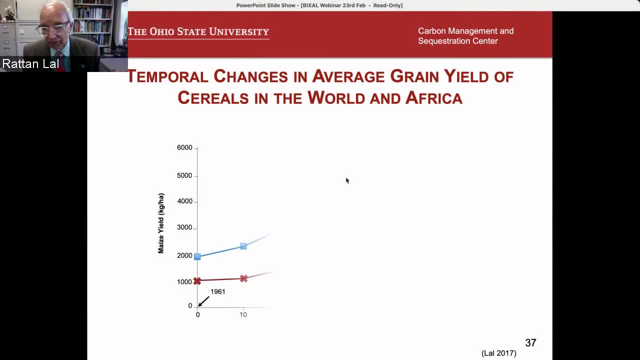 in africa, in the world, and still big yield gap, maize production the same way, big yield gap, and this yield gap is soil quality not being managed properly. so, while health not being restored properly, it cannot happen otherwise. so let's take, in the case of a road map, what should happen? 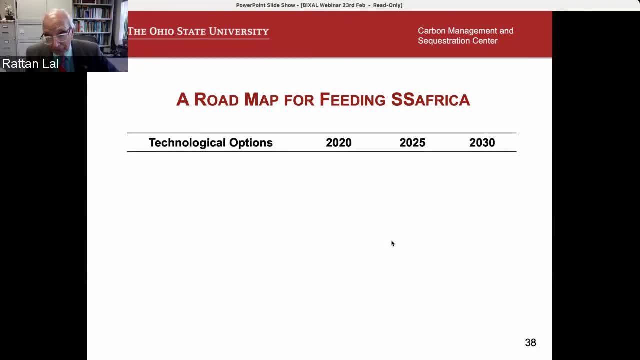 in sub-saharan africa between now and 2030. for example, on a short period of time, fertile other use: from 13, 15, 17 kilogram go up to 60 kilogram. irrigated land area from seven percent to twenty percent. conservation agriculture on about one million hectare now get up to 50 million hectare. 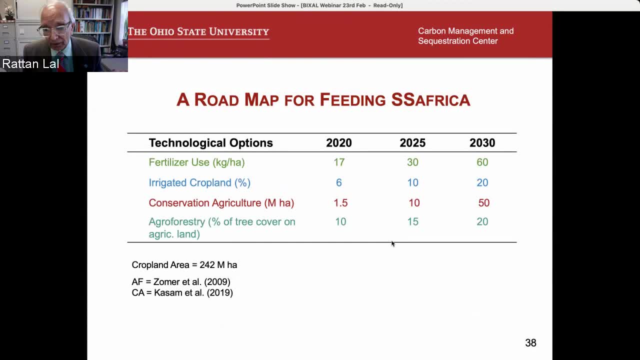 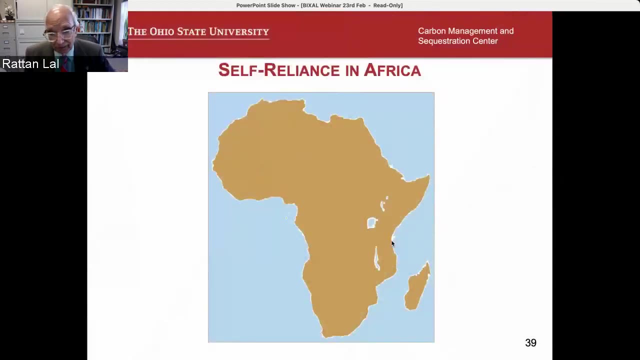 agroforestry, maybe ten percent now, a total area twenty. we must have some guidelines, some agenda, some program and we must stick to it so that we can achieve so 2030 sustainable development goal. africa has a road map that we must try to achieve. it's a challenge but i think, trying to 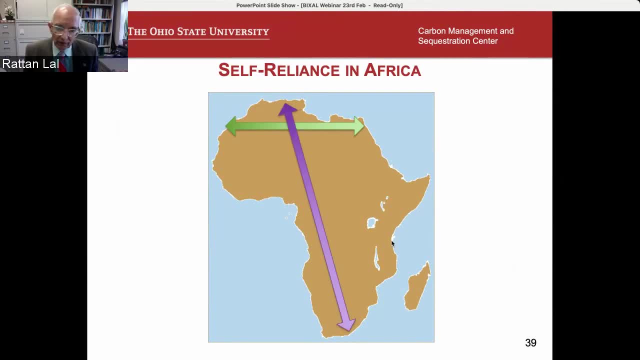 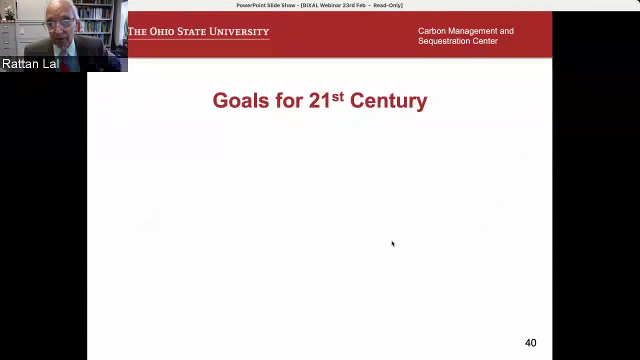 develop some benchmark studies. uh, where you, on a community-based implement what we were talking about? uh, it is possible, it's doable, it's something within next eight year we must try. so the goals for the 21st century: globally return land to nature. how much? ten percent per decade out of. 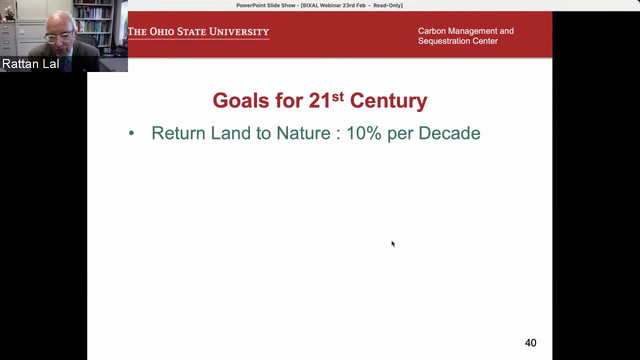 five billion hectare every decade. ten percent return back to nature. stick to that agenda. restore degraded land. we got two billion hectare to get land degradation neutrality. if you are getting a new degradation, 10 billion, restore at least 10 billion, preferably more. the goal for the 21st century is the recovery of the natural system. 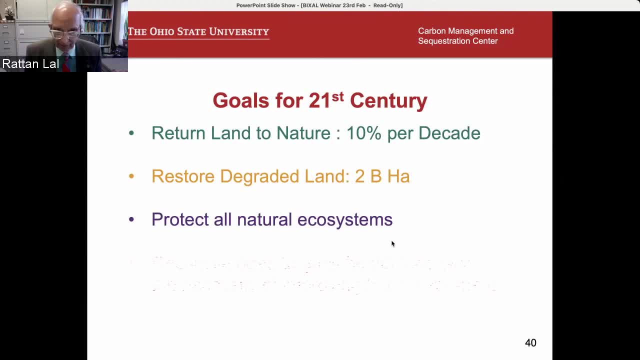 so it's not about changing the system and changing the way the system works. do not just save the environment, but also protect natural ecosystem. and the other part: protect all existing natural ecosystem. do not convert them or human use. protect natural system. we must reconcile the need to grow healthy food. 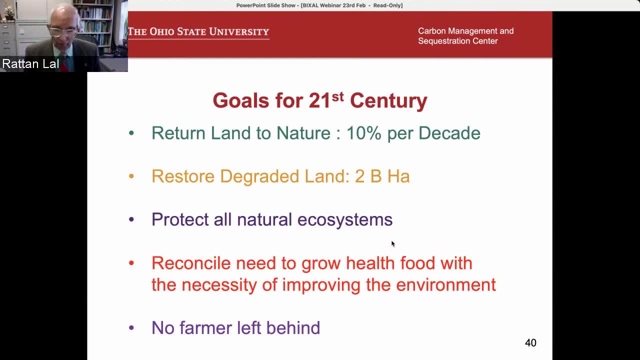 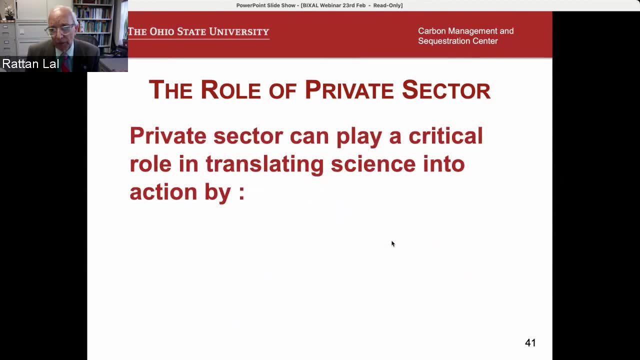 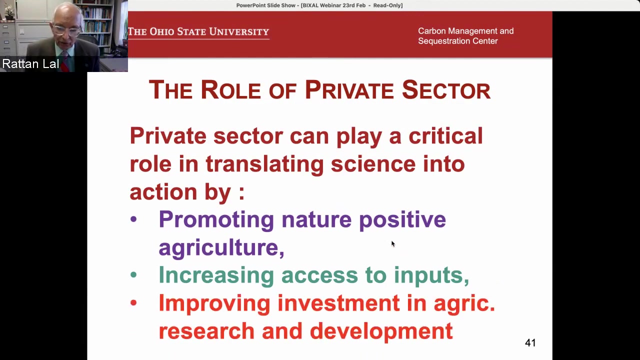 million hectare of them. they cannot be ignored. no farmer can be ignored, no farmer, but especially small farmers. in this regard, the private sector may have a very important role to play. private sector a tremendous thing in translating science into action, in promoting nature positive agriculture, in increasing access to import and in improving investment in agriculture. 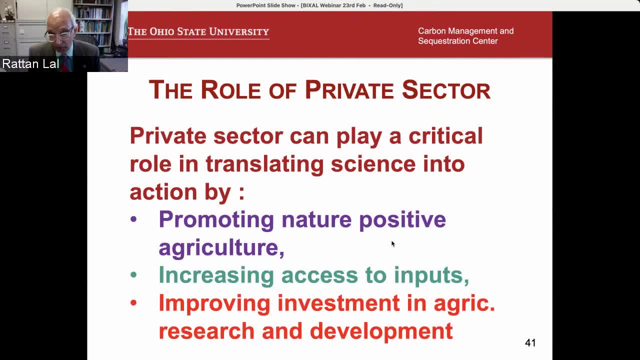 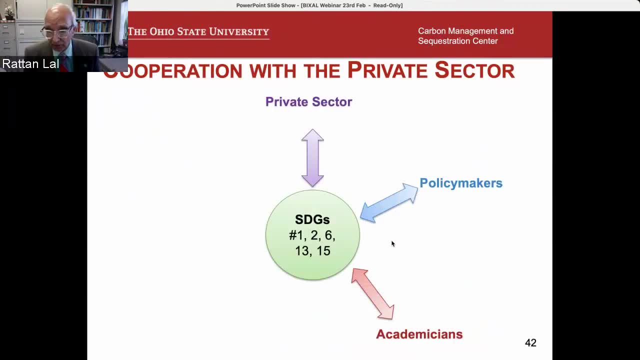 research and development. i can never, ever overemphasize the role of private sector, the combination of private sector with policy makers, with academicians, with international organizations, with land managers, that's farmer. sustainable development goals such as number one, number two, number six, number 13, number 15 can only be met through this kind of very positive 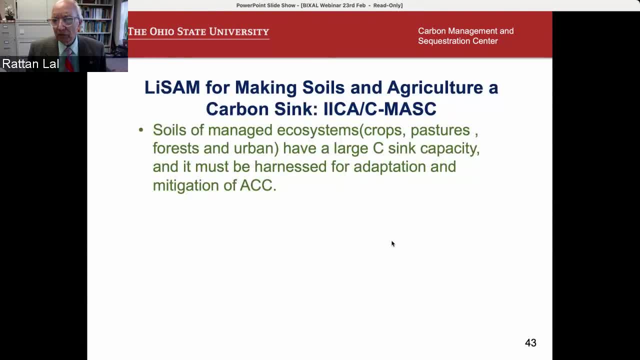 cynicism. i want to mention a license program living soils of the americas eka and ohio state are implementing together. the idea is that the soil is a living entity and that life-giving processes of the soil must be enhanced, must be restored, must be judiciously managed, and while doing that, we can also, of course, sequester carbon. 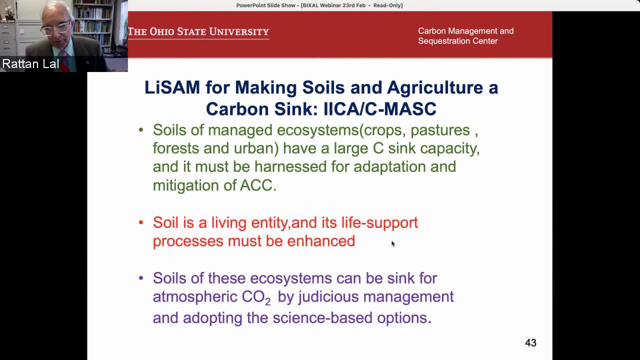 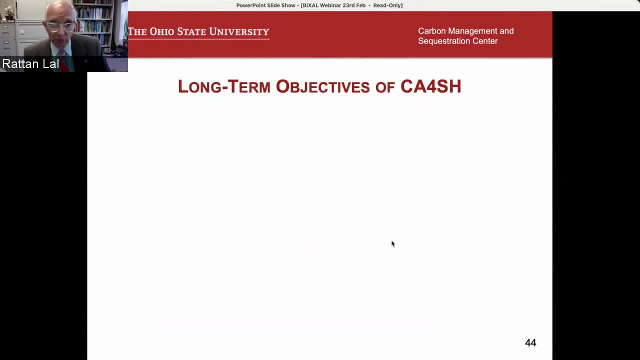 in soil. hopefully, this program can also be implemented not only just out all through america- four countries- but also in africa, asia and elsewhere. the long-term objective are also being considered very actively as we speak by a program called cash, that is, coalition for soil health management. that emerged from the food system summit and this cash. 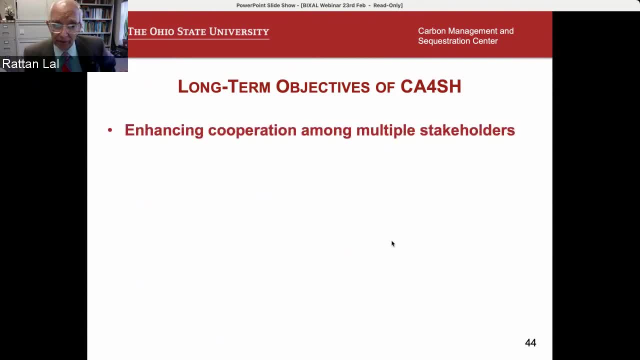 has already got support from 110 member nation. to do what? to enhance cooperation among multiple state holders. to promote on the ground adoption of best management practices. to develop tools for measurement, monitoring, verification of soil health and its indicators globally. to advocate a system-based soil health agenda. to implement an action plan for restoring soil health. 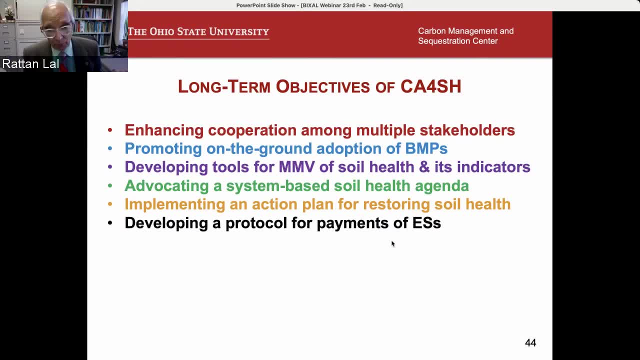 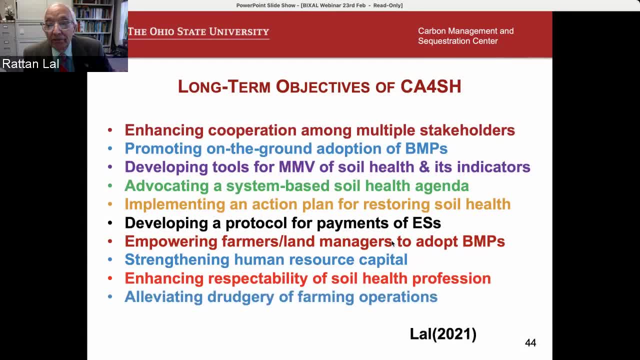 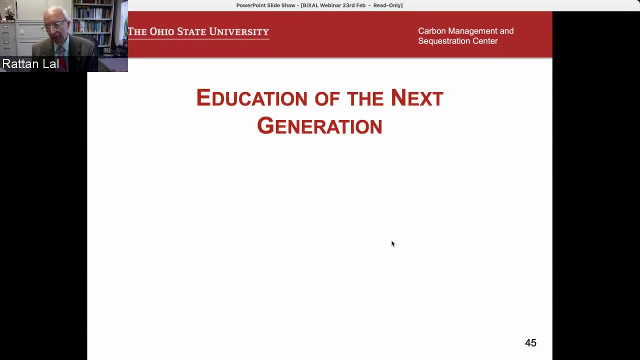 i want to mention the word respectability and alleviated drudgery of the farming operations. the whole, the whole based agriculture, the manual, the hardship, somewhere we need to improve all those parts. and that brings the last topic: education of the next generation. in addition to three arts, goal of the education is to be 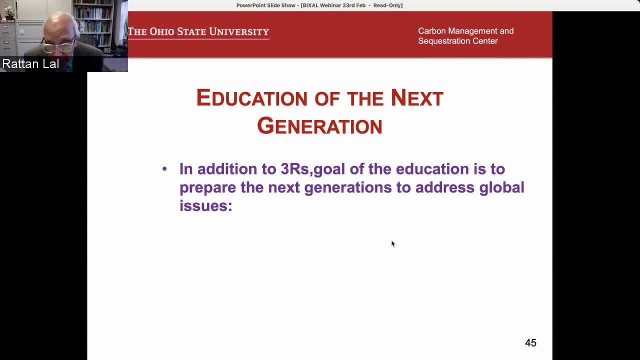 prepared the next generation to address global issues which we discussed, 10 of them: food and nutrition, environment, soil, water, air, global warming, personal responsibility, culprit and victim as we talked about it. ethics, integrity and professionalism in respect for nature. respect for nature: do not take nature for granted. in this regard, connecting children with nature. 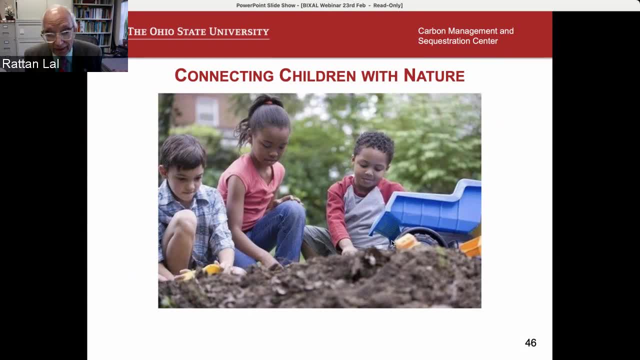 right from the beginning, from the kindergarten stage, is very critical. i would like to see children letter books, alphabet book written in a way that emphasizes nature, that emphasizes agriculture, that emphasizes soil, so the children know where the food comes from and what a healthy soil look like, and this is something which is. 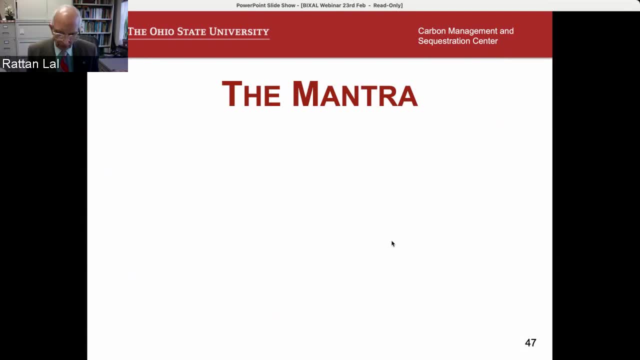 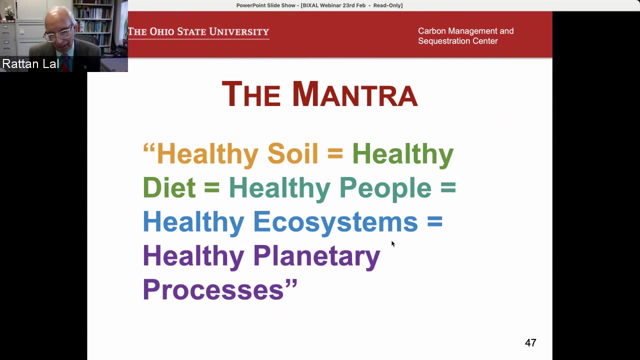 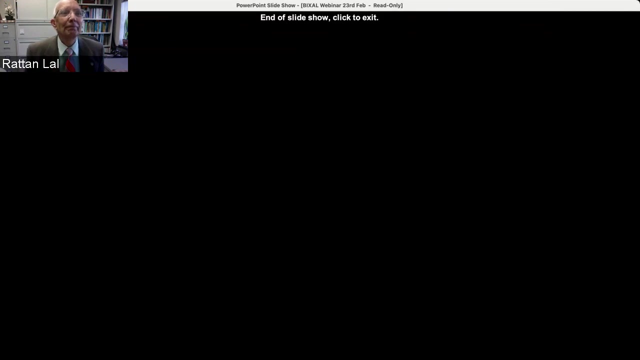 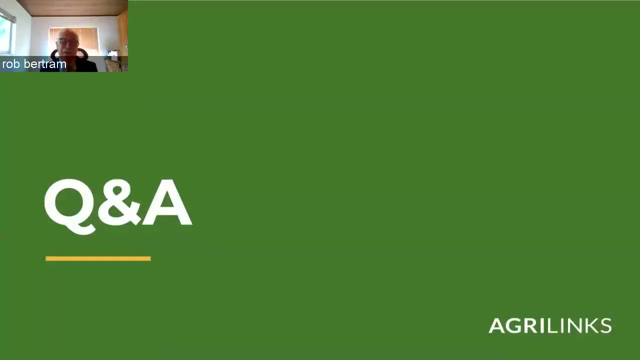 a mantra that should be teaching to our children from the very beginning, and that is the healthy soil, equal to healthy diet, equal to healthy people, equal to healthy ecosystem, equal to healthy planetary processes. mike and rob, thank you for the opportunity. well, thank you so much, rattan. uh, what a tour de force you've given us. i know all of us at 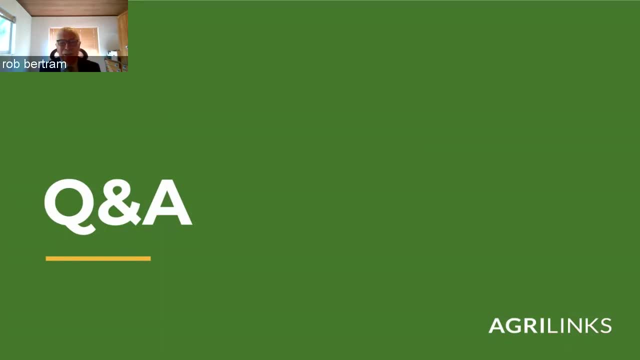 usaid have been very excited uh looking forward to your talk today, and i think everybody- almost 300 people- have been watching this and many more- will see the recording and i believe that they uh will be able to see the recording, and i think everybody will be able to see the recording, and 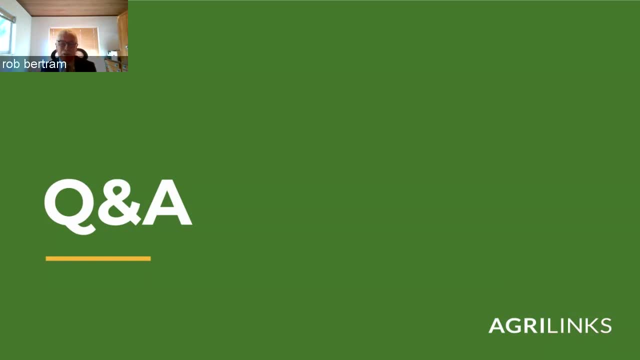 we know why people came: because you have done such a fantastic job at integrating these global challenges and and and showing us so many things, and your, your talk, has stimulated many questions, rattan, so i'm going to try my best to uh do them uh justice. um, let's start with one from albin. 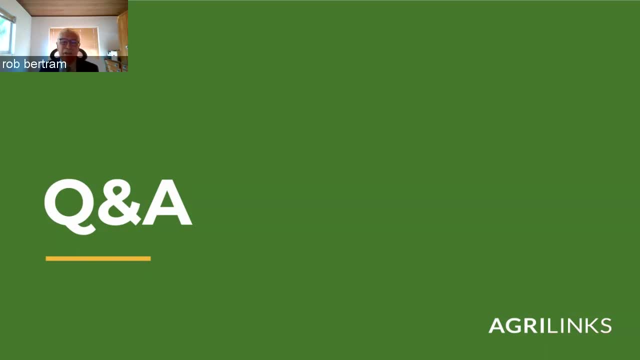 hoopsher, the director general of the international fertilizer development center. uh, dr lowell, you indicate that agriculture produces 30 to 35 percent of greenhouse gas emission. other sources suggest 18 to 20 percent. what is the difference? i think i know, but i'm going to ask you. rattan, you're. 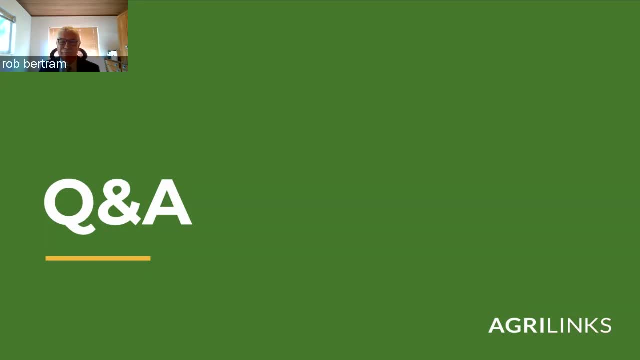 the expert, you caught my mistake. it should be food system that produced 30 percent agriculture. producing food itself is 14, 18, correct? when you combine food production with the entire food supply chain then it becomes 30 percent. yeah, i think that rattan, if i might. where does land use conversion? 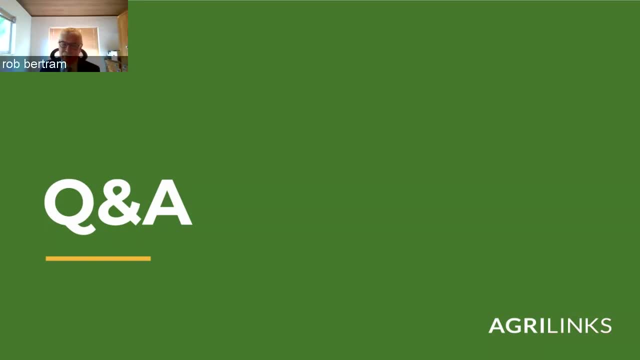 uh fit into that. it's also very substantial, very substantial globally. rob land use conversion is one gigaton uh per year. even last year it was 0.9 gigaton. so if we can stop uh converting natural ecosystem to agriculture, we can also decrease uh emission from the land-based system. 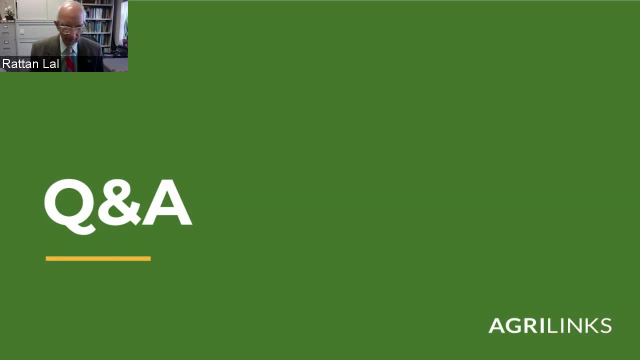 my personal opinion is that this estimate of agriculture is less than what it can be. for example, soil erosion is a major source of emission of gases and 24 gigaton of soil is transported by hydrogen erosion, and the estimate of the carbon cycle from erosion does not appear in some of those one gigaton land use conversion. 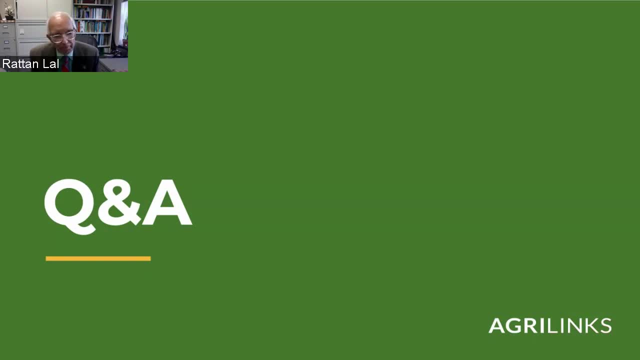 part. so these things are a little bit of guesstimate, need to be improved. but, alvin, you are right, it is total food supply chain, foods system. that is 30 percent and, if i might, given dr hoopsure's location at the fertilizer center, i thought it was fascinating, rattan, how you could build some food. 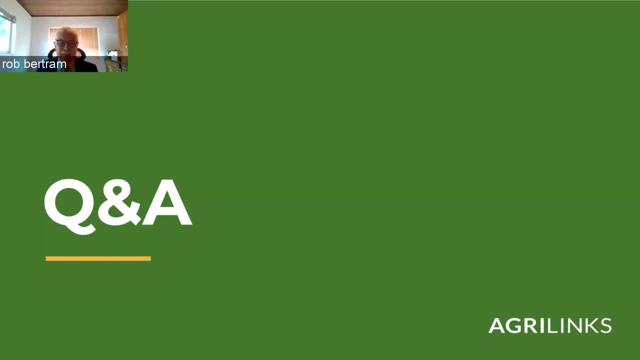 and use it as well. absolutely, you connected carbon sequestration to soil fertility and to the addition of nutrients. this is something that isn't necessarily intuitive for many of us, so this is a i mean. perhaps we'll talk more about that now. the next question i'd like to pose to you is from sabrina burner. can you address? 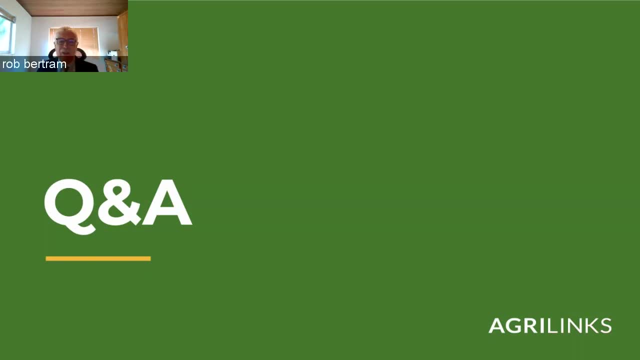 one the timing required for carbon sequestration in the soil and two effective, credible and affordable systems to measure soil carbon sequestration. so two different questions but very related, i think, very, very good question. i want to go back to the previous question. it is very correct that improving soil health will increase the use efficiency of fertilizer. 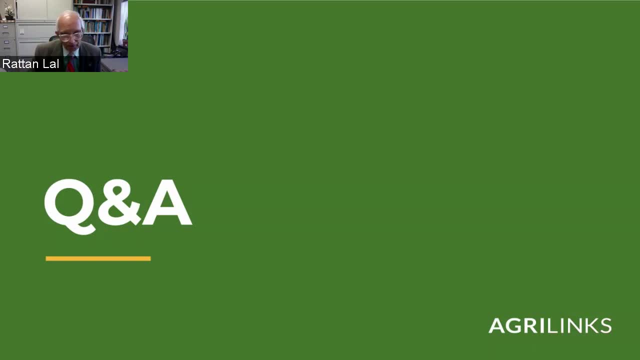 therefore decrease the rate of fertilizer which is applied. i was very surprised the other day reading a paper: fertilizer used in punjab- east punjab- is 240 kilogram per hectare, global average 135 at china, somewhere even 400 kilogram per hectare. we cannot continue, keep increasing the rate. somewhere we have to restore soil health. 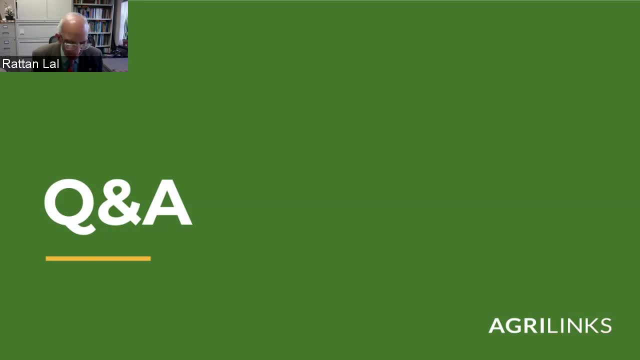 decrease rate, improve efficiency. now carbon sequestration. yes, the rate of carbon sequestration under ideal condition in cropland is really our organic carbon, probably about one ton of carbon per hectare. in the west, for example, some people have monitored one and a half ton, but i think one ton average. 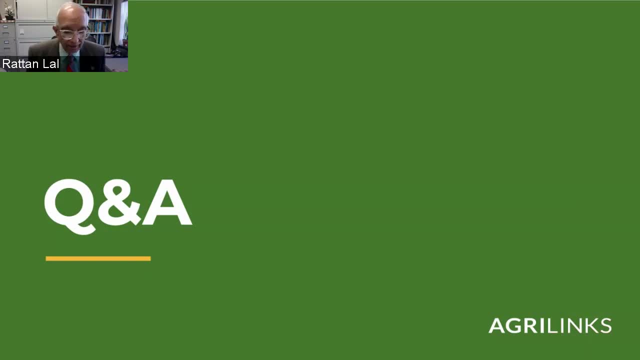 and if you are an arid climate maybe the rate is less. in addition to organic carbon, probably uh inorganic carbon, secondary carbonates and bicarbonate is another part, but the rate of carbon sequestration inorganic is very slightly less and the impact on crop growth of that on. 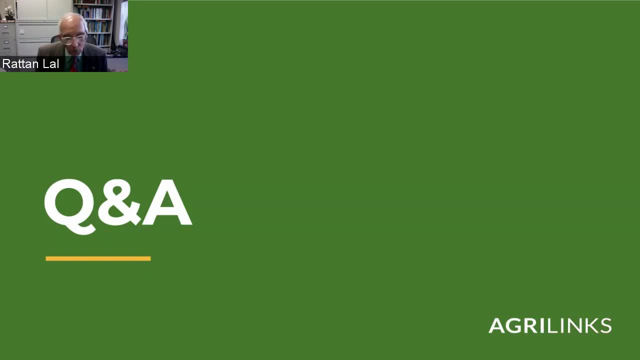 our study, so it's a slow process. while i remember working in africa and nigeria, i lost 50 percent of carbon in almost 5 to 10 years after deforestation. in temperate climate maybe 50 year where you lose 50 percent, but the gain is very slow. it's a slow process. so a new equilibrium of a soil carbon, after adopting, say, conservation agriculture, would be 25 years a generation, so it's a slow process. measurement monitoring is a very good question. uh, yes, the time involved in sampling soil, in preparing sample, grinding, bringing to the lab and analyzing is not only time consuming but also expensive. but i'm very pleased to report. 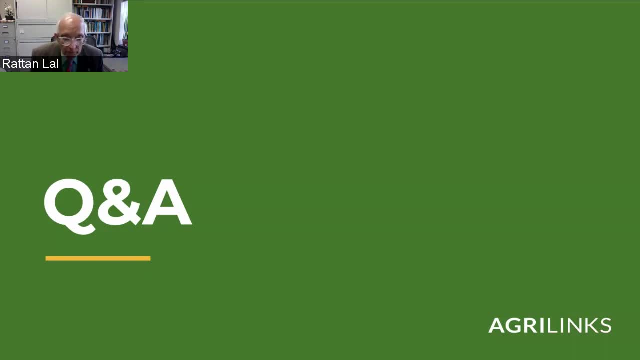 that devices are being developed which can be used in field. i have one uh which cost about 400. it has been huge in malawi and elsewhere by several colleagues. new devices are coming up as we speak. we have a project funded by microsoft. they have a handheld. 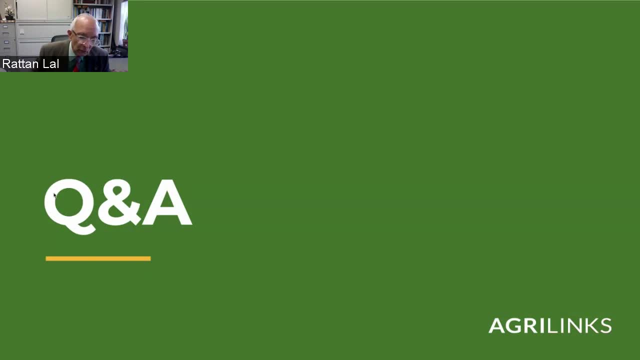 wi-fi to monitor organic matter content. we are working, then, now to improve it to convert also not only moisture but soil organic carbon. a lot of progress is going to happen within the next two to five years and this is a very important part i've been mentioning to my 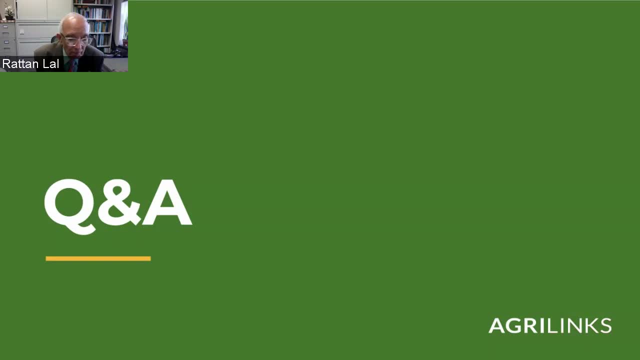 colleague, the biggest breakthrough will happen when a farmer has a wi-fi and they can monitor soil health parameter, such as carbon and water, by themselves in the field at a very low low cost. we are on the path toward that direction. it will happen soon. great, thank you, dr lal. one follow-on from dr berner. again she talks about acidification. 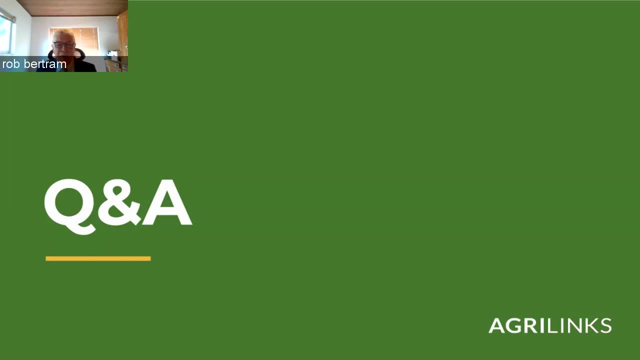 of soils, uh with fertilizer use in west africa and she's asking about, uh, the use of lime, which we know prominently in brazil, for example. yes, acidification, especially with nitrogenous fertilizer, is a serious problem. uh, i was working and on alphysos in ibadan, nigeria, and we were using only uh 60. 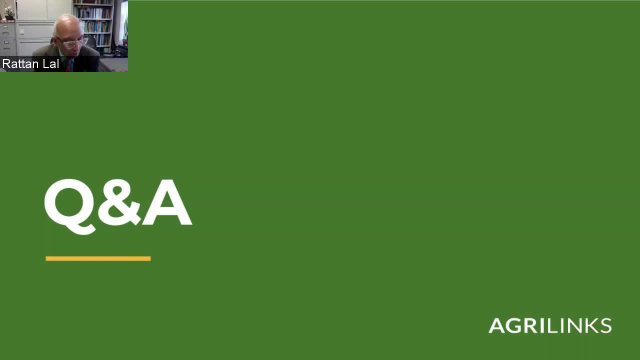 kilogram of nitrogen and those so all with low activity clay locate ionization capacity. so over 17 year period our experiment showed that even at that small rate the ph went from 7 to 5.5, some cases 5.. so acidification has to be addressed if you maintain the organic matter. 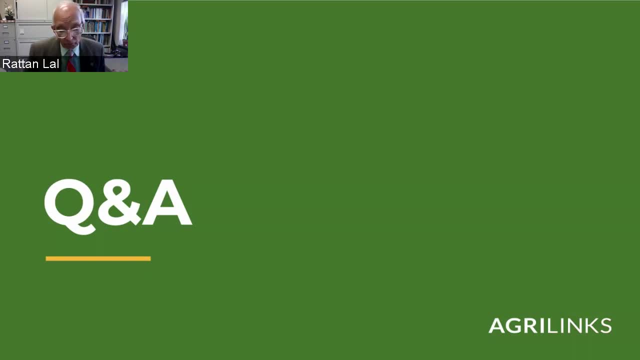 content. of course, that will create more buffering capacity. it will increase cation exchange capacity, uh, it will resist the rapid decline. liming definitely is a very important part, so it's not only c and pk, it's c and pk's and ca, calcium, calcium, calcium calcium. 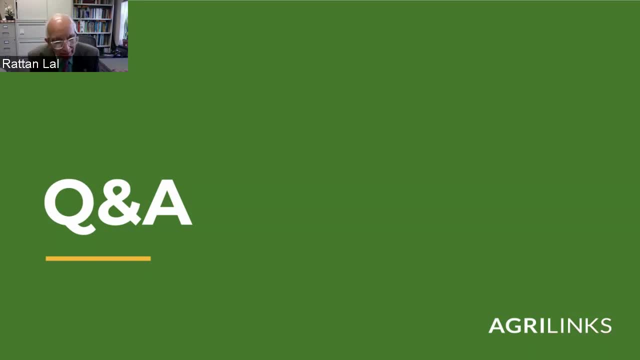 magnesium. that's the lime. so, and that's what the integrated soil fertility management is right, thank you. i want to speak to the audience here for a second and just tell you we have an embarrassment of riches in terms of questions. i'm trying to pick out a few. 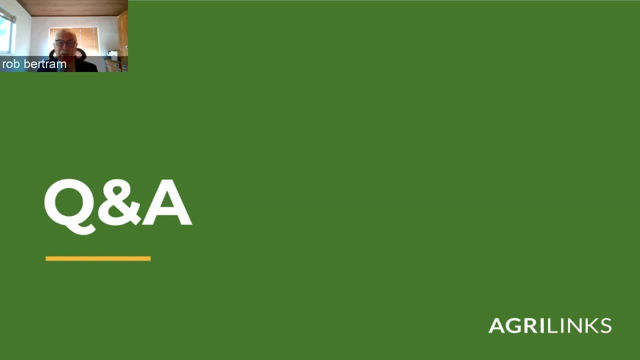 technical questions to begin with, and then we'll move on to some that are at a higher level and and then some challenging questions as well, some scenario questions. i hope everybody will be able to stay with us. we have a good period available, uh, for discussion this morning. so uh, turning uh. 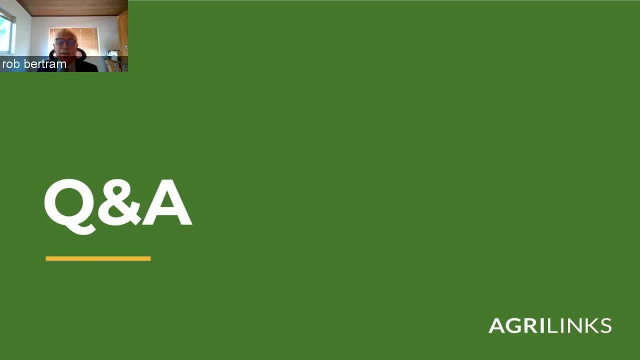 to a next question. um, let's look at um which. uh, we have a question about peak phosphorus. uh, can you speak to that one? yes, um, please, Terry Fowler. Dr Terry Fowler, This was a topic about 10 years ago that we were running out of phosphorus. 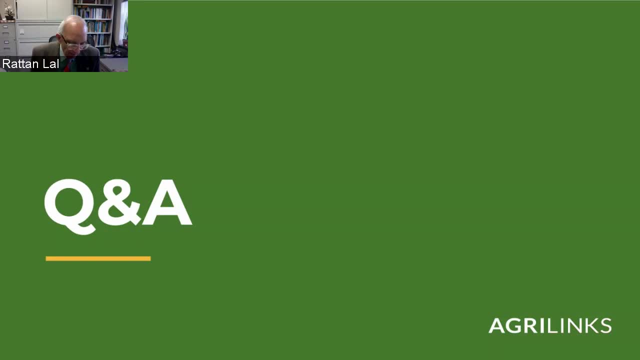 I think, since then, recent data have come out from several sources, both in Europe and US and elsewhere, that there are a lot more phosphorus reserves available, proven than what we thought 10, 15 years ago. But, having said that, making sure that phosphorus is recycled is very important. 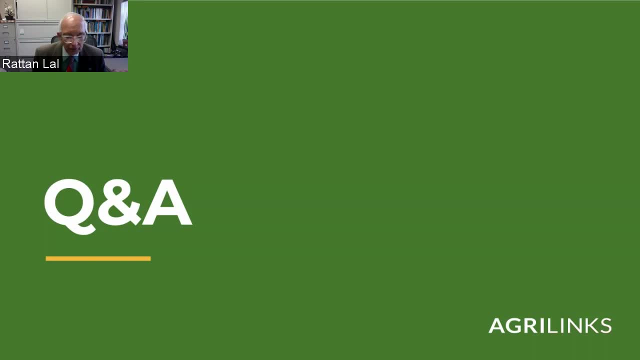 Let me give you an example of megacities, where a city of 10 million people requires 6,000 tons of food, which of course the nutrients like phosphorus coming into the city. So recycling those nutrients to produce 15,, 10, 20 percent of green food within the city limits. 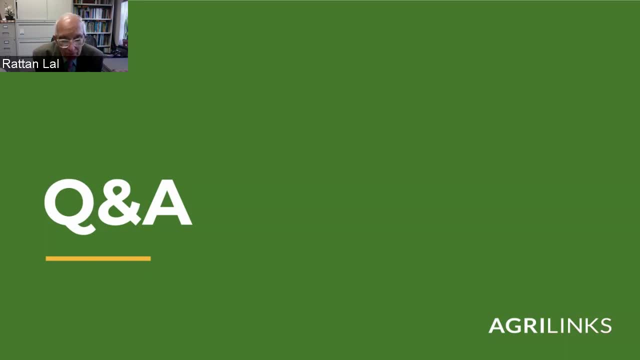 By recycling. something has to be given more and more importance, even recycling of animal waste and crop residue. So the nutrients like phosphorus are recycled. So although the peak of danger, even if we say we have a phosphorus enough, rather than for 50 years, for 500 years, in a planetary and human scale, even 500 years is a little bit of frightening. 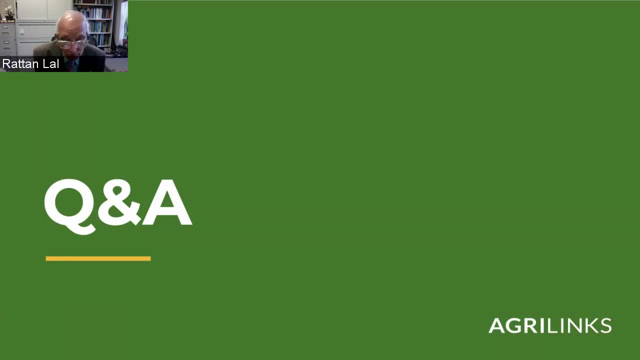 So recycling, Recycling the limited finite resources, using them properly, avoiding overuse, is very critical. You remember 5R I had. P is a very good candidate for that. Thank you, Ratan. Catherine Reby writes: do not many fertilizers also contribute to soil degradation in the long term? 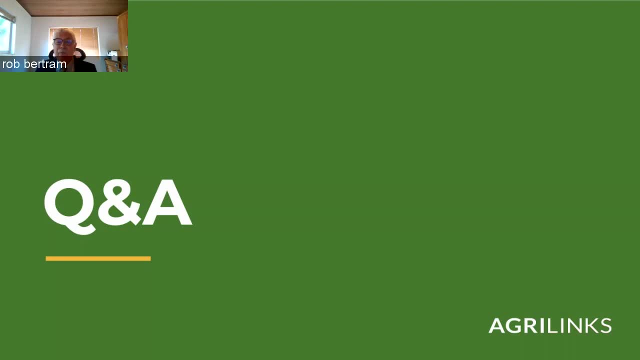 What kind of increased fertilizer use is being promoted? And, if I might Ratan, it seems to me like you're laying out a scenario where, in some parts of the world, we should be using less, far less, and in some parts of the world, we should be using more. 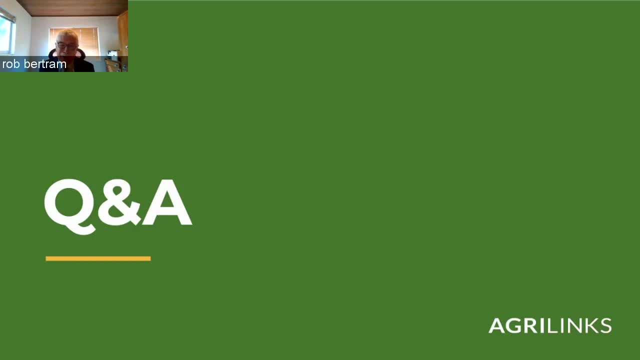 Yes, Let me turn that question back to you now. Absolutely, Rob, as I mentioned China- and I was surprised about India and Punjab- 240 kilogram and China 300, 400 kilogram. That's overuse. 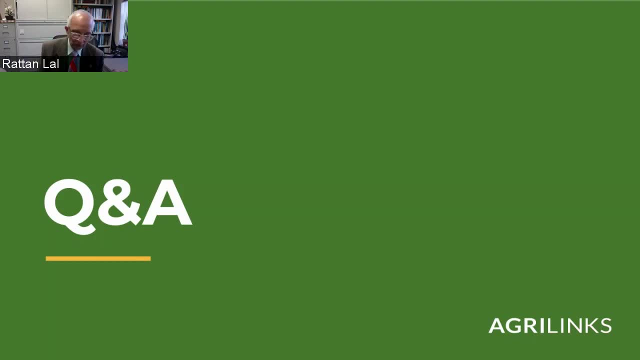 That's excessive use, That's harmful use. It's something not a good thing to do. So use efficiency should be improved. But on the other hand, Africa, which has sub-Saharan Africa, has a 30 to 40 kilogram per hectare of negative nutrient budget per year. 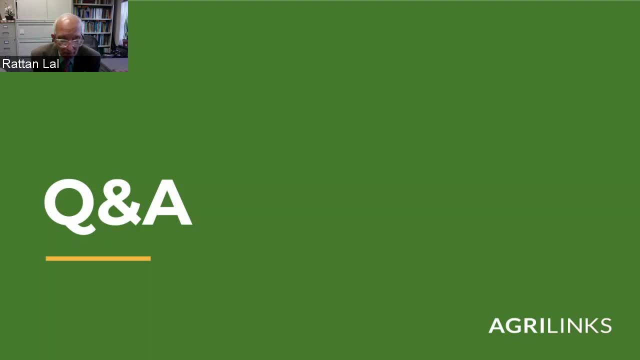 30 to 40 kilogram. And remember the law of return. The law of return says: anything that you take out from soil Nature, you must put it back to the same place one way or the other. So I do not want to go into the question of how the depleted nutrients are returned, but it's very important that they are returned. 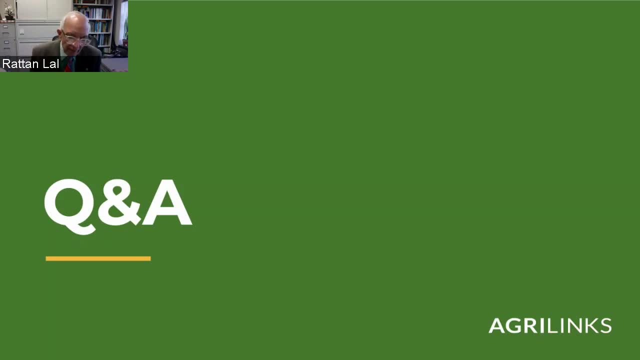 Soil, my friend, is like a bank account: You can never, ever take more out of a bank than what you deposited in it. So, the same way, you cannot take out more nutrients out of it than what you replace on a continuous basis. 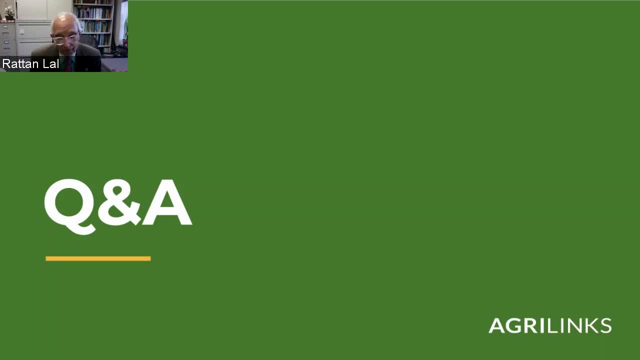 Without degrading soil health. So fertilizer, yes, they have their own issues that need to be addressed, but it is one thing that can immediately and quickly provide the nutrients. But on a long term basis, I think if we manage soil health, soil organic matter content, which should be about 3,, 4, 5 percent in the root zone, the need for high rate can certainly be eliminated. 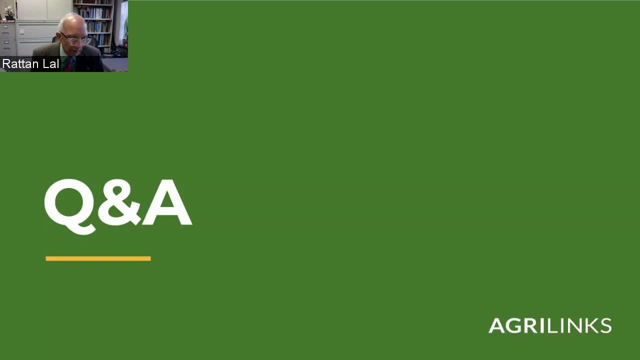 I do want to mention Rob one thing. many people think that perhaps we can do feed 11 billion people without putting chemical. The amount of food we require and the quality of food we require must consider balanced application of nutrients in soil. They have to come from somewhere. 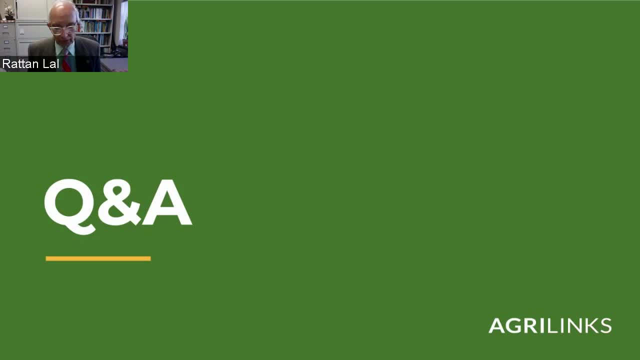 And if that somewhere recycling, biological fixation is not enough, then the judicious use of fertilizer is very critical. Remember, the difference between poison and remedy is a dose and time. So the dose of application of fertilizer and the time is very critical. Thank you, 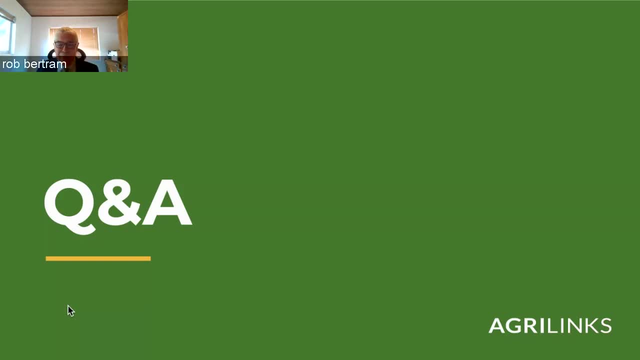 One thing I wanted to underscore, that you said a few minutes ago but I think bears repeating, is that when we have more carbon in the soil, our fertilizer use is more efficient. In other words, we can use less fertilizer just by virtue of the fact of the soil being 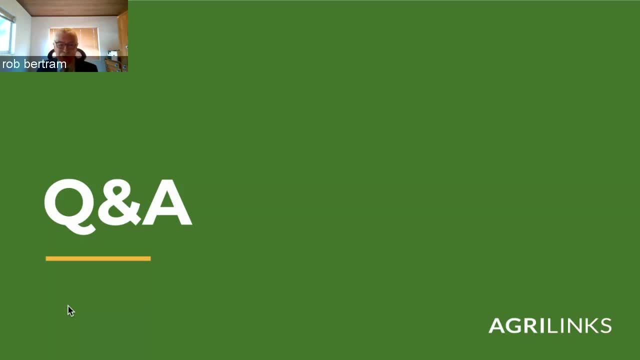 Healthier, and and so this is a this is a synergistic process. so let's turn to this issue of carbon in soils, and we'll start with a question from Dr Claudia Ringler at the International Food Policy Research Institute. She asks in terms of how to compensate farmers for improving soil health. 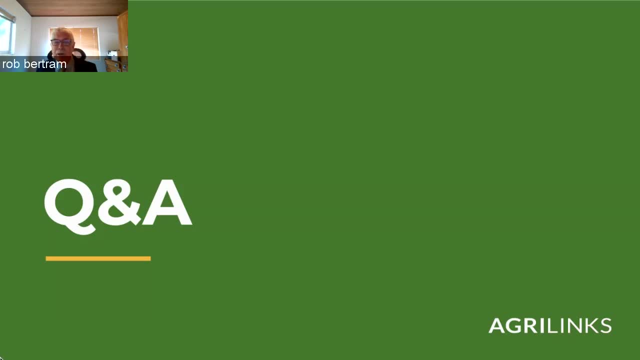 There is a concept of quote charismatic carbon, In other words, acknowledgement of co-benefits, restoring soil carbon first. So this is getting at this, this challenge that would be inherent in what you've laid out. Thank you, I think I fully agree with what Claudia says. 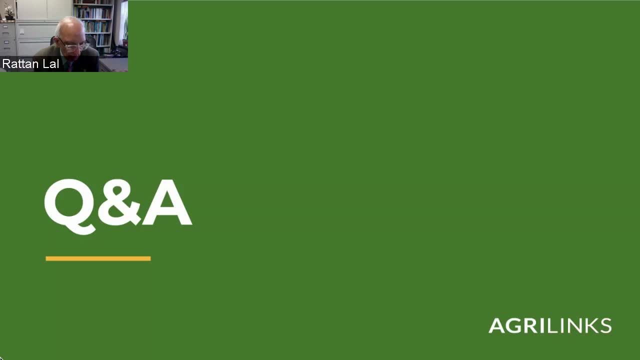 If we can improve the carbon stock and soil, Both the quality and the quantity, Several inputs will be decreased automatically. irrigation water requirement. In fact there is a data: If you increase organic carbon by one ton, much water irrigation, do you say? 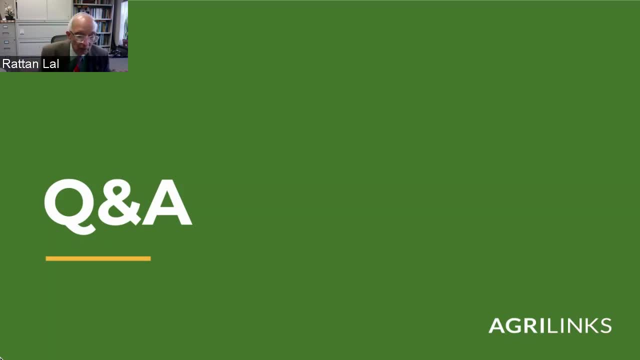 Because of the Increase in water holding capacity. So there's a data on how much nitrogen you can save by increasing the organic carbon content. input: phosphorus The same thing: The tillage, the soil structure is improved when they saw organic matter is good. 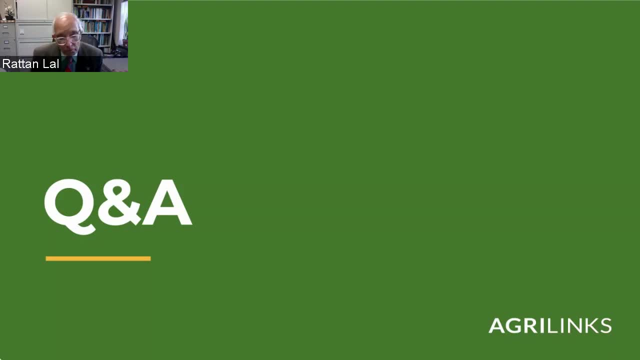 So energy saving is also there, So there are co-benefits of improving soil health. The part that we have to think is that soil health has been degraded by long-term Land misuse and soil mismanagement. It cannot be immediately reversed overnight. 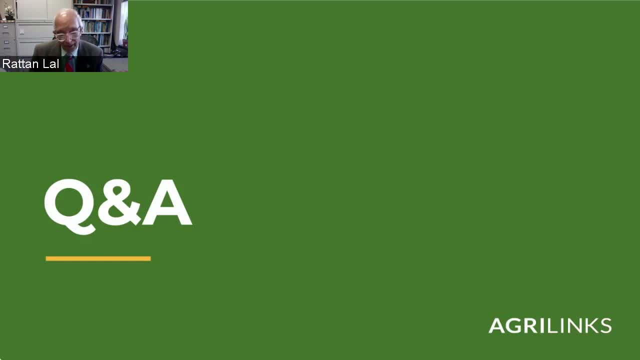 Restoration is going to take time and over that time period, when soil health is being restored by changing to restorative, regenerative agricultural practices, Farmer should be compensated So they do not have to suffer any financial losses. And that is where the ecosystem service is coming. 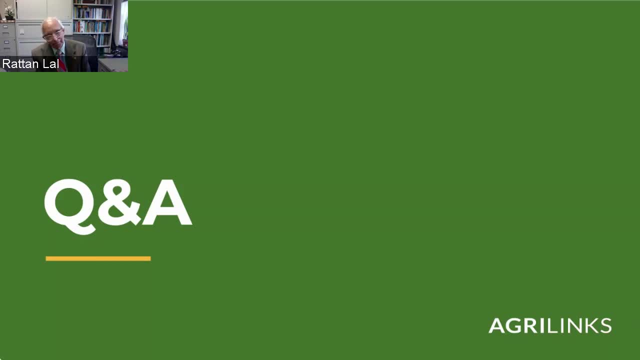 So Katie West asked: perhaps you mentioned this, but you mentioned paying smallholder farmers for the carbon. They return to the soil. Who are you proposing pays them First of all, the What is to be paid? and I did just say that very categorically: do not undervalue the such a precious carbon resource. 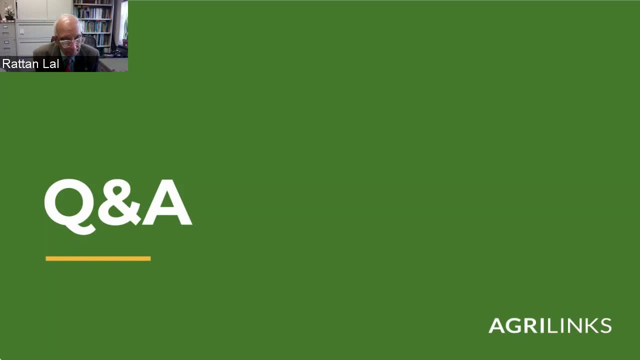 So paying farmer At the price of 30 to $35 per credit- and credit is one metric ton of CO2- is probably fair. That's similar to what the European Union is doing about 25 euro, So I think that's fair. who pays you and I pay? the public pays, the consumer pays. 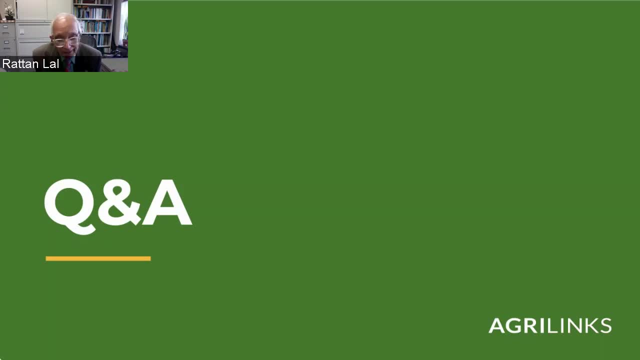 That's always the case. So eventually I suppose the farm commodity Price may have to go up. But in the meantime, industry- certainly I mentioned the role of private sector. some private sector I do not need to mention are already beginning to pay, But I think the payment has to be more than what is being paid. 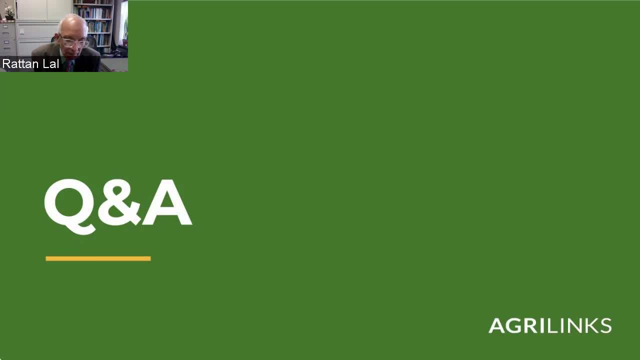 But eventually, the responsibility of payment to farmer is with the public, with us, with consumer, because we are the culprit and we are the victim. Therefore, we must take care of what we have done wrong. So the planet, Okay, thank you, Ratan. now, in this same idea, 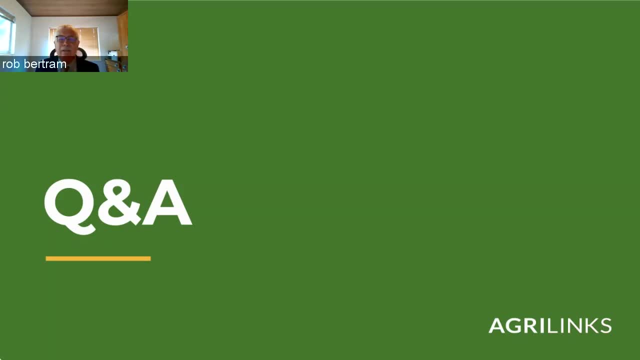 Luke Colavito from IDE says: Dr Lyle, the monitoring best soil practice is challenging. You mentioned some technologies to measure soil health. Do you see best practices in soil monitoring emerging? Do you see systems of certification like now done for organic, organic agriculture as a potential? 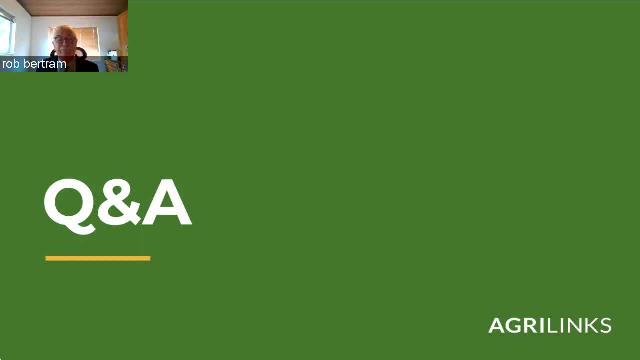 Or regenerative agriculture. Yes, I think you are very right, Not only monitoring the soil health- That's a impact of the native agriculture proxy- but to monitor of what is being done. I think remote sensing is really a very good option: satellite, the aerial photographs. 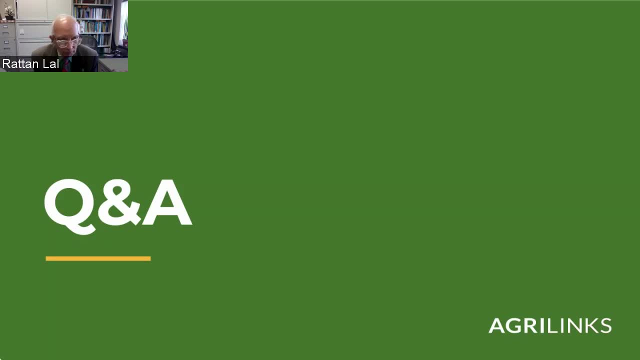 Let me give you an example. CRP was practiced. I stopped in 1987, farm bill in the US and eventually CRP, the conservation reserve program set aside, in European language, 40 million acres, 16 million hectare. We did not actually go to each and every farm and had a plume to monitor runoff and erosion. 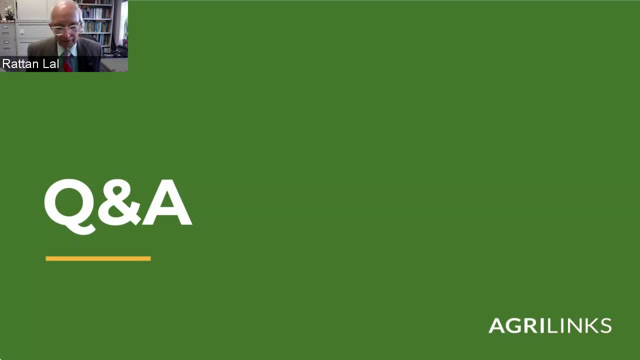 We from the satellite imagery, from the aerial photograph, saw that the farmers are not cultivating their land. It was set aside, It was And therefore we are paying them according to the data that was generated that way. I think it's the same thing going to happen in adoption of conservation agriculture. 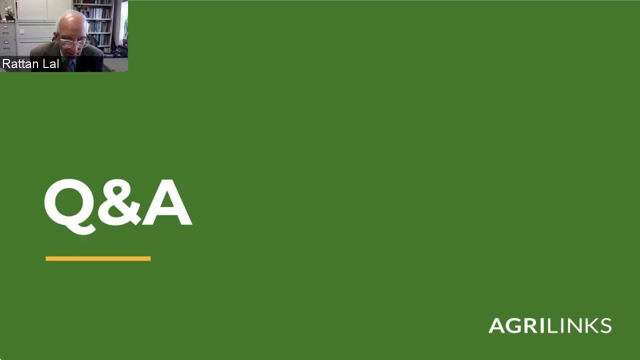 I call that as the best agriculture regenerative practice. So yes, we can evaluate conservation agriculture remote, sensely and, of course, ground to thing occasionally. but sometime we have to believe that the modern technology Can really provide answer to the land use. current land area under conservation agriculture: somewhere less than 200 million hectare of cropland. Maybe close to 180, most of it in the Americas, both north and south of Brazil, Argentina, Chile, US, Canada are doing quite well. Not so in Africa, not so much in Asia. I think we need to promote that practice again, Rewarding farmer and giving them the do that they really deserve. 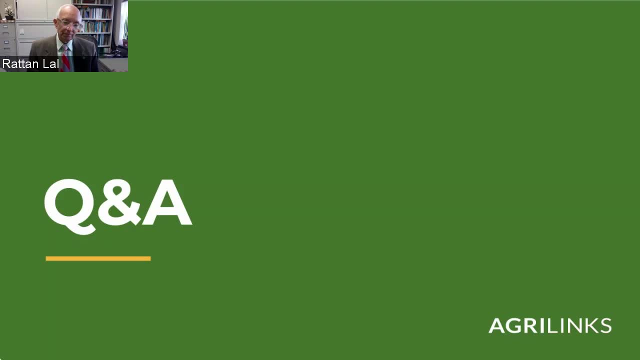 For the ecosystem services they create. Right, We have Something that Casey Aron has commented on. He says the aggregate impacts soil carbon sequestration should be interpreted carefully, which in the long run, can be lost quickly and go back to the atmosphere. 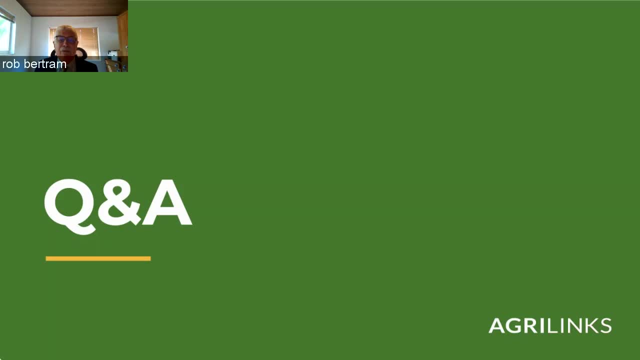 How can we deal with this? And then I'm also going to share a question from Kashlandra Tingi, who says: is there a method to provide carbon credits for agricultural products which have more than two years of utilization life cycle? So his examples are cotton and other fiber crops. In other words, trying to, I guess, see the life of the product as also a source of carbon being sequestered. 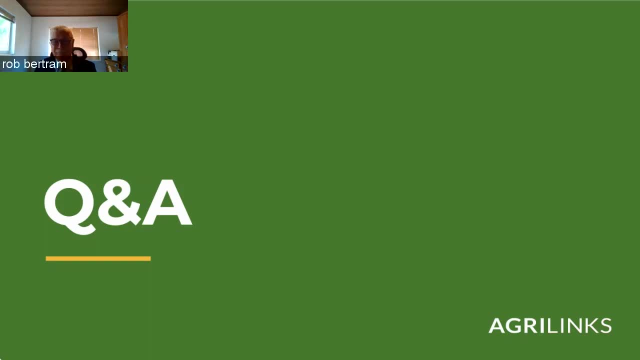 Thank you. Yes, Permanence part, Rob. it comes very often. The carbon that you sequester in soil, will it stay there? And of course, it's not a sequestration if it doesn't stay there. So please, 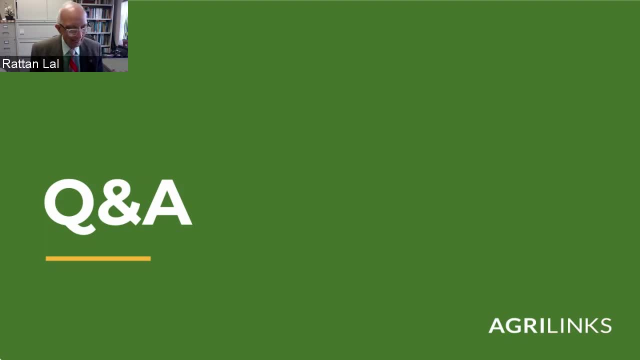 Remember, when I talk about carbon sequestration I mean it's going to stay there for decades, if not for centuries and millennia. And, of course, if carbon is protected properly in soil, we know that it can stay there for millennia. 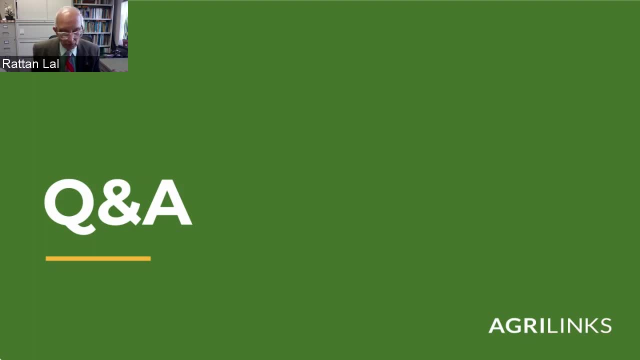 And what is proper protection? A- it's deeper in the subsoil. B- it is a formation of interaction with clay or susquexide, formation of so-called organomineral complexes, formation of carbon dioxide and so on. And, of course, if carbon is protected properly in soil, we know that it can stay there for decades, if not for centuries and millennia. And, of course, if carbon is protected properly in soil, we know that it can stay there for decades, if not for centuries and millennia. 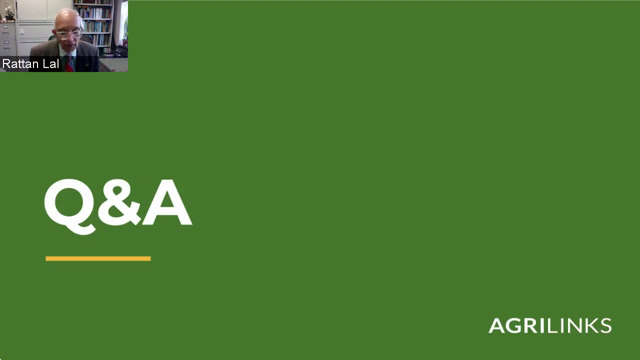 So it's a combination of stable aggregates And to achieve all this, eliminating fillage, mechanical tillage is the critical part. So, if you follow carbon sequestration practices that we are talking about, some people think conservation has three pillars. I think it has five pillars: No plowing, returning crop, residue growing cover, crop integrated soil fertility management and complex crop rotation. 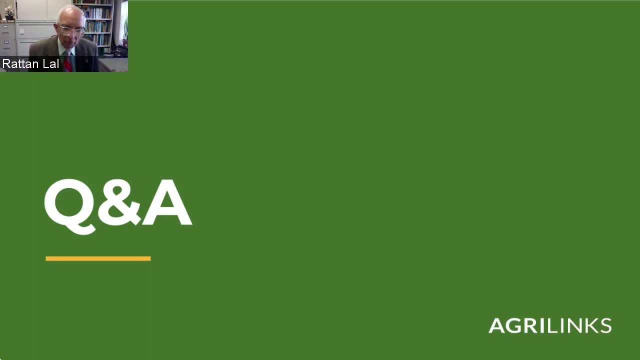 So if you follow carbon sequestration practices, then you can achieve all this. If you follow those five basic principles, where will the carbon go? It will stay in the ground. The question is making sure that those five components are followed. We should be able to check that by remote sensing, by satellite imagery, by aerial photograph, by ground-truthing occasionally. 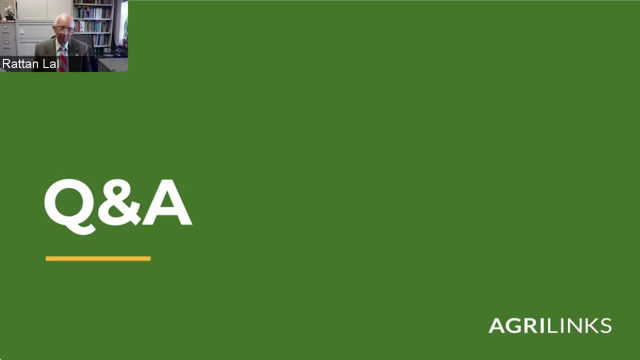 and pay farmers for doing exactly that. It will stay there. Yes, byproduct of the commodity. When these components are used properly, also sequester carbon. you're absolutely right. The typical example is wood, forest and forest. wood is used for long term development of even the homes, furniture, other things. 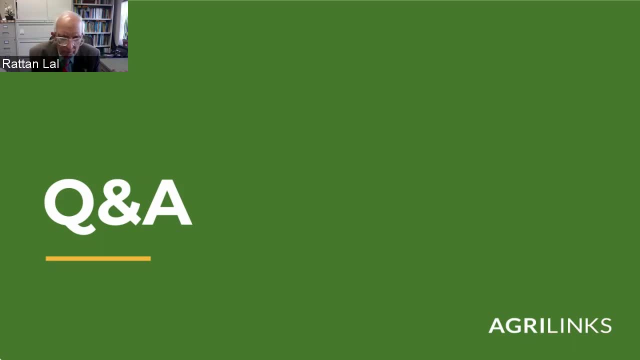 It's life for a long period of time. So payment for carbon credits should be based on how long is the carbon staying in the land based sink, for which farmland is Services. You're using it for forty days. It's time and time again. 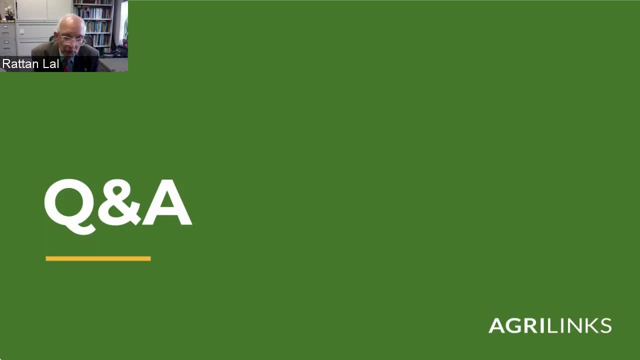 It's very important. It's not about time. It's about time, It's very important. It's very important. farmers are paid, so development of a proper protocol is certainly required. it's being talked about, being discussed about developing a indicator, key criteria, not only that, the carbon. 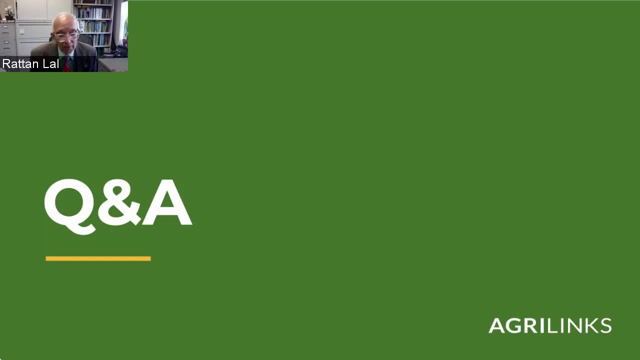 is put in the land, but it stays there over a longer period of time. farmers should be rewarded accordingly. so, um, thank you, ratan. peter sutton asks something about, uh, land restoration and rewilding. that's going to be a good term. you recommend we return land to nature at a huge scale. where will this? 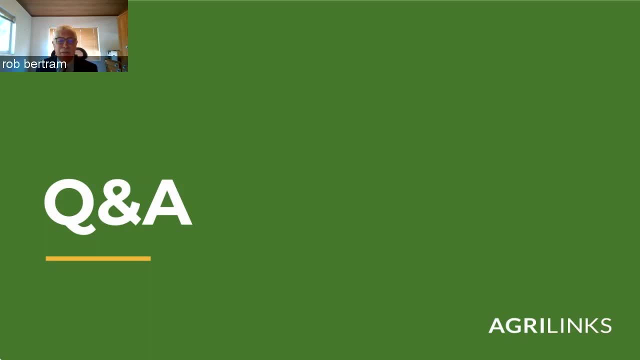 land come from and who will pay for it. another question of how this will be financed, and should we allocate ten percent of each farm or take out huge areas, and i think that's a thing that's going to be a good question, and i think that's a good question and i think that's. 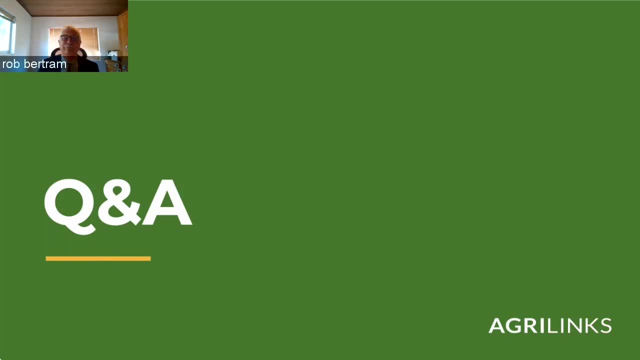 important question too. yeah, i, i think this is a very, very important philosophy. i'm concerned when i hear that we need 250 million more hectare by 2050, or 500 million more hectare- absolutely not. i think we have too much land already. so what in europe language called land? 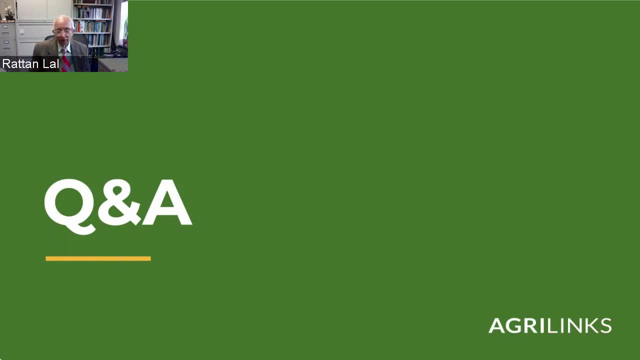 sparing and rewilding is what i call. land return is exactly the same concept, but human are already using 40 more percent, 40 percent of the land area. we don't need it. i have taken a board step and saying: why can't we return half of the land out of 5 billion? 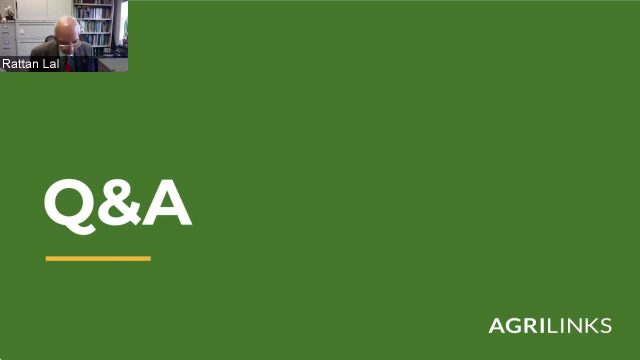 two and a half billion go back to nature, let's say by 2100. and where will it come from? well, it comes from uh a producing judiciously, making sure that the yield gap such that the yield gap is not reduced. and uh producing judiciously, making sure that the yield gap such that the yield gap is not reduced. 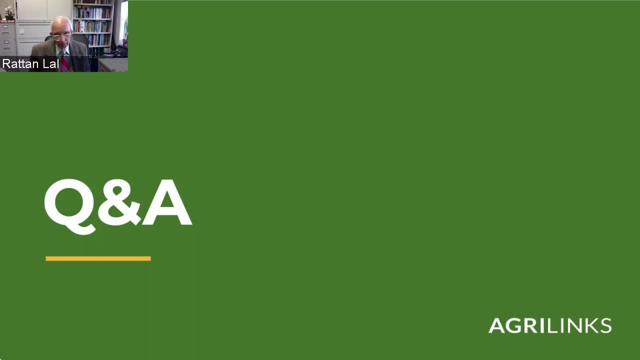 as in sub-Saharan Africa, probably tremendous yield gap, The yield of cereals at one and a half ton per hectare on a continental level, even the 70- my yield experiment was five ton per hectare. Why can't it be tripled or even quadrupled? Same thing in South Asia. 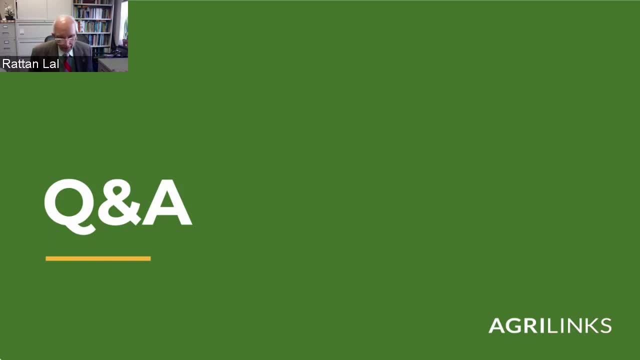 India. the cropland yield are not all that, especially of the rain fed agriculture, all that great In Indian condition. Africa quadrupled, India at least doubled. So bridging the yield gap is one where the land will come from The second part, where the land 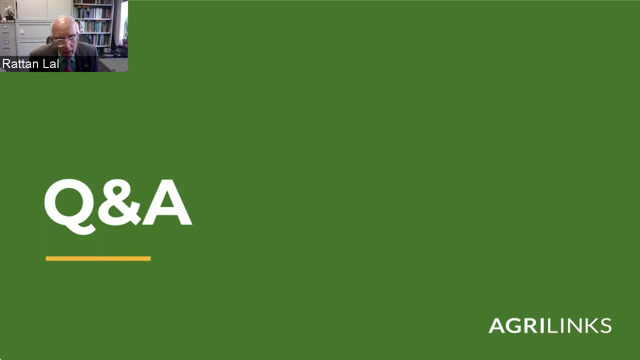 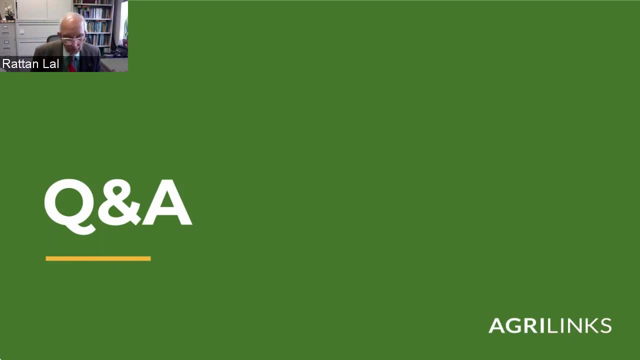 waste. even in the United States, Tremendous amount of food waste. Food waste is a crime against nature and humanity. The total amount of people being underfed 820 million and being wasted a billion or a billion and a half. So food waste has stopped, I think, five percent. 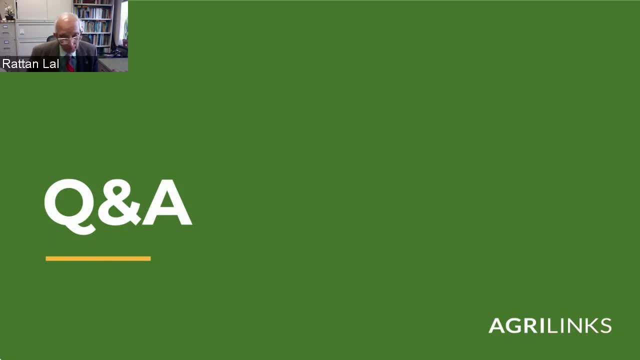 maybe it's acceptable, but 30 percent, 40 percent, absolutely not. So that's where the land will come. Total food wastage is equal to the entire area of South Asia Indian subcontinent, Can you imagine? So we got to think that is where, I think, the children are being educated: the ethics. 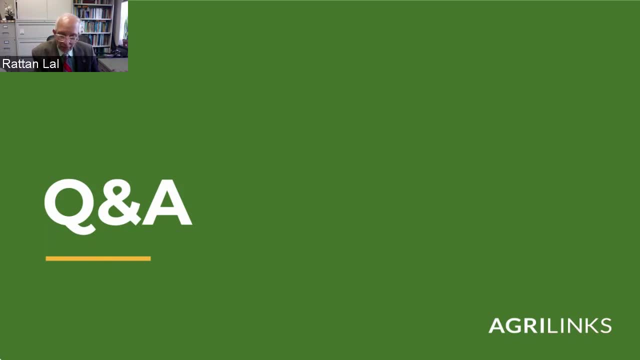 the morality, the value of the natural resources, where the food come from and should be taken is very critical, And then we should reward farmer for using the land properly. So the slogan is: use the best And save the rest for nature. No way to bring more land back for agriculture: return land We. 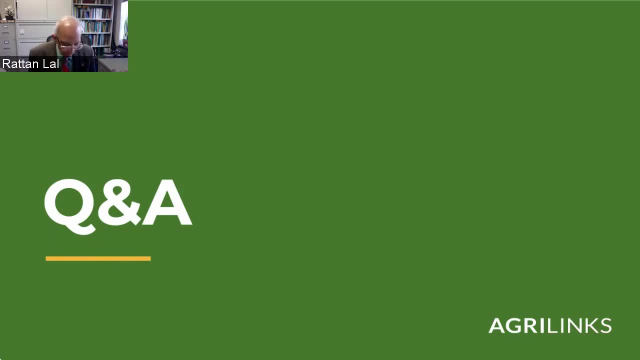 must have an agenda. Ten percent. I think it's too small, Those small farmers who have only two hectares. what I'm going to ask them to return, But a community as a whole. I have seen in Mato Grosso some kind of rule that every farm must have a 30 percent forest- I think something like that on a 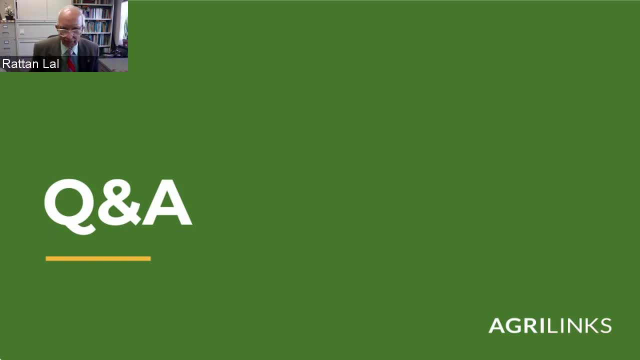 region by region basis, that every farm should have some spare. that's the only option. I want to challenge you a bit on that, Ratan, because I mean, I think you could, like you, say, region by region. the context- specific, But let's take part of the argument- is that we have 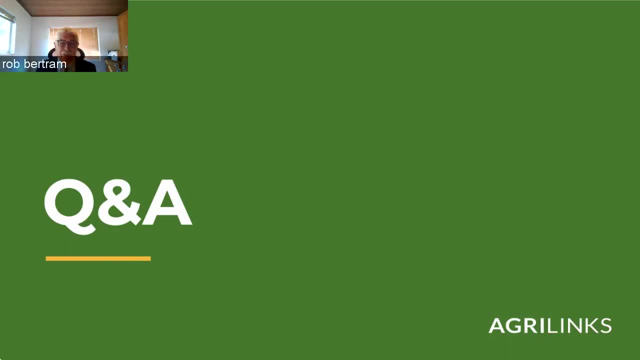 extended agriculture into fragile context, the fragile soils, hillsides, wetlands, that otherwise could be providing all kinds of environment for agriculture, And I think that's the only option. Environmental services, And I'm guessing that for some kinds of environmental services, 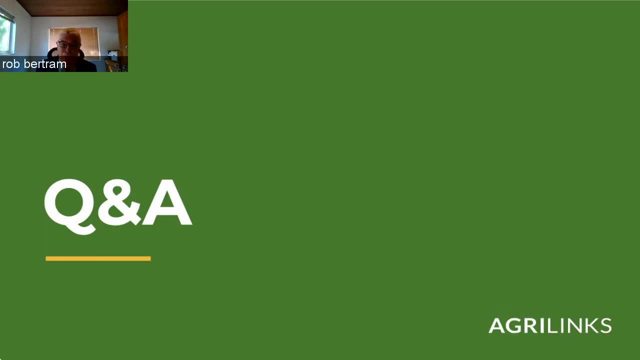 not necessarily say pollination, but say, for example, watersheds and such. you need contiguous areas that are going back to nature. And we're going to get to questions about policy shortly too, But can you say a bit more about this question about where that land should? 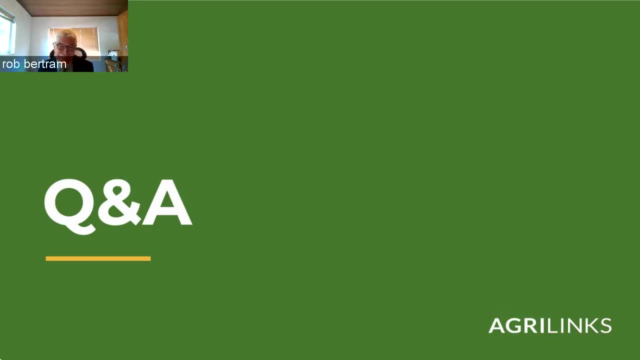 come from, Because I think, like you say, it would really vary. Yes, Rahab, you are absolutely right. You are absolutely right. You are absolutely right. There's no contradiction about that. Agricultural, that's suited for agriculture. So the so-called fragile ecosystem or ecologically sensitive, 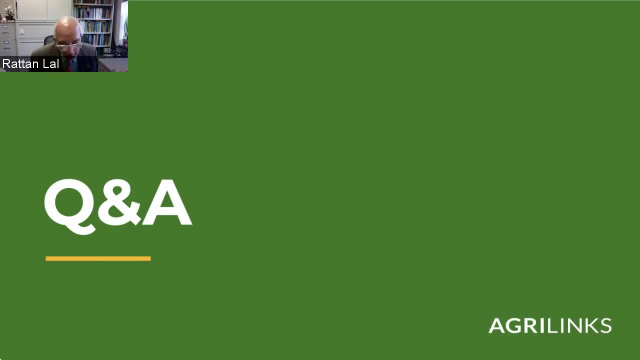 land, Amazon, drier, co-op- steep slope. they really should not be under agriculture. You are very correct. So those priorities, where are the agricultural land which are steep slope, like what we did in the past? We have a lot of land that is not under agriculture. We have a lot. 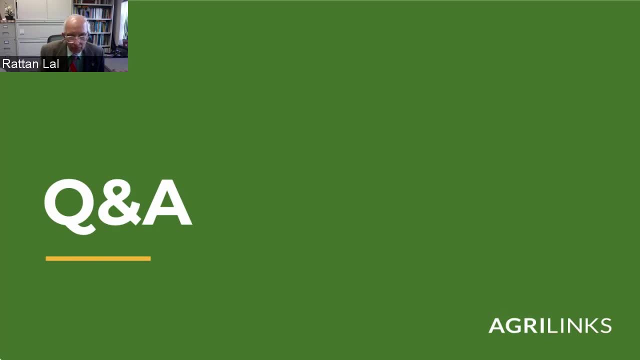 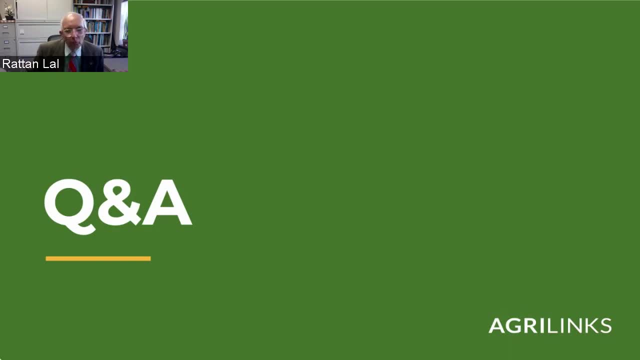 more than a certain slope percent was taken out. They are at. it was. I think the same thing applies globally. The basic concept is that the land which is not suitable for agriculture is the first land to go back to the top. That is where restoration of carbon, water resources and biodiversity 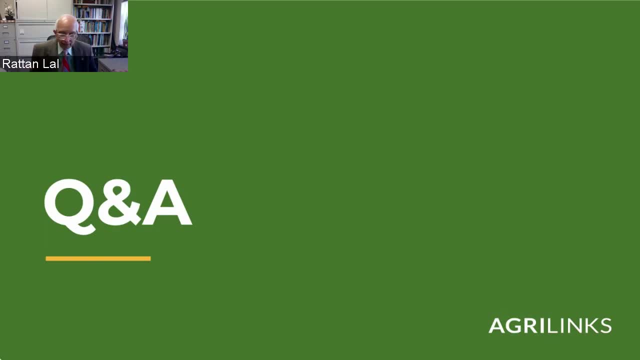 And you're also right, The continuity of wild land from the biodiversity point of view is very critical. it is a complex issue. i think we should all agree that, yes, returning land back to nature is a high priority, but then how we implement, i think all these factors we discussed have to come into play and come up with a policy. 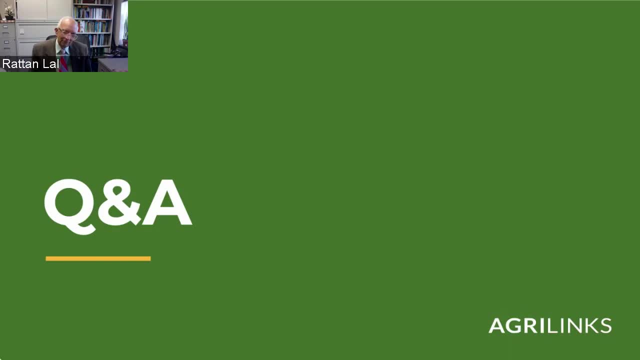 great, thank you. i want to have a scenario question here for you, a fascinating one from perry fowler: a what if? question. what if there had been a cgir center focused not so much on specific crops but on soil? in the absence of this, do we have structures or mechanisms coordinating? 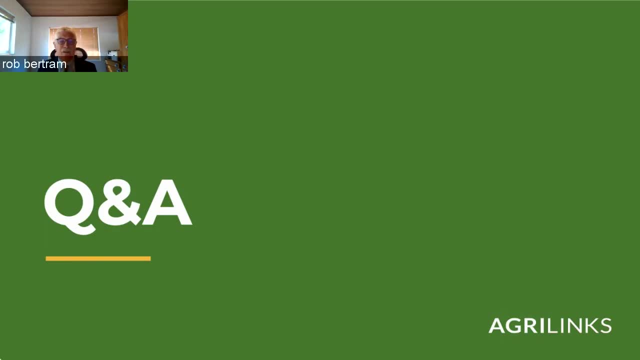 prioritizing and promoting implementation of soil science research. what might you suggest? this is a question that really is very close to my heart. yes, iita in 69, and we thought iita was going to be a soil or natural resource center. uh, the first, some of the first scientists hired. uh uh war. uh, soil scientists. uh, frank moorman, bt kang. 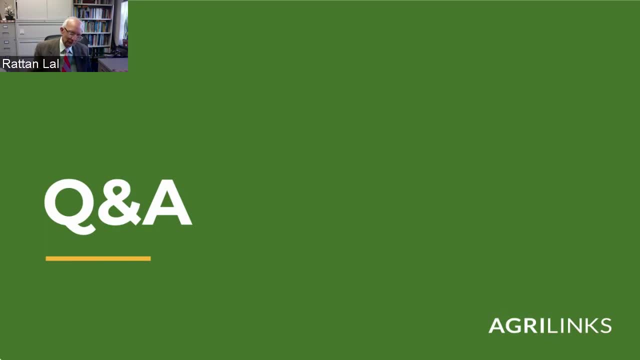 uh, ayanaba myself, tony juo, uh, quite a few. and then later on we learned, uh, that was not the case. uh were also considered to be natural resource based center. and then, you know, in the 60s, uh, these were not cgar, these were kind of funded by. 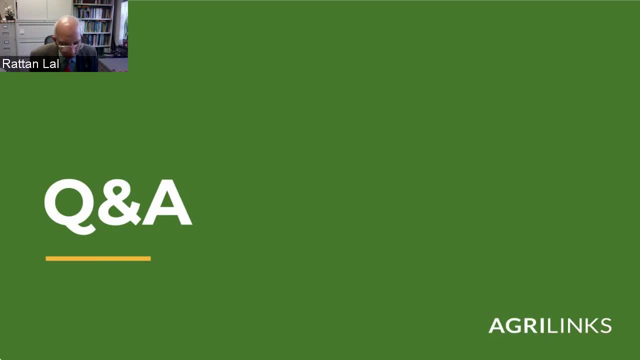 donors like ford and ruffalo foundations of egr came in mid 70. when that came, the mandate again became more commodity oriented and i think part of the problem was we were looking for very rapid impact and unfortunately a variety uh impact can be very rapid, which is a good thing, but uh, that's. 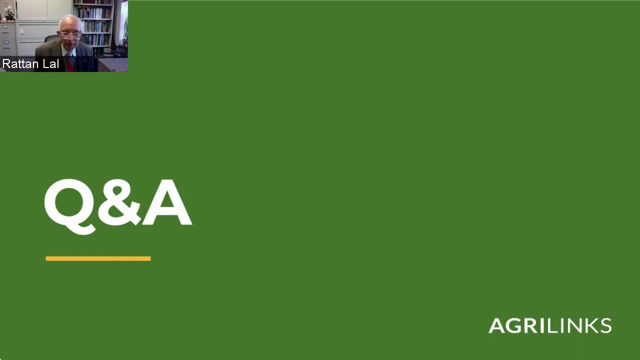 the word. unfortunately, the soil impact may take decades or longer. so over a period of time the role of soil scientists in the cgr system kind of vanished, disappeared in fact. my replacement did not happen very quickly, my experiment was not continued. some good scientists were hired, certainly, but not so. so then they came up the need for this an. 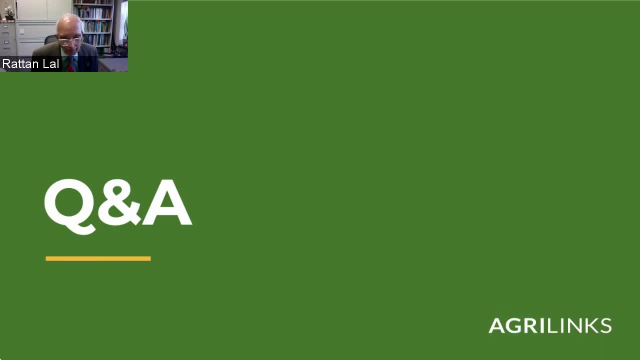 ibsen international board for soil resource management. it was uh, set up in bangkok center and funded primarily through french government. we had a couple of very good scientists: a french scientist, followed by eric craswell from australia. they were dissolved and they joined with me, but you. 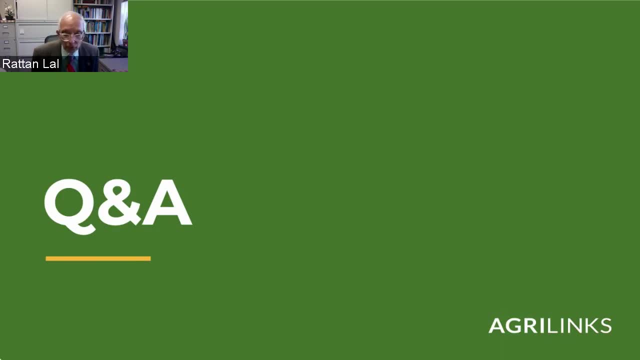 are very right: there is a need for a natural resource soil centric, cgi ar center and whether it will happen. i think now is a good time because now cgr one umbrella and this is a discussion that must happen. uh, icarda has a very important component on natural resource management, so 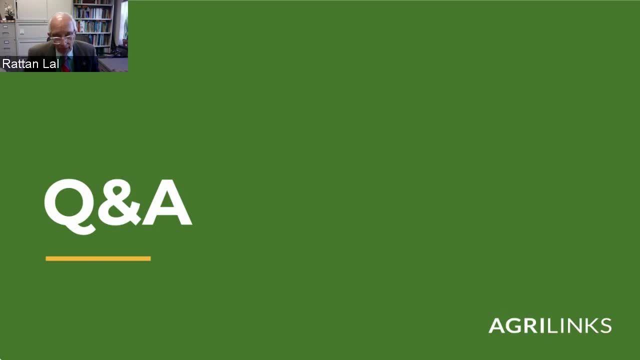 yes, or does uh be at and others? perhaps they could somehow merge together their soil natural resource part. but the need is there, there's no question about it. maybe you know, uh rotan, you made me think back to the first time we met in the mid 80s in iita in ibad in nigeria, where you were working on coming up with. 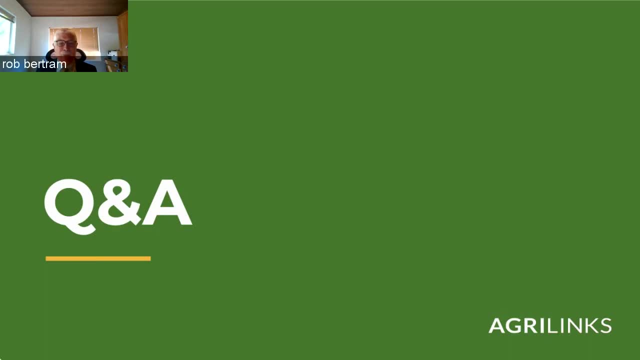 replacements for slash and burn agriculture, which would work with very low populations but is not sustainable and won't support the cgr part of the niger research or the cgr part of the niger research, but it is gonna be the niger research part of the niger research and see which is the best way to. make sure that they can get a good theничarito and ibsen and ibsen and pepsi and and asia were going to work in these work. in these work and ibsen and pepsi will be working with them, but not in ipsi in the 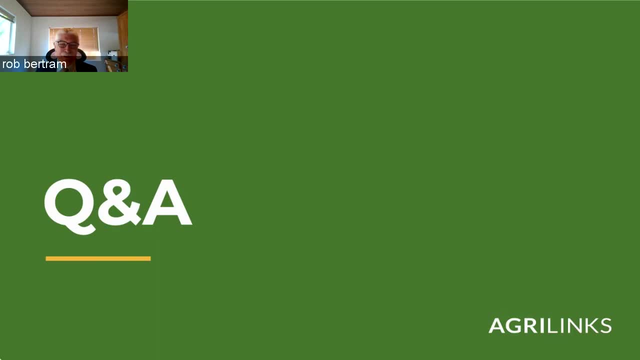 higher levels of population growth, as we've seen in that whole region, and so I remember the work on alley cropping. and these principles are, these challenges are still there, they're inherent, I think, in all the things you were discussing earlier this morning, that right one thing I must mention. 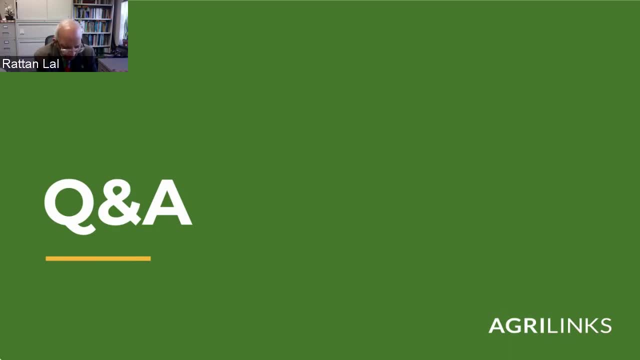 again, I really may have said it: the green revolution in sub-saharan Africa still awaiting happen is because soil, sustainable management of fragile natural resources has not been given the attention that it deserves. and it's not too late, eight years to 2030- to end hunger and poverty climate. 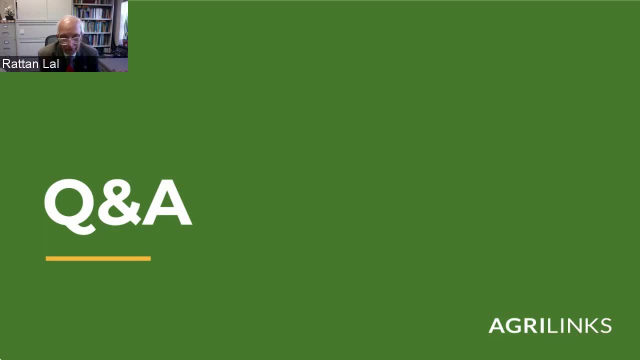 change action. we can still do it, but we got to translate our words into action, so you. so let's turn Rattan towards some of these challenging policy questions here. so let's start with here's one: how do challenges with land? this is from Austin. 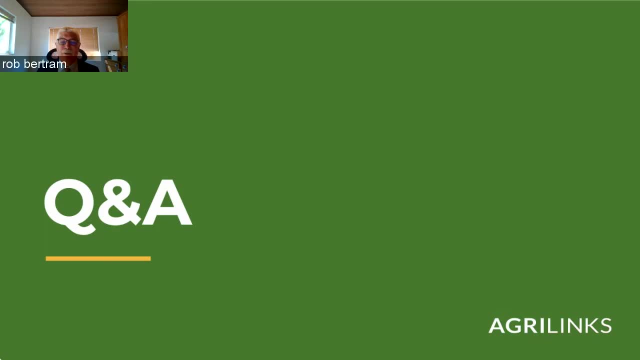 Moore, how do challenges with land tenureship, lack of documentation and elite capture- you talked about land grabs- affect carbon payment schemes? this has been a challenge in operationalizing these approaches in poorer countries. I think this is a very good point. unfortunately, I am not very knowledge about social issues on land tenure, but 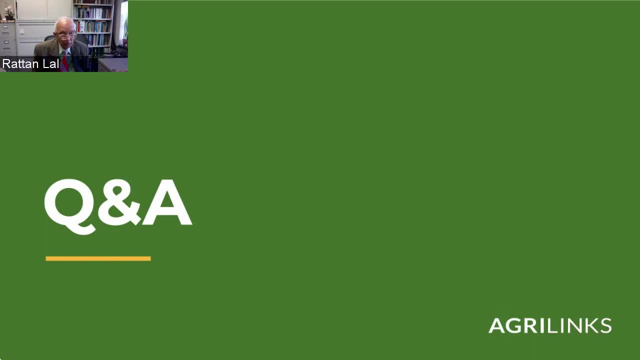 you are absolutely right. land tenure right, especially in Africa, sub-saharan Africa, are not pro farmer. the farmer who is cultivating the land may not own the land in most cases, and especially the women farmers, which are sixty to seventy percent of those small holder. I came across as something which I will never. 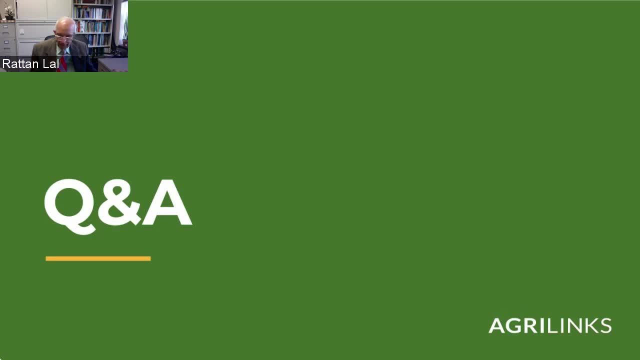 forget I was visiting cement and the colleague there took me to see some farm and on the way I saw a farmer packing the crop residue, putting on a donkey cart- obviously take it away to market- and I stopped a picture and asked: why don't you leave this crop residue back? and the farmer 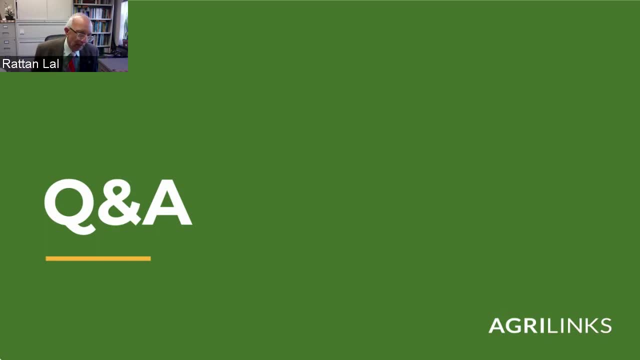 who try interpreter said: why should I? so I gave him all these common. you know your crop next year will be very good. you save water, you save nutrient, you will save your productivity very good. and he answered back: this land will not be mine next year and I don't need as bad what they're going to happen next. 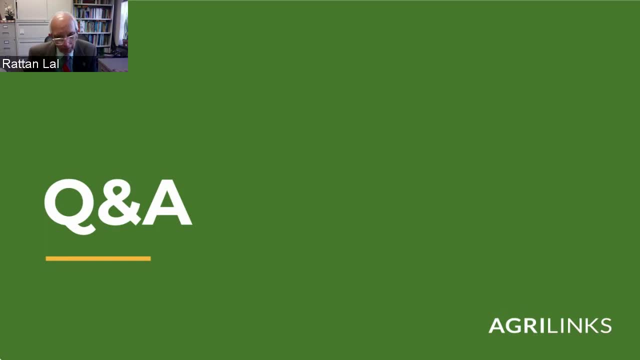 year. I need the money tomorrow morning to buy shoes for my child. here is the story of tenure. if a farmer does not own that land, he or she has no reason to invest long-term basis on that. so government, local organization, they must make sure that the property rights are secure so that the long-term ownership, long plea, killer of. 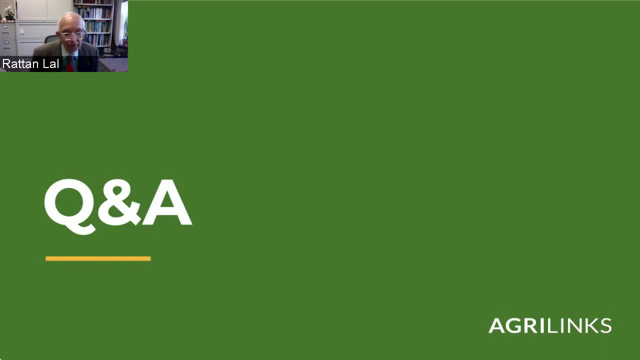 the land so that the that killer of the land is rewarded on a long-term basis. that's a very important issue and I think the policy makers should really pay attention to it. great, thank you. and that's Tata asks. he's firstly thank you for your presentation. he says it is obvious from your presentation that the need to 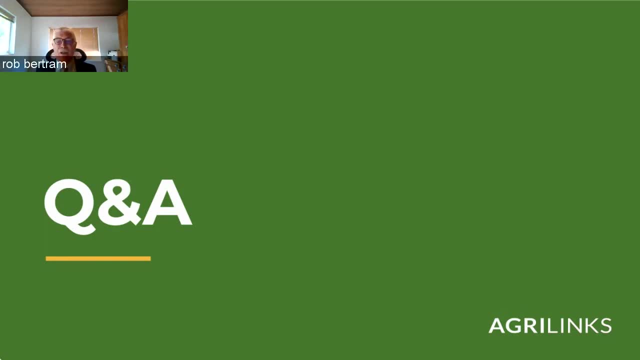 restore soil. health cannot be overemphasized. in your presentation you recommended some technical solutions: regenerative agriculture, conservation agriculture, etc. do you also see the need for sustainable, new sustainable policies to drive the change? and, if I might, I just wanted to make one comment about the tenure. seems to me rattan. if we're going to, I'm going. 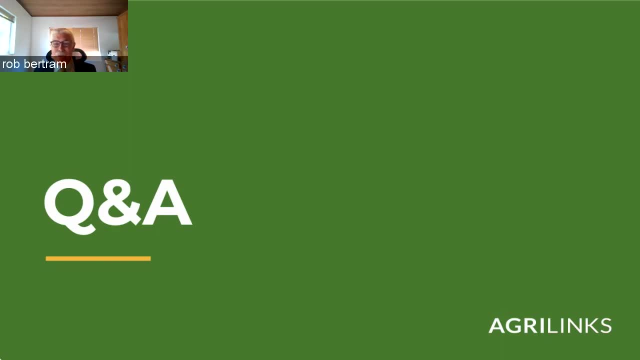 to say this first: sorry, if we're going to shift towards a system of payments, this issue of tenure and ownership is going to become more critical than ever. for all reasons, the question are flagged. so but but let's. let's go on now to this question of policy. what are your thoughts about how policy can play a? 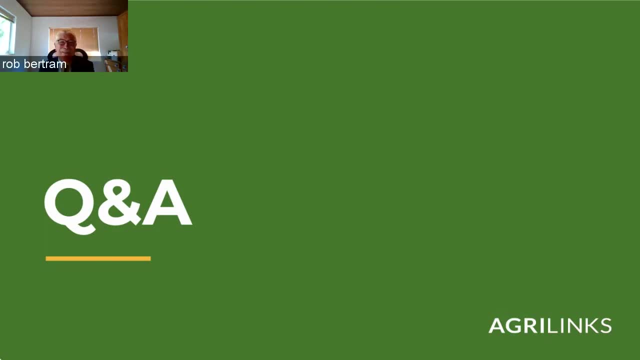 role, which also takes us from that to policy as well, Rob of. the important question really is how to translate known science into action. you know whether it's a conservation agriculture was agroforestry, alley cropping, whatever you have. how do you try? there are four ways we could possibly think of. one is 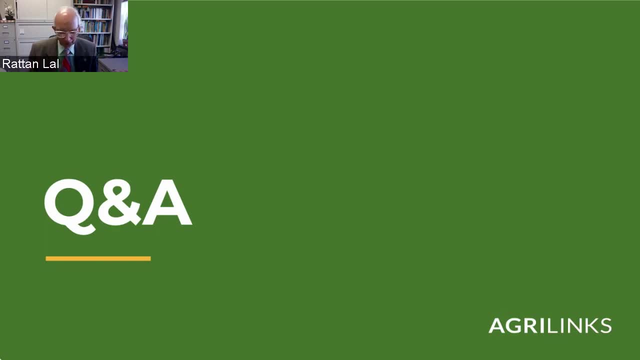 go back to the original spiritual, religious beliefs, whether people are believing in Islam or Christianity or Islam or whatever you want to call it. so, whether you want to call it Christianity or Judaism or Hinduism, all scriptures- Christianity or Judaism or Hinduism, all scriptures really say protect, restore. 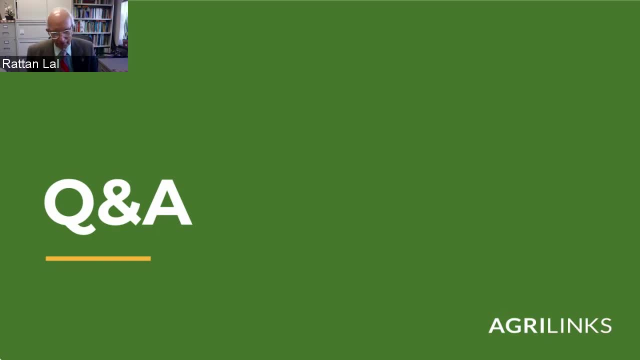 manage Mother Earth properly. in fact I have a table showing what Judaism talks about it, what Hinduism, Buddhism, Sikhism, Islam. but they so go back to our spiritual leaders, and Pope Francis does a great job. in his encyclical he really emphasized the importance of protection of land resources. that's one. 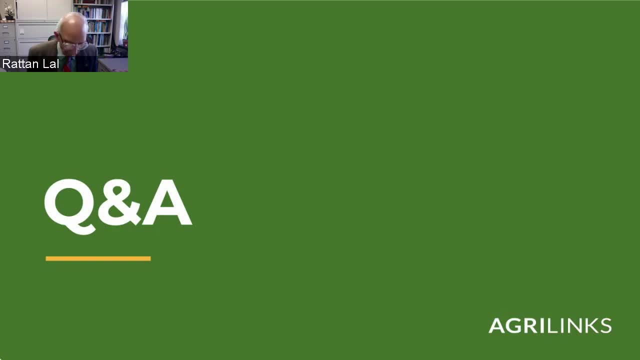 the second part is giving financial importance. the third part is education, and I talk about education right from the children. the fourth part is policy. it's a very important part. the policymakers have to really translate into action, and I have been talking about the us. in the us, we have a 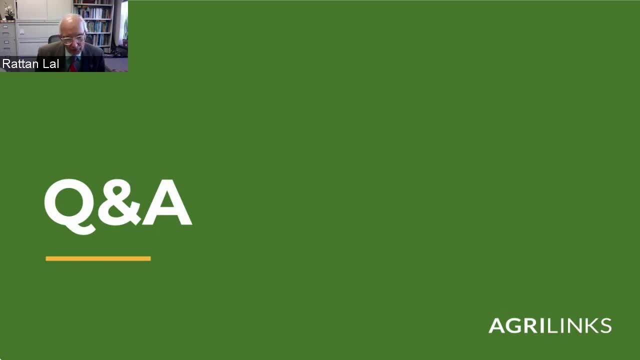 Clean Air Act. we have clean water act. I question whether you can have clean air and clean water without a healthy soil act. I really hope that the farm bear 2023 or 2024, Rob, will have a healthy soil act. I want to make sure it. 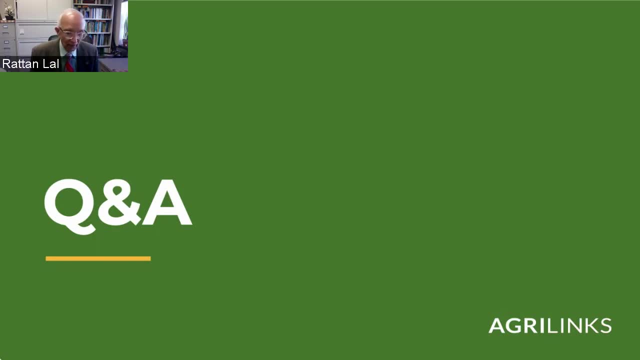 does not mean people who do not protect soil are going to be punished. no, it means those who protect soil will be rewarded. I think that's the way to go for it. we have, on a global, a few had a soil protection resolution going back to 70s and 80s, but it has no implementation. 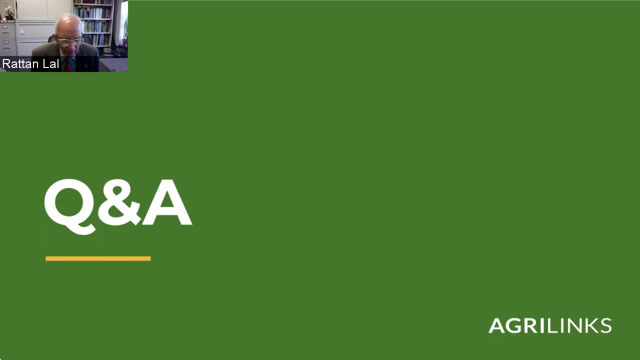 part. in 2008- I was at that time, 2007, president of Source inside America- I did submit a soil protection resolution. US Senate passed it unanimously. it is a resolution 440. the 440 resolution was never translated by EPA into soil health act. there's a need for it and if us adopted, I'm sure Europe and rest. 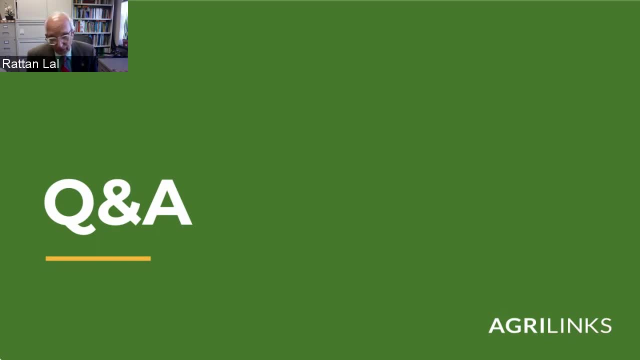 of the world will follow suit, and this is something very close to the concept you are talking about, fortunately. again, going back to the US Senate, last year- 2020, I think- we had a growing climate resolution act. it was approved by US Senate, but it again need to be translated into action. 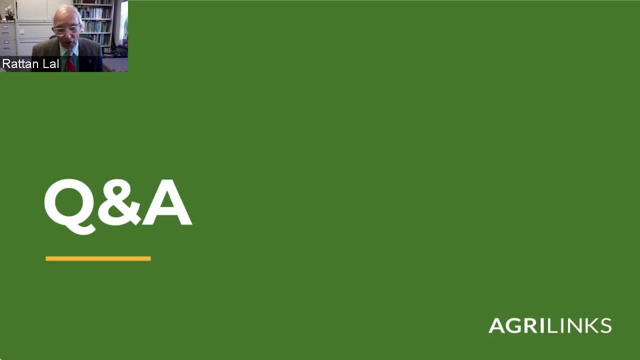 and that action translation means policy where farmers are rewarded. I think the farm bill coming up must really look into very closely and on a global scale that should that should really follow so soil health act and payment to farmer through farm bill as an example of what can be done globally. thank you, thank you. 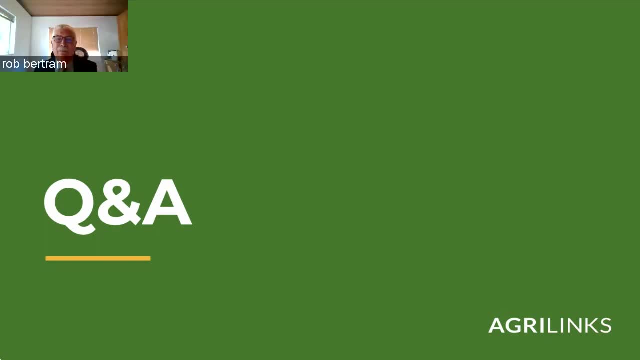 Rattan that the, I have to say, the number of questions that are coming in about this whole issue of soil carbon financing it. here's another one from Bram Peters. I mean well, I was gonna say is I think we we may need another session deeper dive on this. but brown Peter says very: 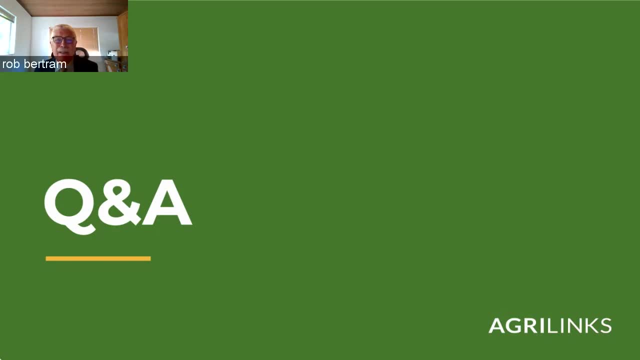 insightful. what tensions do you see between land grabbing and soil carbon farming schemes now currently being proposed as part of climate action? again, this question of money ownership tenure, etc. well, you know land grab the issue, and I mentioned when the per capita land required is point two, five quarter of a. 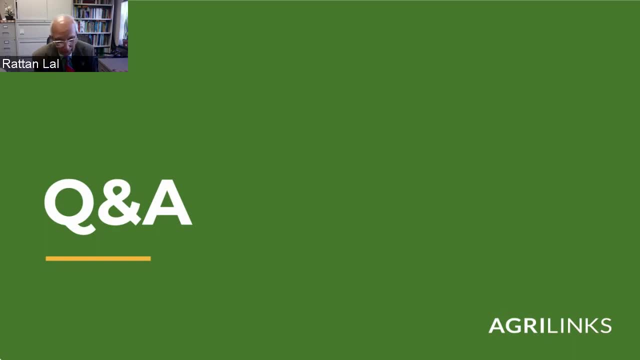 hectare and the country has only point zero five or point zero six. this is going to happen. so somewhere along the line we have to make sure as a universal law- national as well as international community- hopefully United Nation can take more active part in it- is to make sure that the land within a country is. 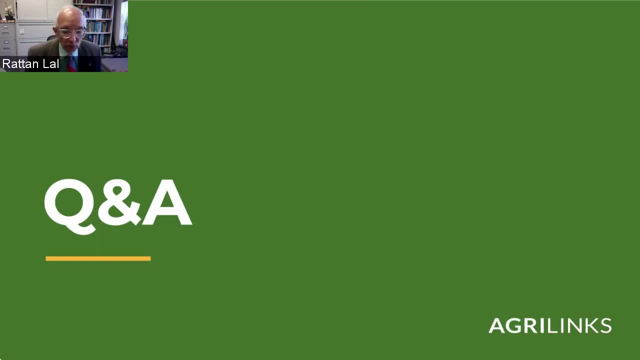 used properly, justly and with science-based methodology, science-based, proven science technology to bridge the yield gap which exists very, very hugely in developing part of the world. I mentioned in India, I mentioned example of Africa, same thing in Central America, same thing in the Caribbean, that is. 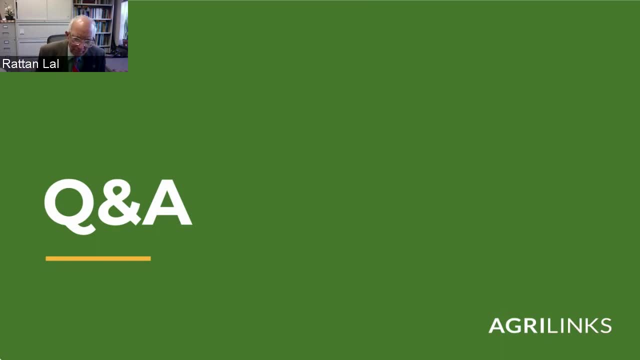 where the refugees come from, by the way, and that's what I call soil refugees- in numbers of varies on who is estimating and what is considered as a refugee, but it's a 75- 80 million people which are so-called internally displaced, and land grab is a symptom of that. that problem that we have to address, that's the problem that we have to address. 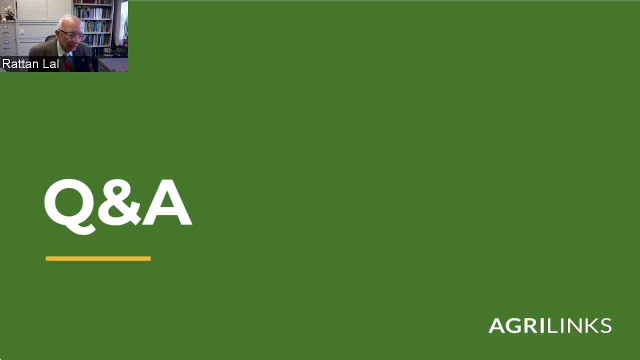 So somewhere it goes back to that. this soil must be managed in such a way that it can support the people living on it, and my favourite concept, which I have been talking about, is land and people are intricately interconnected. They, in fact, are a mirror image of the land they live on and you don't have to go. 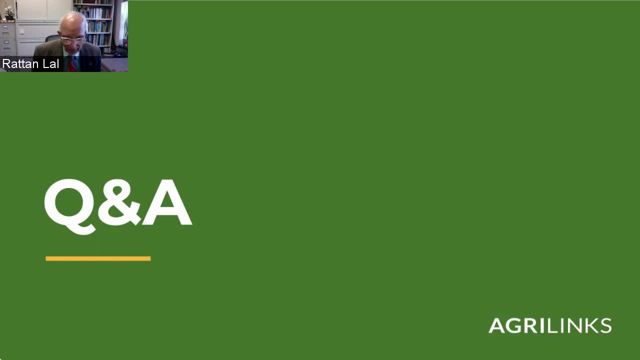 far to see that interconnection, drive through Midwest and drives to sub-Saharan Africa, South Asia, the Caribbean. You will see that. So when people are miserable and suffering and poverty-stricken, they pass their misery to the land and land reciprocates. 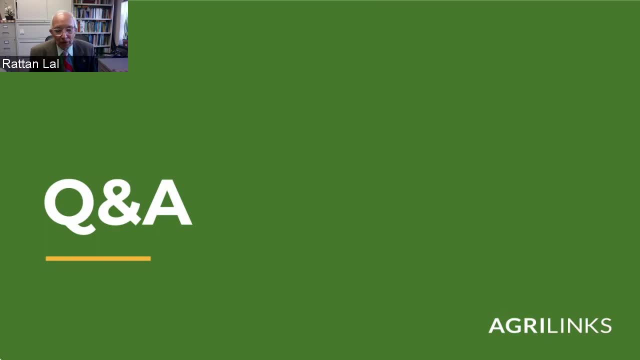 and that causes refugees. It's a spiral. The solution lies in restoring soil health on a long-term basis. I want to also pick up Ratan on a question from Carl Wall, who says: you know, how do we move from this systematic? 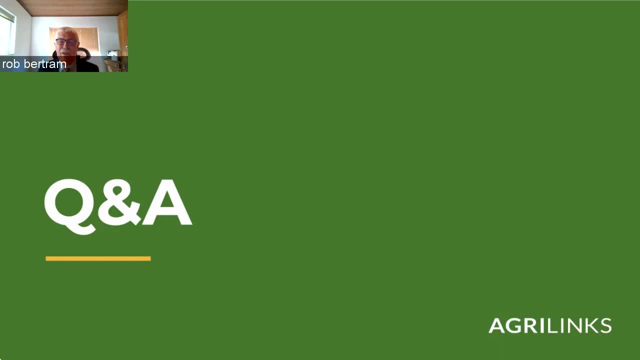 formulaic form of agriculture- improved seeds and fertilizer- voted under the green revolution to one that requires far more nuance according to specific soil and rainfall context. What are the implications for extension? And I guess that was the key thing I wanted to put in front of you. 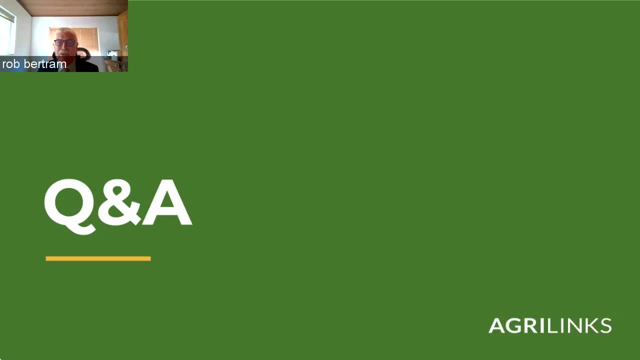 from this question. How do you see extension coming into this? What is the overall effort that's needed? Extension has a very, very important role to play. You know the problem that the technology has not been adopted in those countries where there's a big yield gap, because the support services 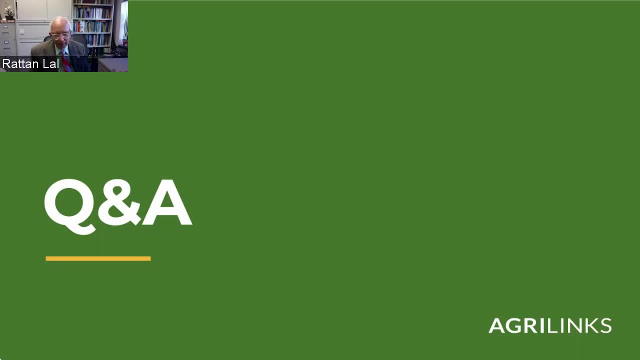 of extension especially, are very weak, very weak indeed. So organization extension service, which means really helping farmer. what are the modern technology and land grant system has worked very successfully in the US because here we had a combination of research, teaching and education. 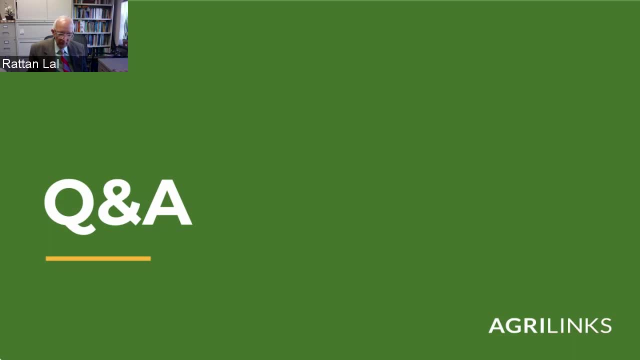 And some of the successful universities in South Asia adopted that system. I think that system is still not very well adopted in elsewhere, such as in sub-Saharan Africa. Extension is under one guarantee, under one government, education is under research is another government and i think that separate. 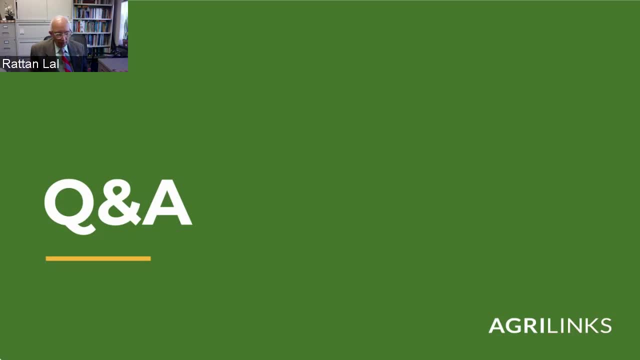 entities have created also a problem. so one is the quality of extension uh, the magnitude, strength, ability of the extension service to provide. the other the mechanism, how they get education and research information to integration. uh, extension obviously is a very, very critical part and it is even going to become more important, even in the us now and other elsewhere. 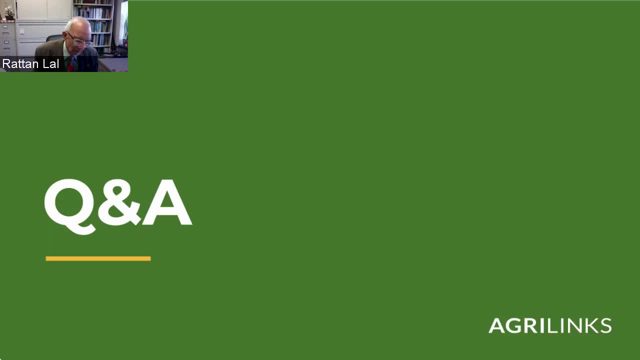 you know the moral act and you know more about it than i do. at that time, 1980, when the population of us came from rural to urban- 50- 50. right now it's 80- 20.. is the land ground system now really effective in extension, not only for agriculture but also for? 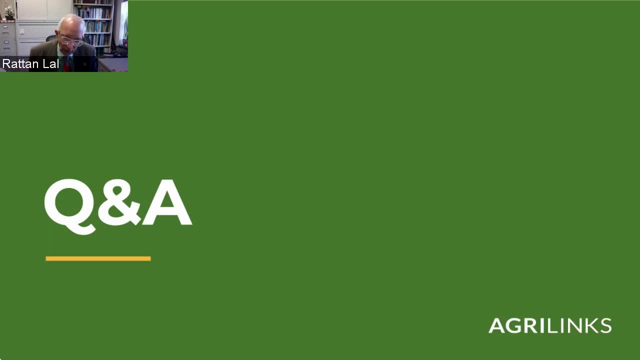 urban systems and health systems and other. so extension role is dynamic. yes, it has to keep so. rattan, i'm going to jump in because i know we're just need to wrap up here, but i want john baker, our chief nutritionist here at usaid, said: thanks you. and he says it's a privilege to listen. 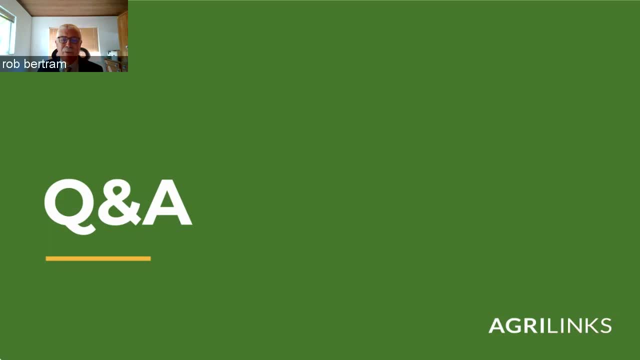 to your wisdom for the food system summit, the un summit from last year. what, for you, were the biggest wins? what were the biggest missed opportunities? well, the biggest win for me was that i was invited to be a member of the science committee and member of action track three, and i learned many things by listening to. 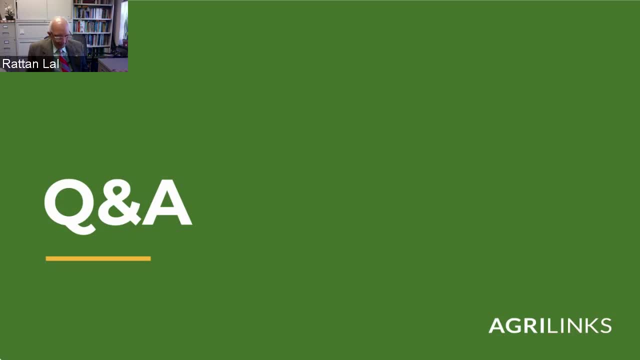 others. so it was really a personally a great um player to be part of that whole system, but i failed. i really failed. for example, i talked about nutrition, sensitive agriculture. i talked about one health concept: health of soil, plants, animal, people, ecosystem is interconnected. the one health concept that came out in the final was not the same. i talked 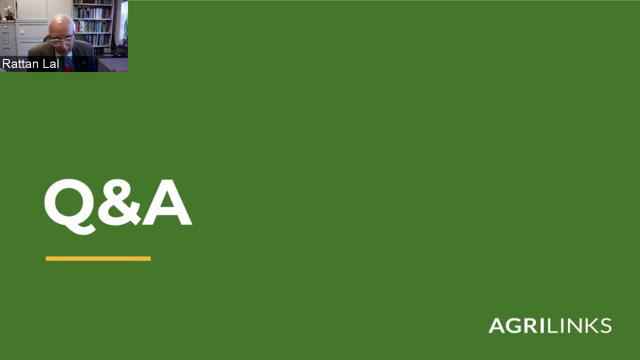 about the word soil health restoration as the basic component of sustainable development goal achievement. the four-letter word soil was not in the secretary general report, so that is what i said. i feared so, but failure is when you give up, and we should never give up. uh, cop 26 was also failure from that point of view. the word agriculture and solver not in. 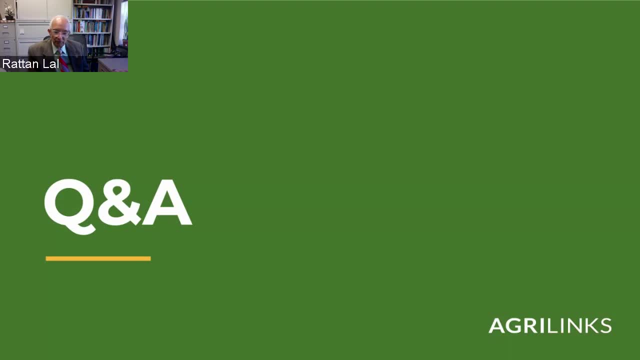 their final report. should that happen in cop 27? no, it should not. we are not talking about isolation, that varieties are important and irrigation is important. further, we are talking about soil health integrated system. how can you ignore it? so i think that was a disappointment, but this appointment does not mean that. uh, the cash i mentioned, uh, something that 110 countries. 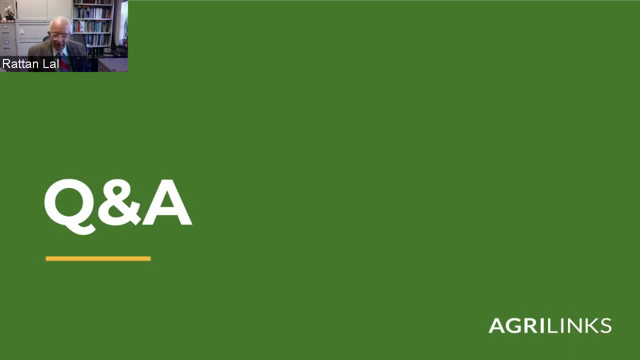 are already. we are not giving up. they are continuing it. one day the top people will hear. so, rattan, i want to try to give you the last word here this morning. i just can't thank you enough for and we have so many questions we couldn't get to. i apologize. 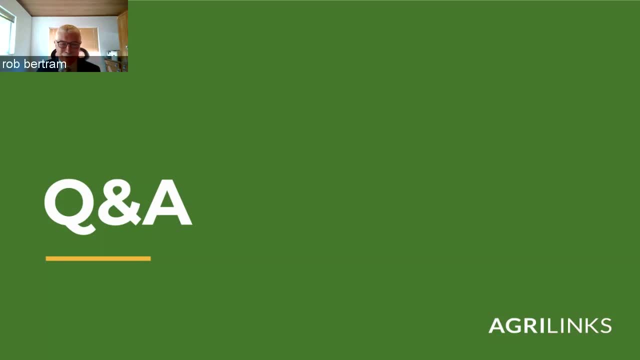 to those who wrote them. I tried to pick ones that I thought were representative. But, Ratan, I guess I'd love for you to talk a little bit about in your last comments: about agriculture and food, the environment and biodiversity and climate change and what needs to happen that isn't happening now. 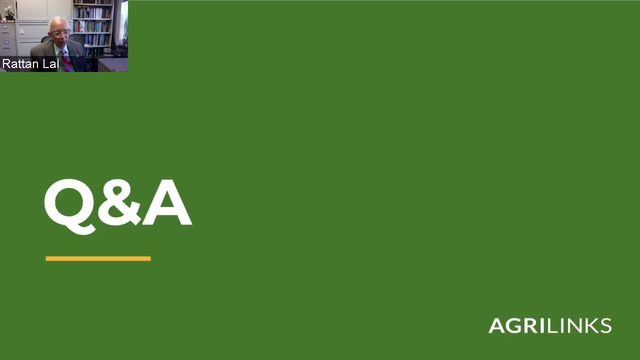 I think giving a respect to agriculture profession, The farmer, comes number one on that, Making sure they know that the public, the humanity, respect them for doing great things such as giving them healthy, safe and nutritious food. One part: healthy environment. Farmer are the greatest steward of the environment.